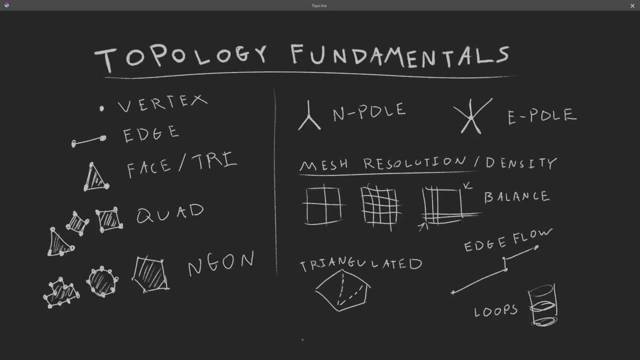 hand is going to be a vertex, with five edges or more, up to an infinite amount, coming out of a single vertex, right? So mesh resolution, density, kind of the same thing You can think of like a grid. That's low resolution, low density. Subdivide it multiple times, you'll end up with a higher. 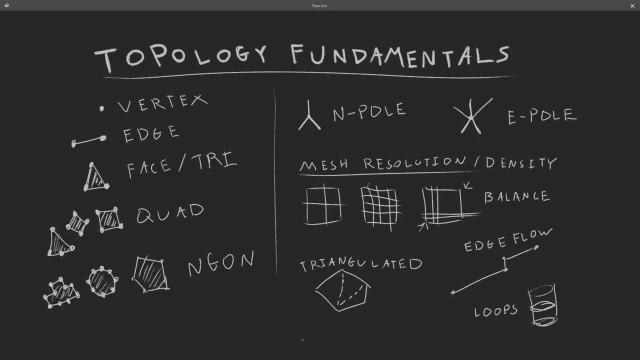 density mesh. Your model itself can have fluctuating densities throughout the model. It's better if you try to balance these things, but it's not always going to be possible. in some situations, You actually don't want to do that. when it comes to like optimizing models for games and things like, 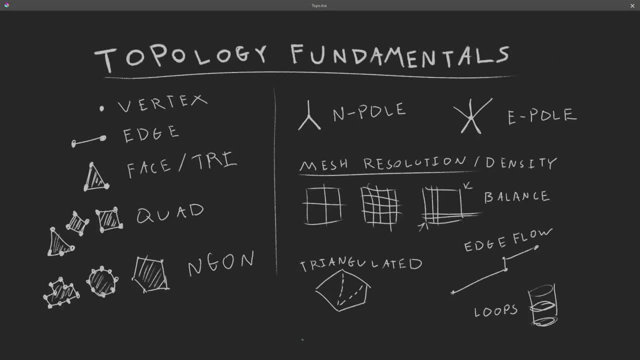 that. So all mesh at the end of the day, or all faces at the end of the day, except for a triangle, will be triangulated underneath everything. You won't see the lines drawn. So if you have a face, an ingot or a quad and you pull up one corner, you will actually see the 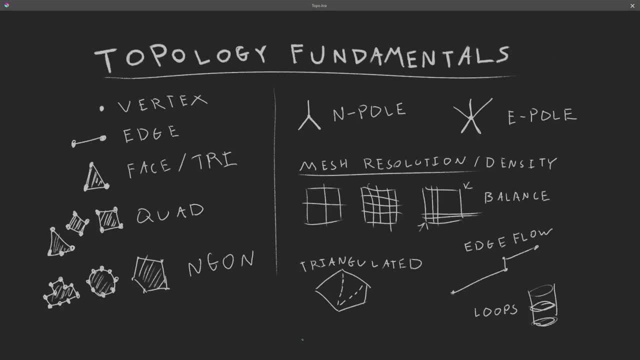 triangulation take effect on that face. We're going to talk about that one more as well. Now, when you have edges, usually they naturally kind of have a flow to them, And if you take that edge flow and you wrap it around your model, it'll end up creating a loop. 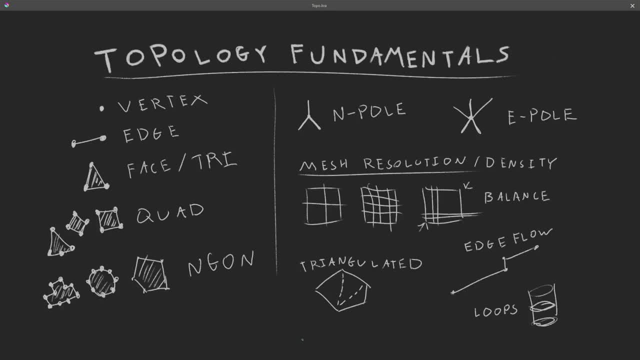 basically. So edges, edge flows are like the best way you can control your mesh, generally speaking, when you're working with 3D models. So we're going to play around with all of this, but we've got to go to Blender to do it. So this scene here, all we're going to be doing. 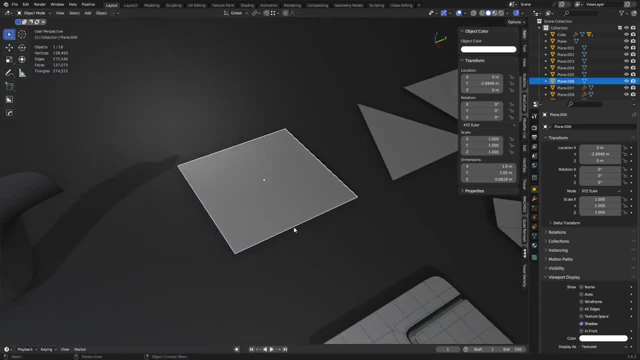 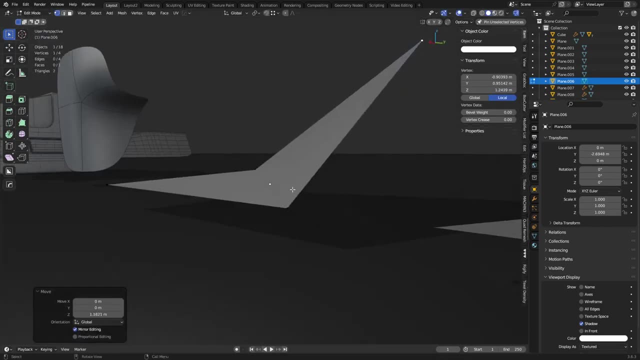 is kind of breaking down a few things, some of the stuff I just talked about. Let's start with the plane first. If we lift up a corner, you'll see it actually is triangulated And that's why we get this little crease here, And so if it's flat it's called a planter face. If it's not, 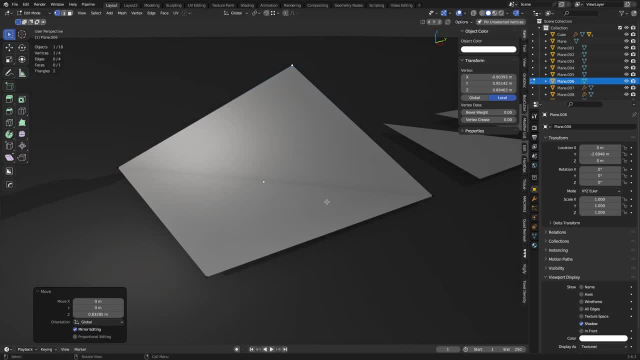 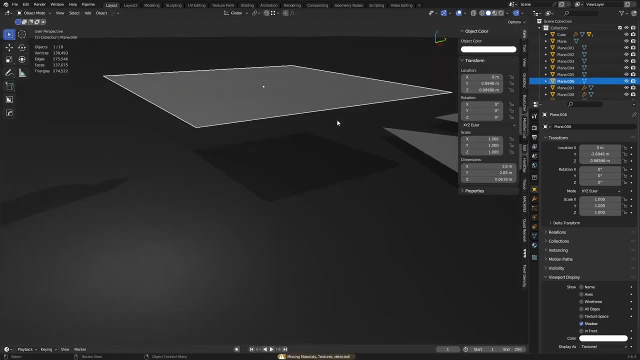 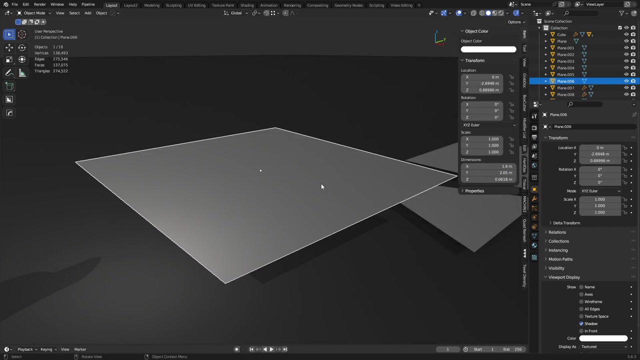 flat where you do something like that, that is going to be called a non-planter face. Now let's go ahead and lift this one up a little bit real quick, And what we'll see here is that by default in Blender, all faces are rendered double-sided. 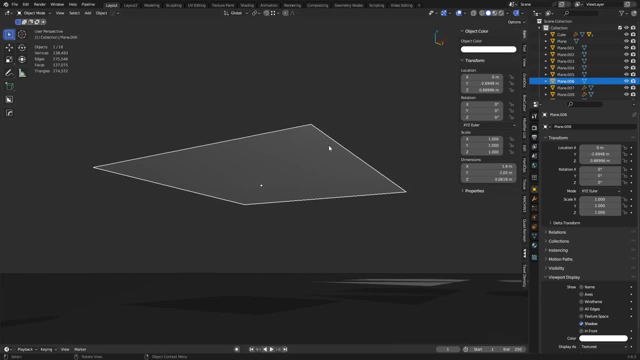 So it'll have what looks like another face under here, right Or a backside to it. anyways, That's not how usually game engines display things. So if you turn on backface culling, you'll see it actually becomes transparent. I only recommend getting used to this idea because 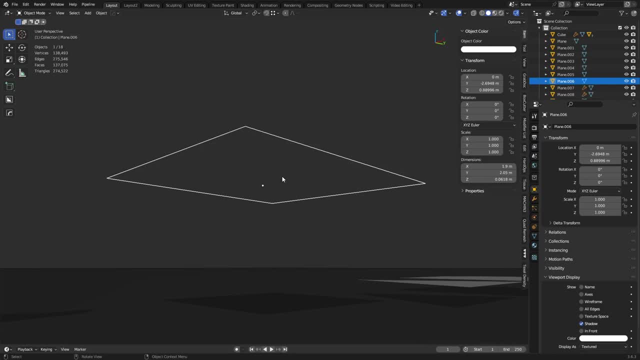 if you ever run into this problem in a game engine, you'll be able to recognize this a little easier than if you were using a backface culling. So if you're using a backface culling, you'll be able to recognize this a little easier than if you were using a backface culling. 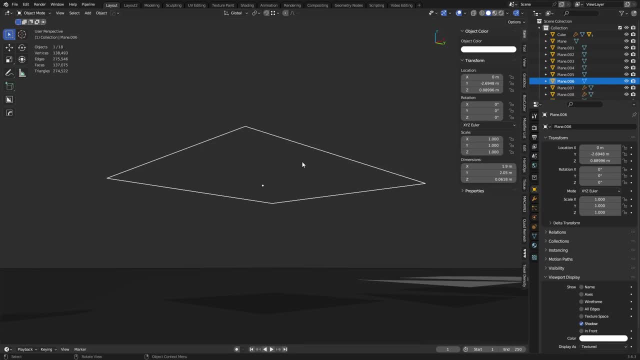 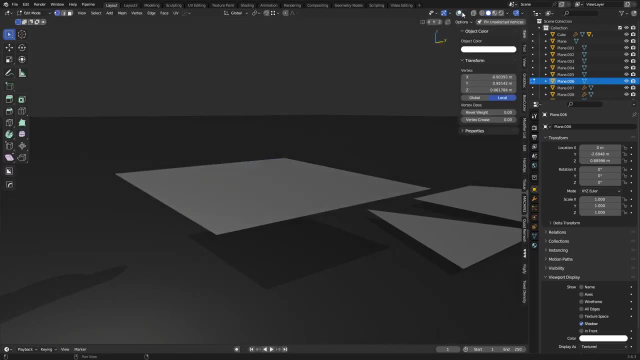 Other ways of checking if a face is forward or backwards, But you can check it in other ways. So if you turn that off and you are in edit mode, you'll see here that in this dropdown there's something called face orientation. Okay, And so you can see what it's doing. It's drawing. 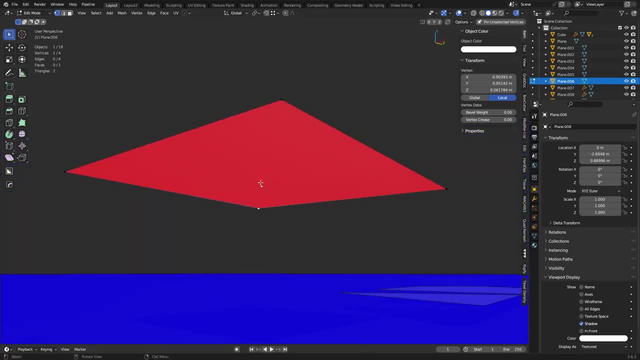 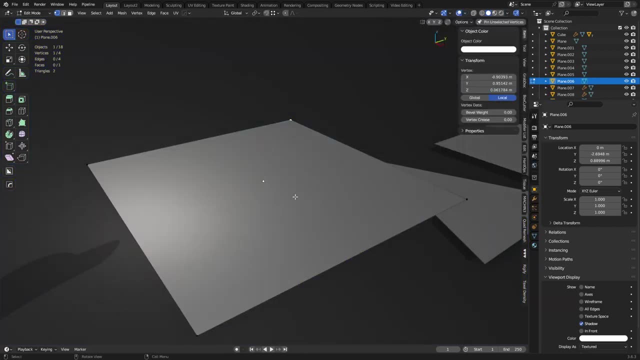 faces that are forward blue, but if they're backwards they're red. Okay, So you can also do that if you wanted to. That's going to be up to you. I prefer just going with backface culling Now here in Blender, if you're working with a backface culling, you can also do that with a. 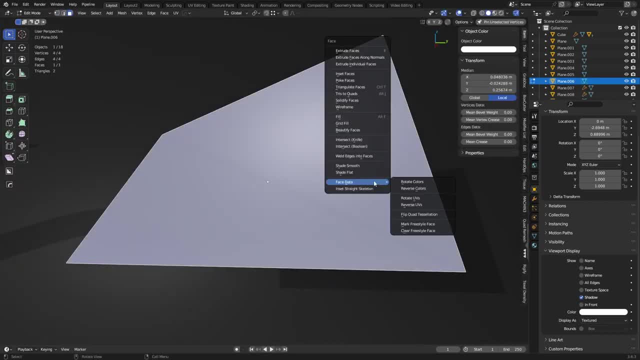 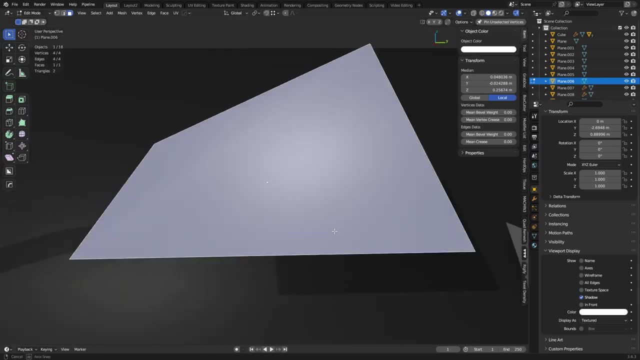 quad. You can actually switch that triangulation by hit control F doing face data, selecting face. control F, face data. flip quad tessellation. You can actually set it up something like this if you wanted to. A little hard to see it, but basically the edge is now running down this way, So that's. 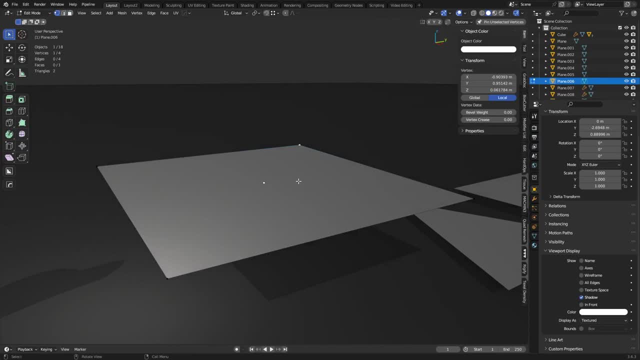 something to keep in mind as well. And of course, faces do have what's called a normal. You're in edit mode. You can turn on the face normal here and make it bigger if needed, And so it does have a direction to it. So when you hit all in and you flip it, that's going to reverse. 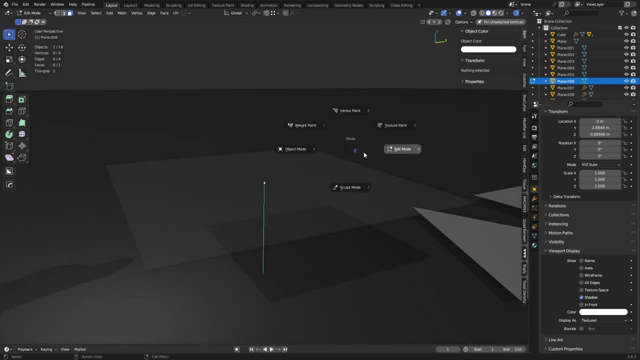 It basically right. So that's what's going on there. Now you don't just have normals on faces, You have normals on vertices as well. I'll flip that back. So when you're working on a mesh and you extrude another piece out here, it always has this normal data for every face. So here's the. 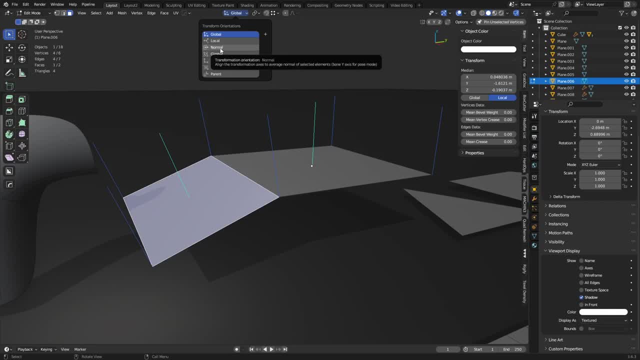 trick about this. You can actually use this to control your transform, So you can use normal up here. So if you're using like the move tool, you'll see it actually goes up and down on that normal. So normally when you do like an extrude it goes out on that left side So you can actually 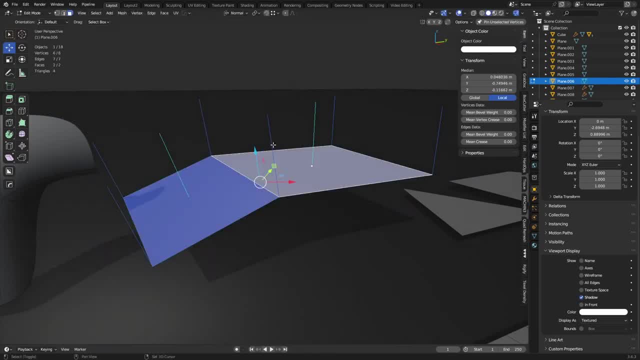 do a little blue line. That's what it's actually doing. It's following the normal there. So when you select two faces and you extrude, it goes on the combined normal between the two. If you ever don't want that behavior, you can switch to an active element. You can shift, double click on. 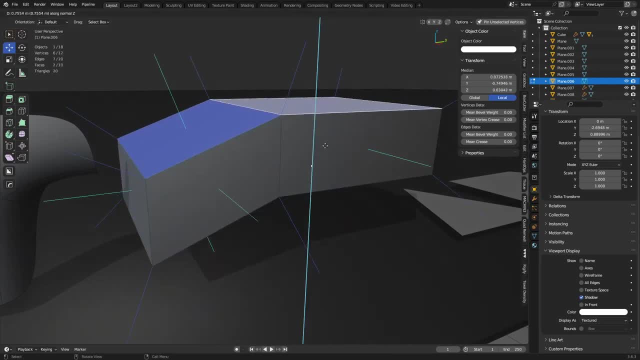 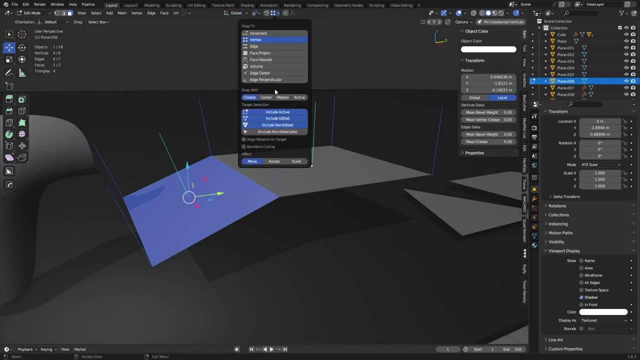 something and you'll use that one instead, even if you have both of them selected. Okay, So it's just a good piece of transform information there that might help you out when you're modeling. All right, Let me delete that. Let's turn off the. 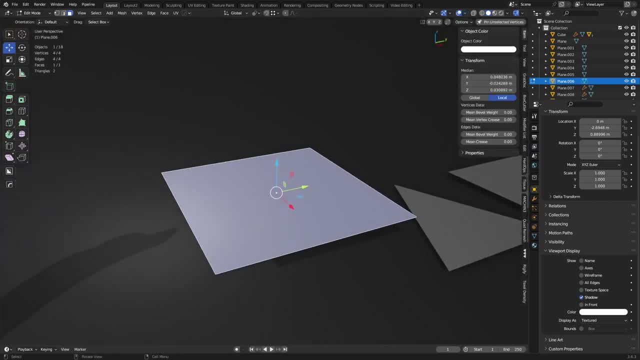 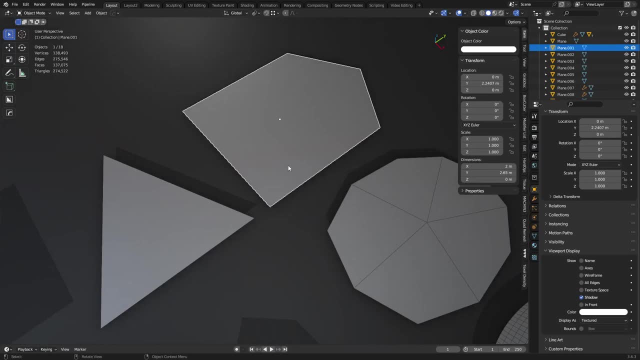 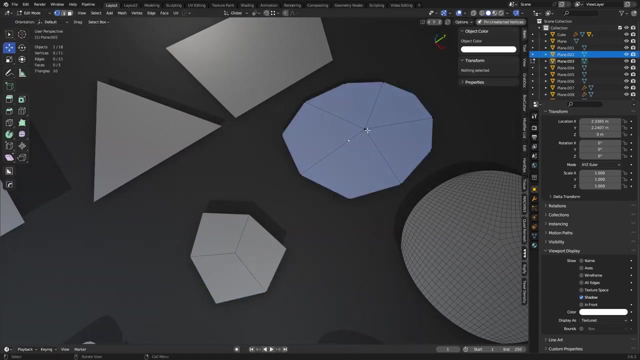 normals, All right. So let's go ahead and check out the end pole and the E pole real quick. So if you had a triangle or a five-sided end gun and you subdivide these one times, they're going to actually create the end pole here, I'm going to create the E pole here and these are surrounded. 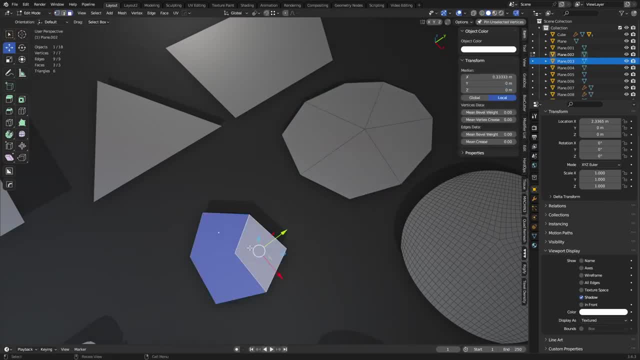 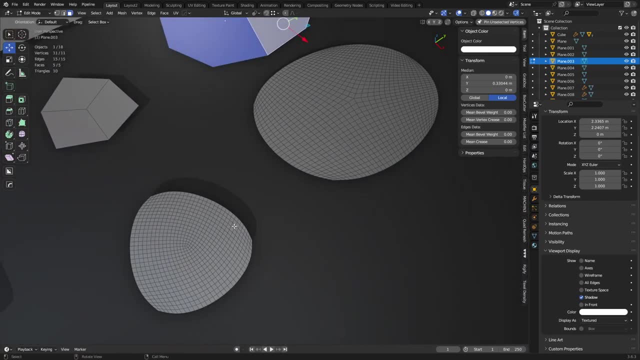 by quads, So just pay attention to that as well. It's three quads here and there's going to be five on this particular shape right Now. when you subdivide them more, the end pole is going to start to create the end pole. So if you had a triangle or a five-sided end gun and you subdivide, 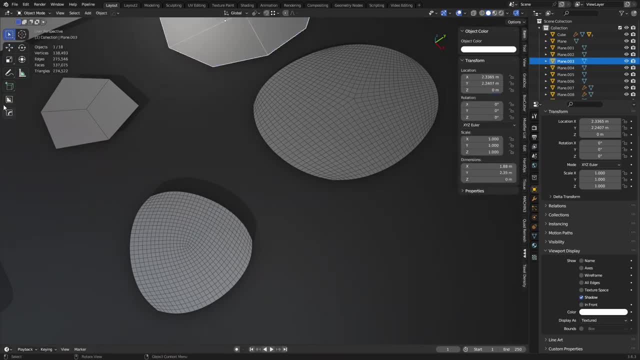 them more. you're going to see the end pole will start to create the end pole. right, This is going to create the end pole here in the end pole, So that's going to be kind of a pinching effect here. Okay, As you subdivide it up, this is just something worth noting that it's going to get. 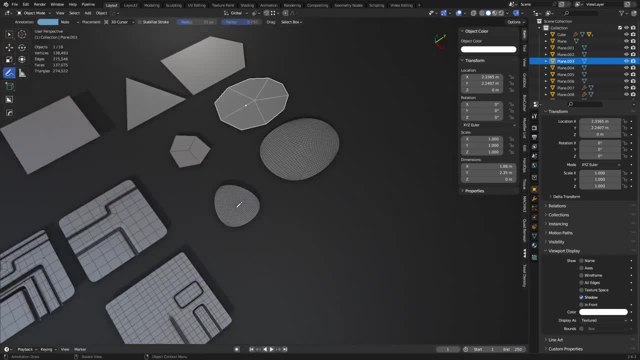 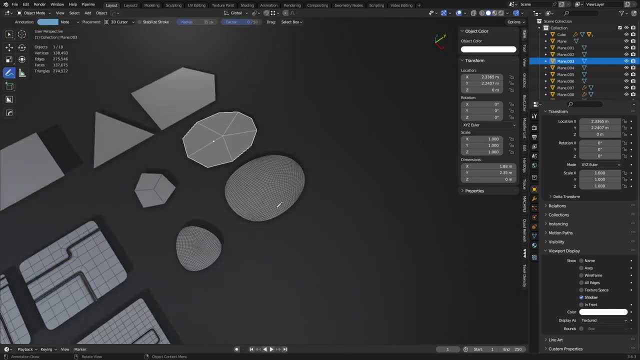 denser in that little area right where the pole exists. So if we zoom out you can see what's actually going on there. So the mesh density rises a little bit in those areas and on the E pole it's going to stretch apart a little bit So it actually isn't as dense in that area A lot. 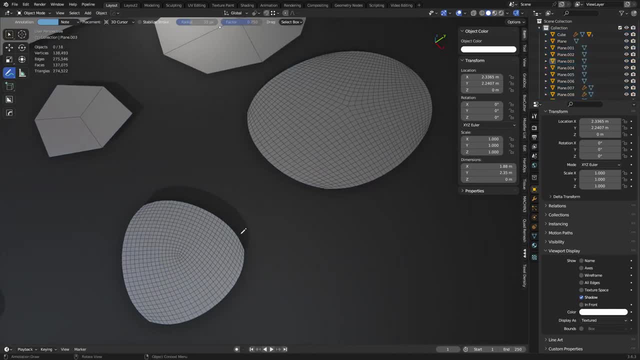 of times the poles are used for redirects of your topologies, So you can actually see how the topology is flowing here. these edges, the edge flow, the end pole is doing something like that, whereas the e-pole is a little bit more interesting because 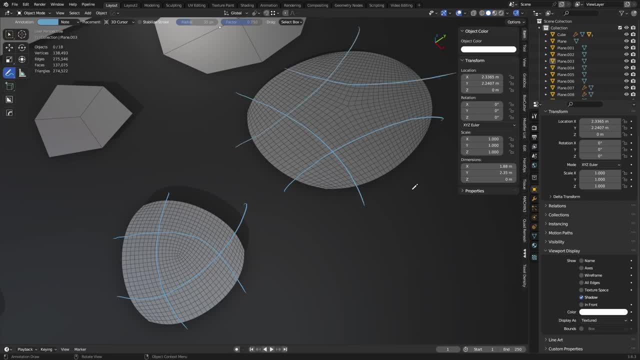 what this one does is it sends edge flows out in all kinds of different directions. so it's actually really useful when you're trying to run different edge flows into each other but you want to just kind of redirect them back out in different ways. now, truthfully, you're more than likely not going. 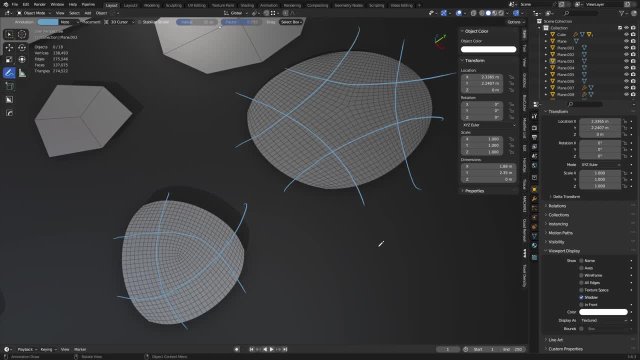 to intentionally try to create e-poles. it's just usually not how it goes. however, the um, the end pole you will want to utilize in a lot of situations and pay particular attention to it. you will be creating that one for sure, because it's more useful for redirects in most cases than 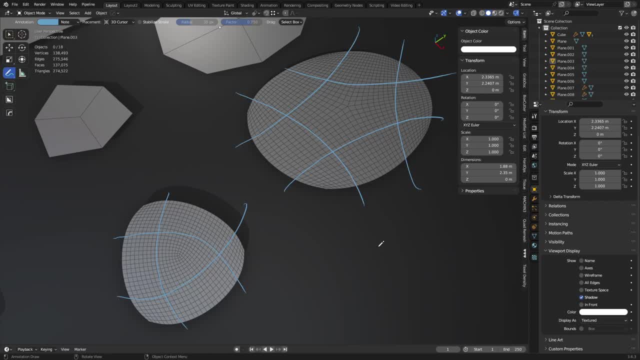 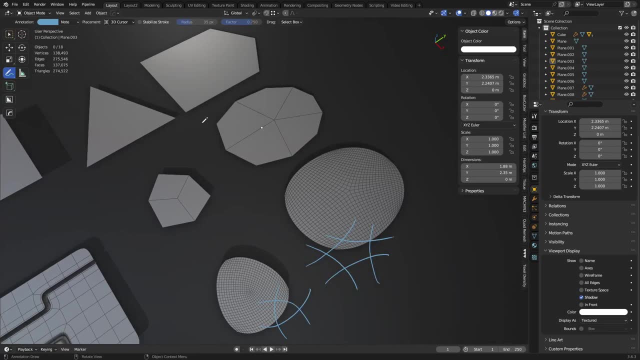 the e-pole actually is now. something that's interesting about the end pole and the e-pole is that it acts or behaves very similar to the triangle and end gun. obviously they were created from it, but when you have triangles, end guns, e-poles, end poles, you usually want to try to. 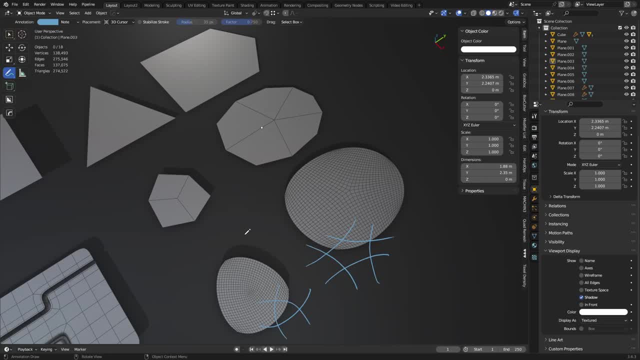 keep these on flat surfaces or planar surfaces if possible, and so when you're doing hard surface modeling, specifically, if you can bring these around or you can push these e-poles and end poles, or you can make your triangles or end guns on the flat surfaces, that will actually render. 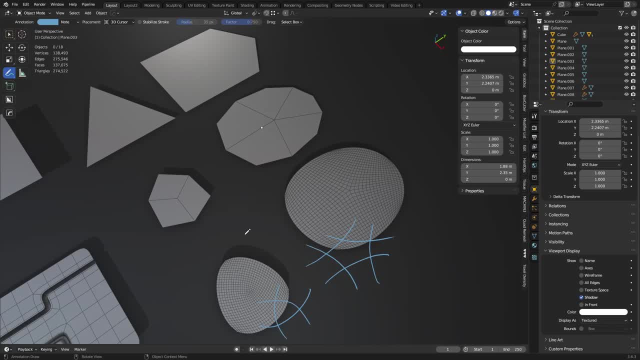 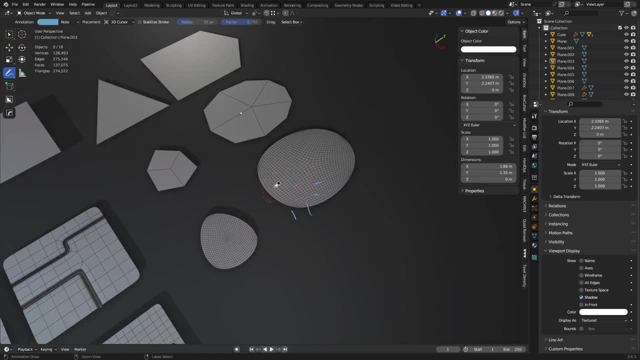 just fine if it's on a flat surface. even if you have a really crazy e-pole with like bunches of edges coming out of it, you won't have as many issues with it because it's on that flat surface. so so let's go ahead and dive into the end pole a little bit further. 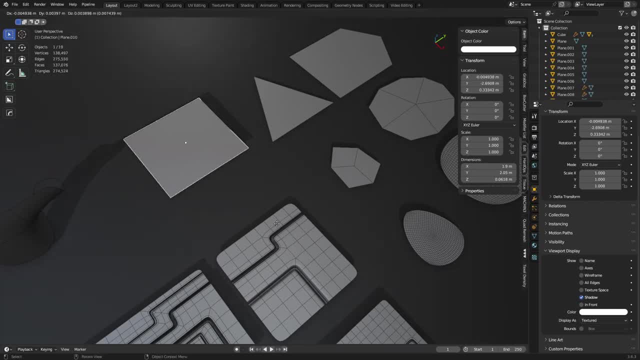 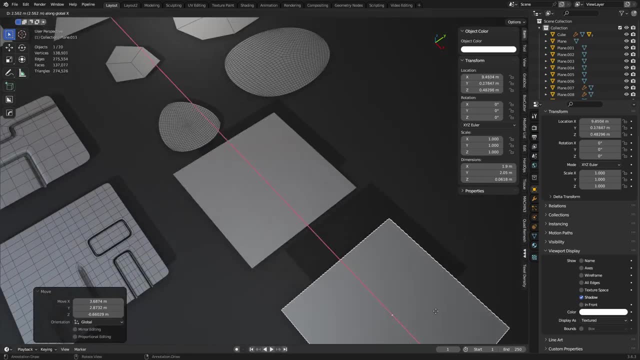 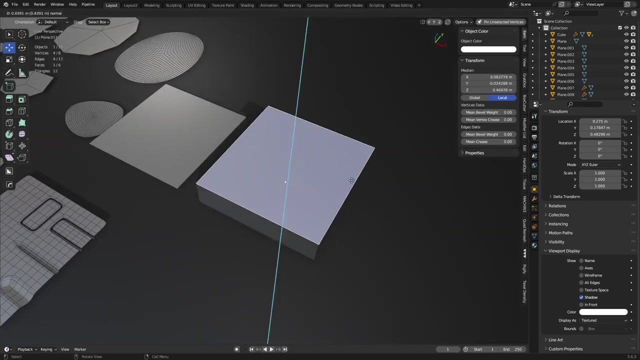 and we'll take this plane and we'll borrow it real quick and just kind of send it up here. so or we'll put it down here anyways, we'll make a duplicate because we're going to do this a couple times. so we've seen this topology before the: the end pole with the three quads, when you create a cube, it actually exists. 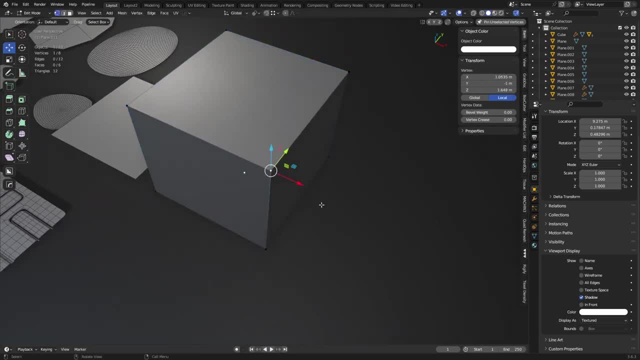 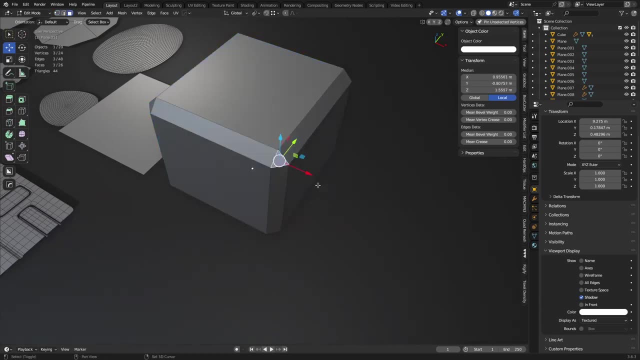 right here on a cube. there's your three quads, here's your end pole, if you've ever noticed that before, it gets better than this, of course. if you take a cube and you chamfer it like this, you see, you get the little triangles okay. so we know what a triangle is going to do if we 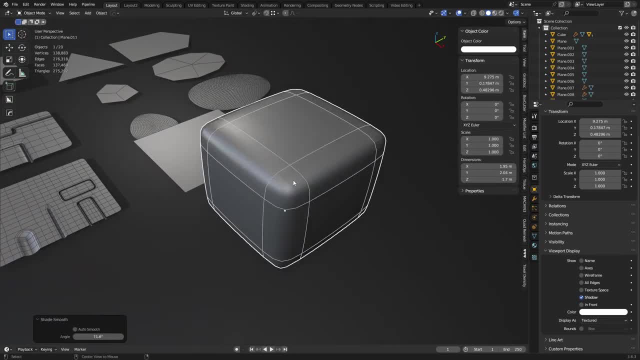 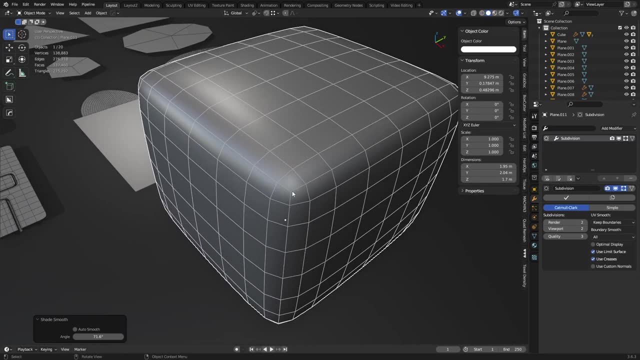 subdivide it. so if we subdivide this, we hit ctrl 2- shade it smooth. what we'll see is that we turn off optimal display. it actually does create a subdivided triangle, just like so, and so we have the end pole with the three quads there as well, and so this is pretty much what you'll see in a 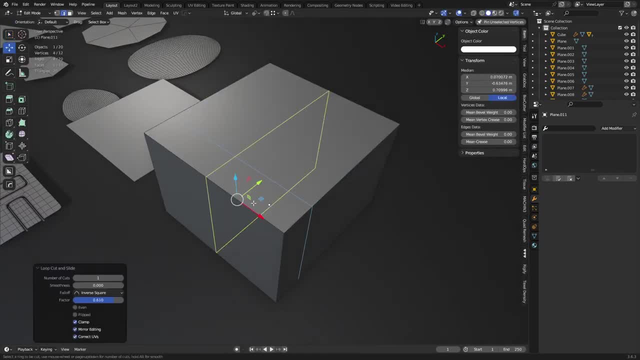 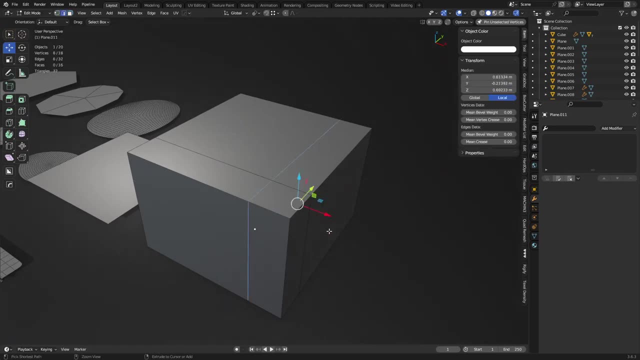 lot of tutorials where guys are adding loop cuts into the corners here to hold a subdivision model. that's the three quads. there's your end pole, also a regular bevel, right. if you took the whole shape and you put it in the middle of the cube, you get a three quads and then you put it in the middle of the cube. 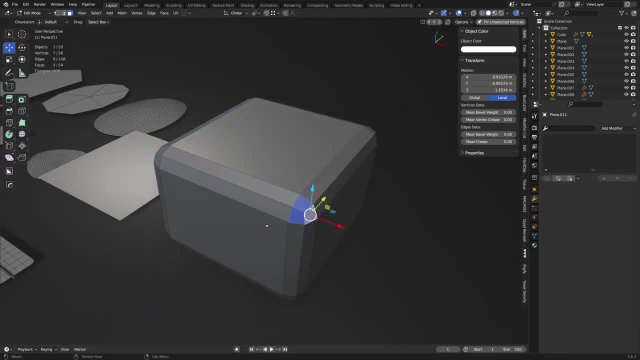 and you put it in the middle of the cube. and you put it in the middle of the cube and you put it in the middle of the cube, beveled it, you get the three quads with the end pole. just wanted to point that one out for you. 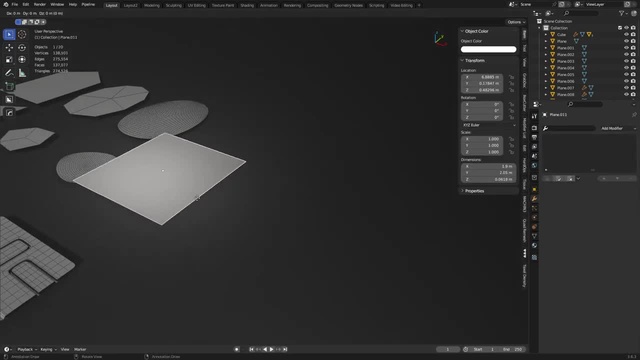 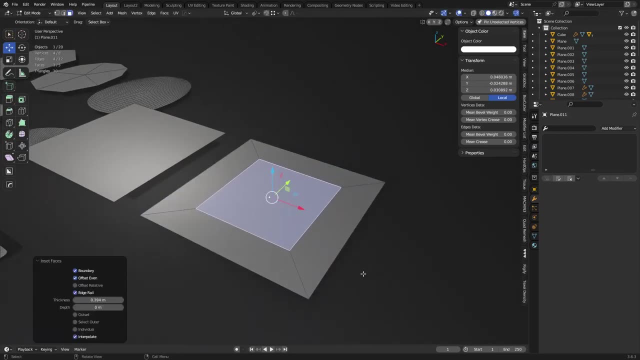 it's kind of common. you'll see this shape take place in a lot of different areas. so even if you had done an inset on a face right, so you press i on the inset, cut this in half- you'll start to notice something kind of familiar here. press y and rip it. move it out real quick. 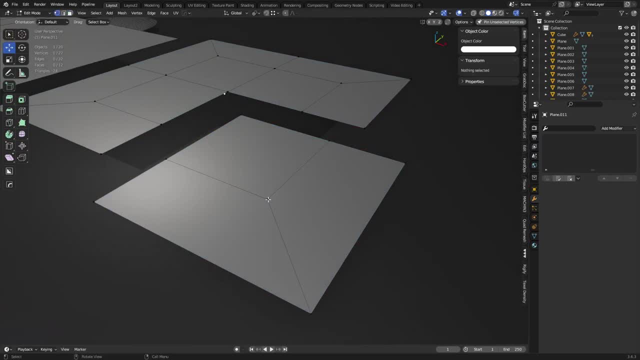 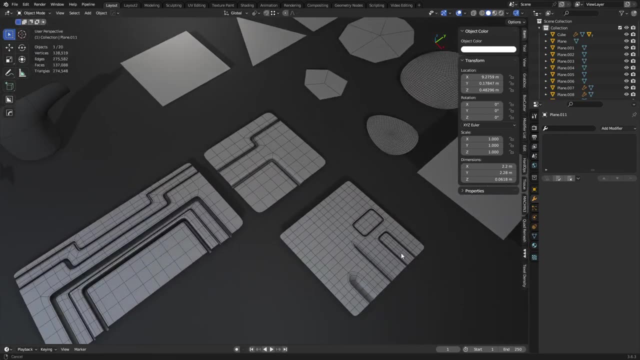 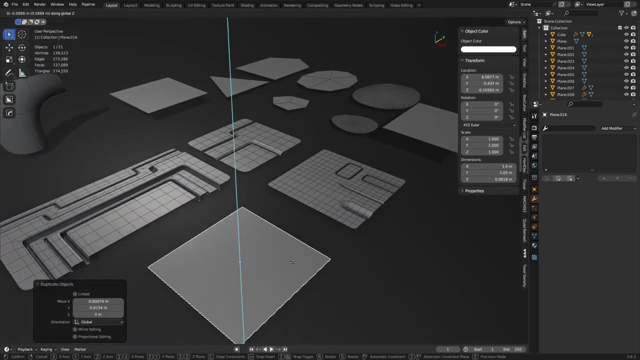 okay, this is in fact an end pole with three quads, so even your inset is the same. now, this is where it gets fun, because when you have a plane and we're going to put a grid out on it, we're going to subdivide it a few times. 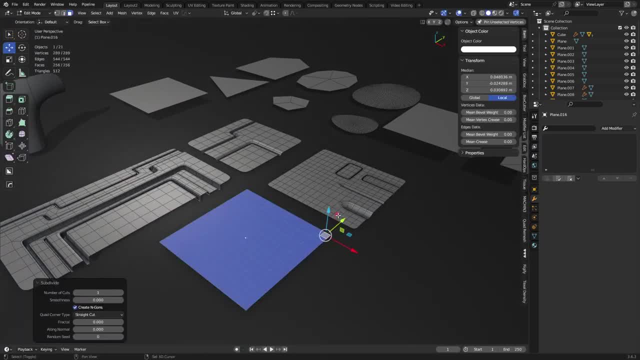 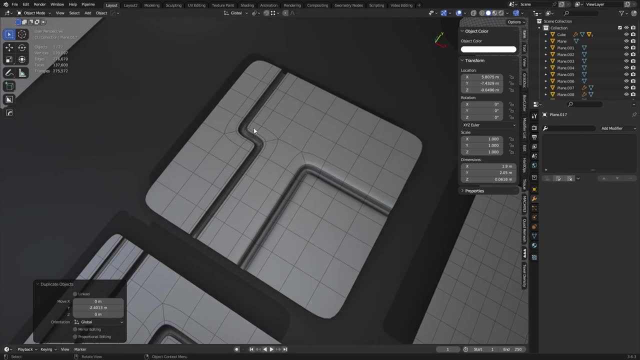 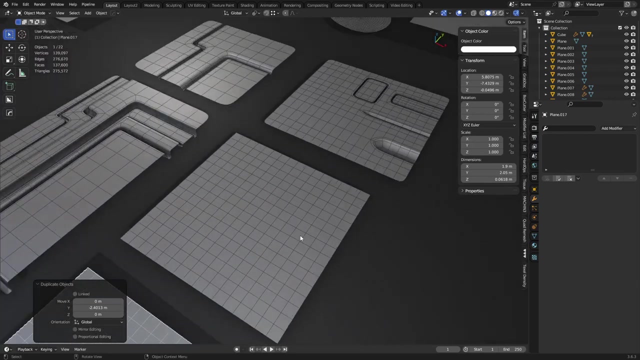 and we're probably going to use that twice as well, so we can start to see that these have kind of a flow to them where they're going through the shape here, okay, and that's happening on all of these, that same kind of thing going on. all right, this is going to be your redirect slash edge flow. 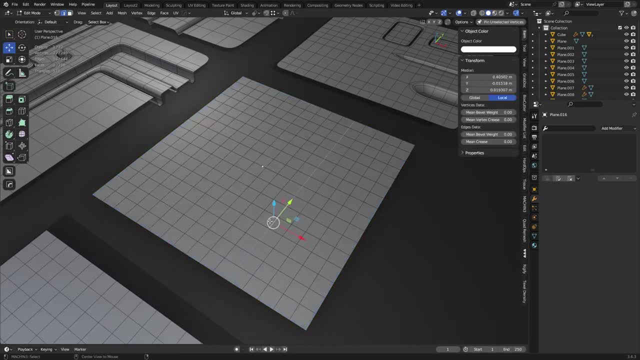 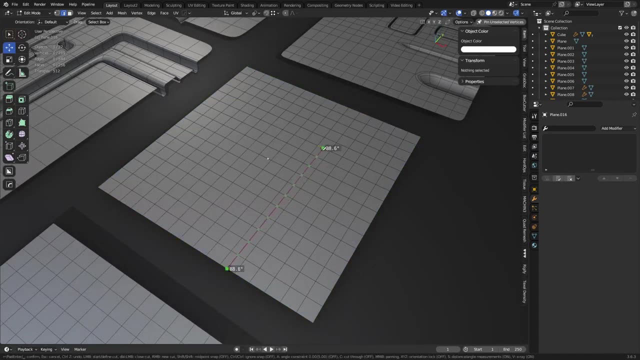 so we're going to use that twice as well. so we're going to start to see that these have kind of a flow and you have a plane like this: it's subdivided. these are your edges, these are their flows. right, it's pretty simple. however, if you use a knife tool, you can cut out and you can even press x, y or z if 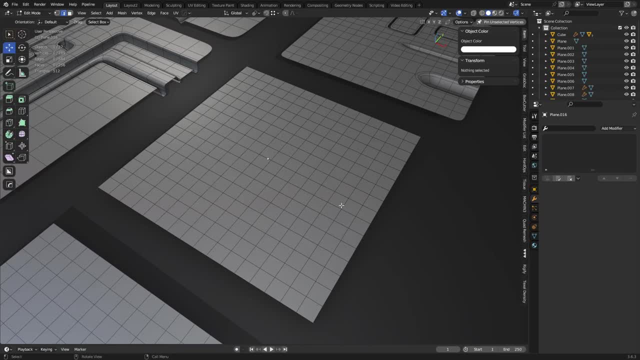 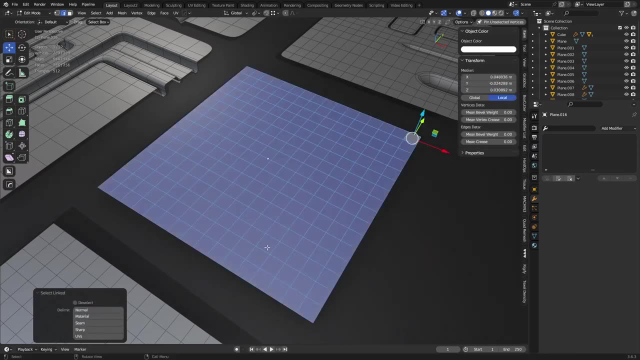 you need to. or you can hit a, or you can actually do. hit a twice and you'll line up to: oh, i guess it doesn't work on this same example. oh, my bad, you hit a, though, and line up on angle as well, but this usually lines up. 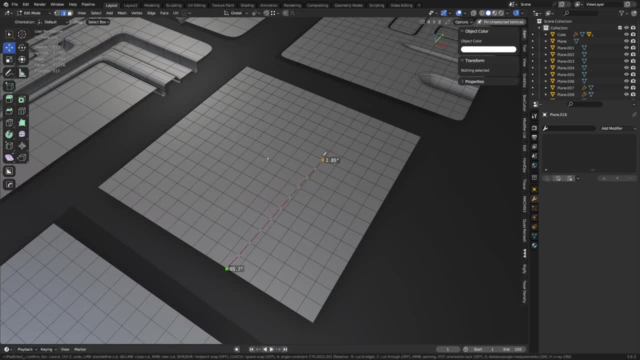 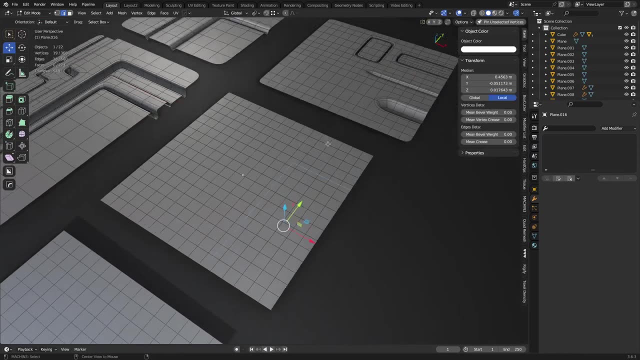 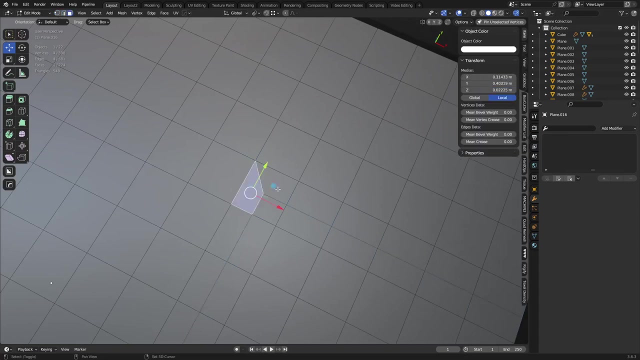 between two faces if you hit a twice. unfortunately it doesn't work if you go across that, so we'll have to hit y in this case. now if we hit x, we can go this way. okay, look what we have going on here now. if we press k and cut there to there, we've created the three. 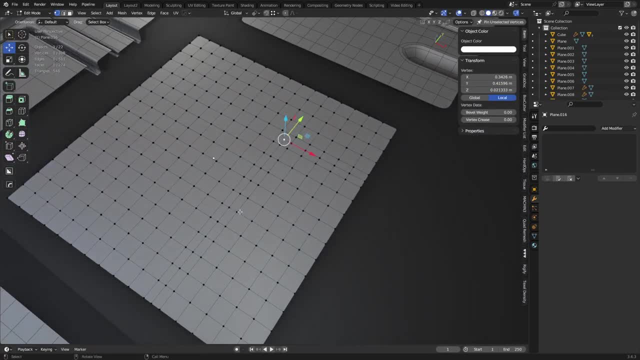 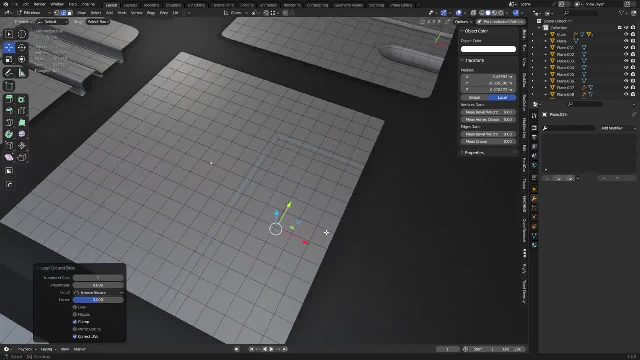 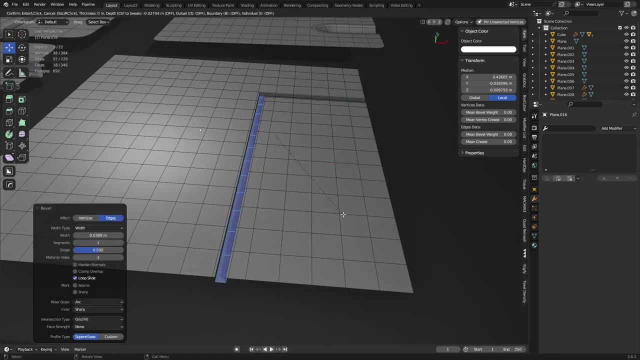 have the same amount of vertices so we can hit ctrl r and we can loop, cut through that if needed, so we're able to control our edge flows, so we can actually send this all around a model, and i'm going to do an insert hole control and hit b so we get rid of that little border down there. 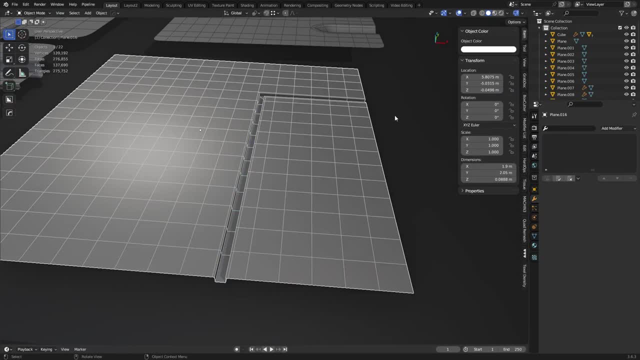 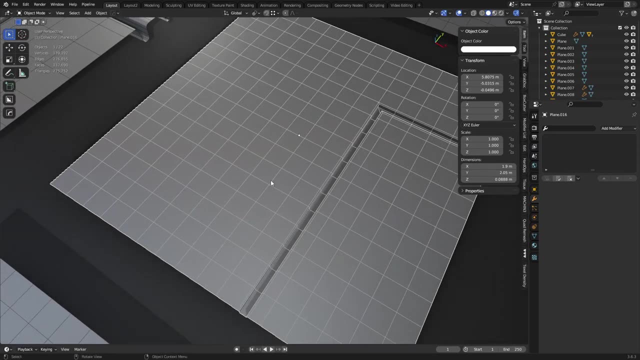 okay, so we can do this all around our models and kind of direct the topology around on it, at least edge flow on the topology, right? so in reality topology is just the relationship between the- uh, the different edges and vertices and whatnot, and that's all really it is. it's kind of arbitrary in nature. where you can have good topology, you can have. 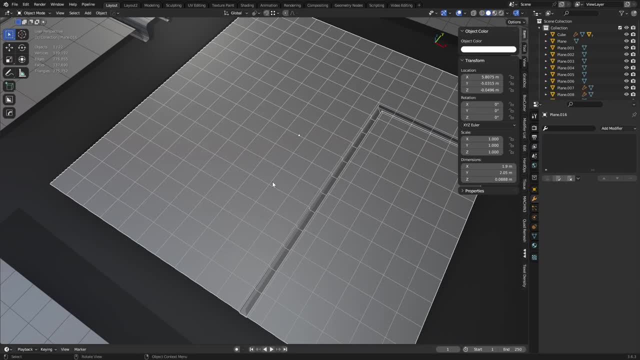 bad topology, but if something works, it works at the same time. so when you're doing like meshes that you want to bake high poly to low poly, it doesn't really matter if it's a perfectly clean quad mesh, if it's not deforming, you're just baking it like you could use triangles ingons. 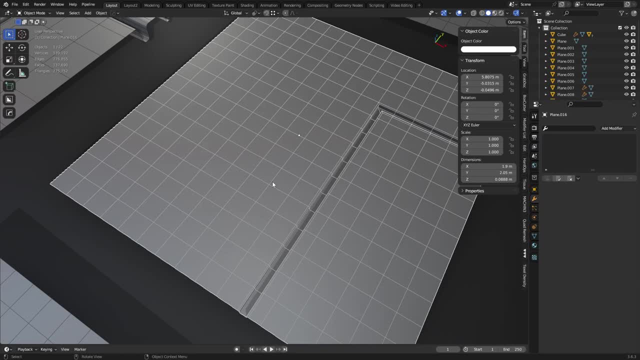 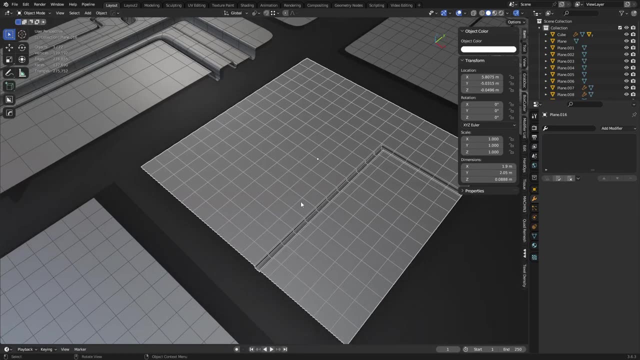 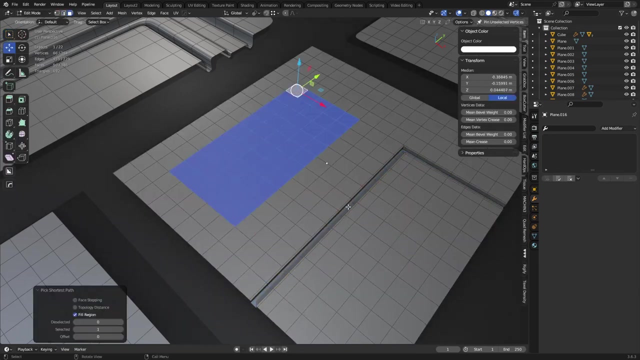 and it can be relatively messy. you can have quite amazing, amazingly bad topology and still use it. but you can see we can control that edge flow, which is nice, and we're going to go ahead and do an inset real quick. so when we inset something, it's doing the 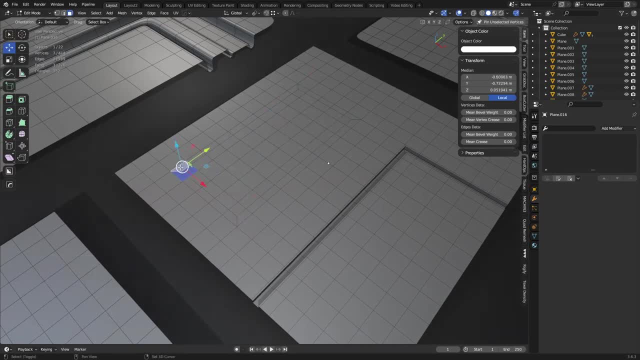 same thing, right like we have our quarter inset here, but it does it four times, so it loops back around on itself and so that's just a loop. you can have a loop anywhere in your model as long as it comes back to itself, so you can push that in and subdivide that. there you go, we have something. 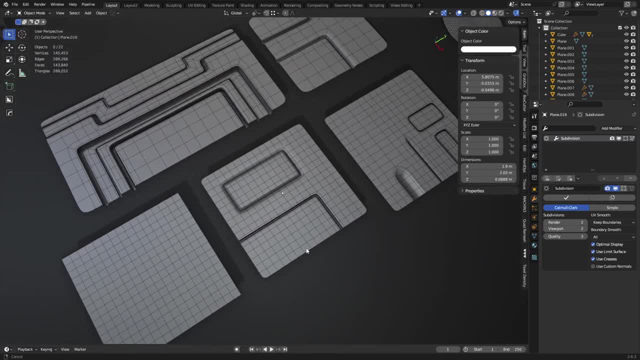 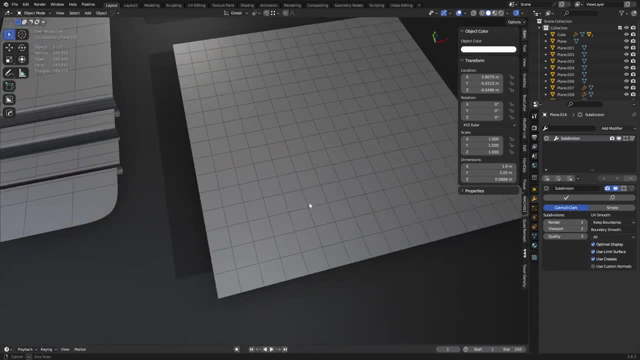 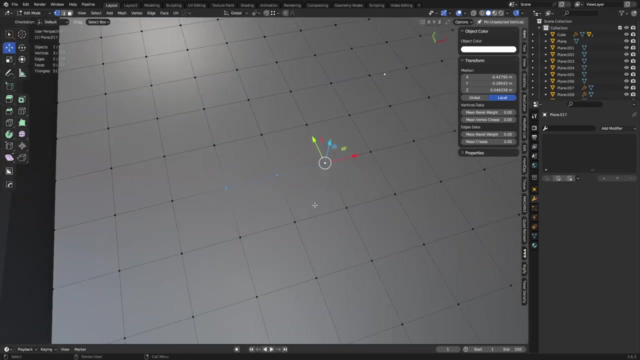 like this going on in this area now, all right now, a lot of those topology guides you see online or some youtube videos even they get kind of confusing because they're talking about all these cool techniques of doing reductions. so a lot of times you use end poles for reduction as well and you'll say, like, take three vertices. 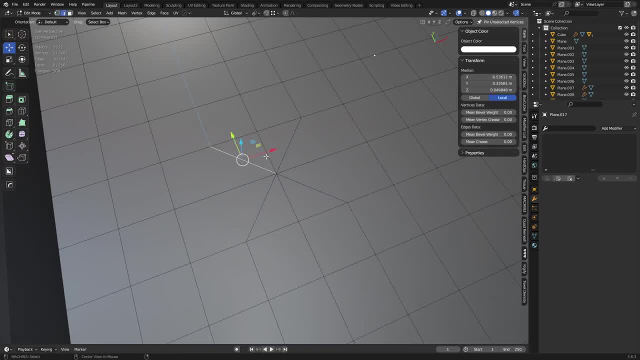 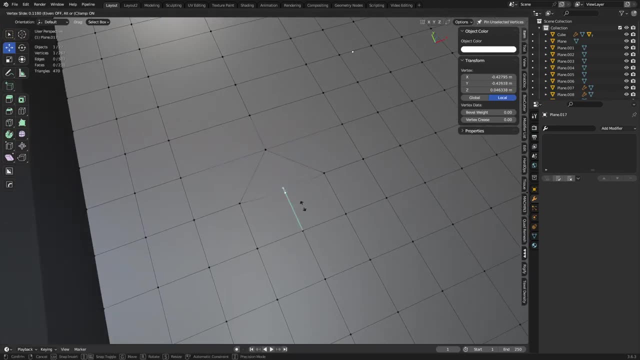 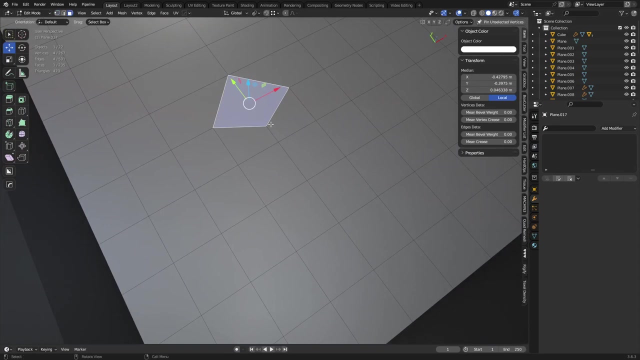 merge them together. so press m, merge at center. alt click, alt shift, click, control x, right, and we'll get something like this: now we control x here to quickly dissolve that. this dissolve selection, by the way, control x, and if we gg twice, we pull that back. what we see here is we turn these three edges into one. 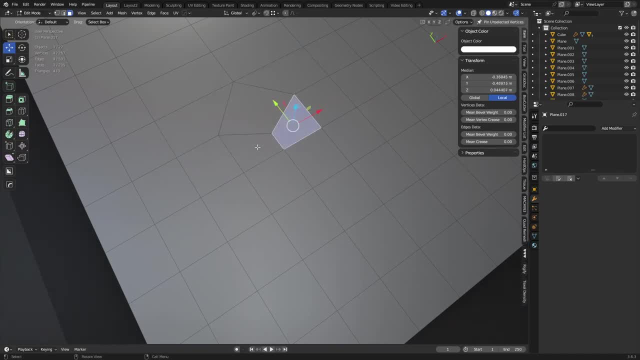 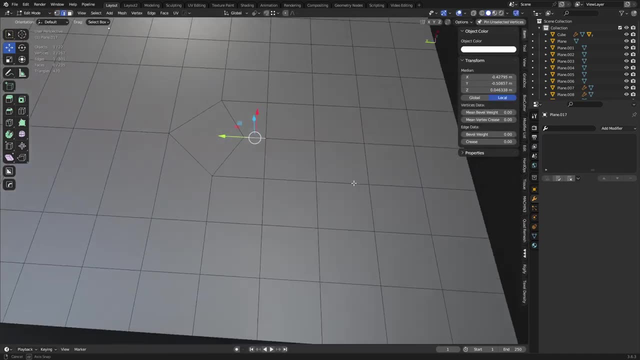 basically. but we have all quads everywhere. now you probably didn't realize it. but what we've created here, you guessed it: three quads and an end pole, all right, so it's the exact same topology, it just looks different. so once you start looking for this in your models, you're going to have much, a much. 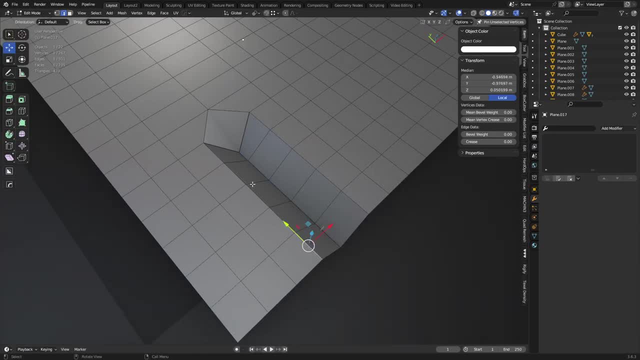 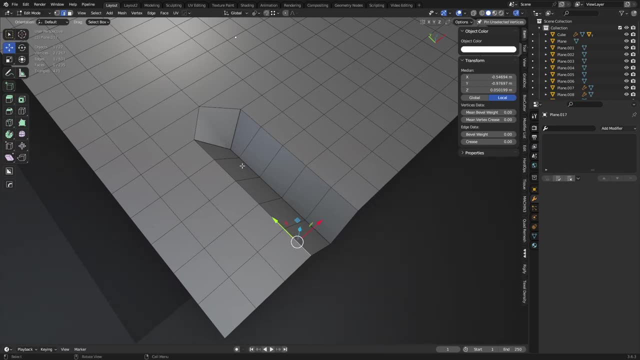 better time working on your models. this impulse is extremely important, like i was saying. so edge- oh, by the way, you can alt s to scale along normals and that's what i did on that middle edge. so control, click around this. we'll hit control b, we'll do a bevel mouse wheel up once and when. 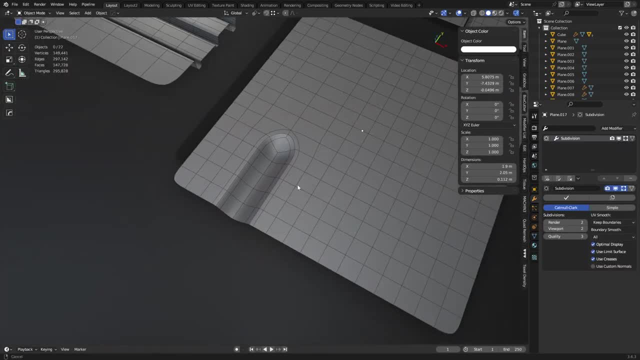 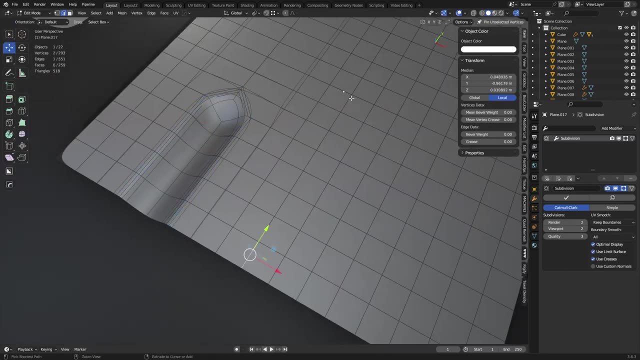 this subdivides. we'll get this kind of shape here. okay, someone was asking how i do these really small little um, crease lines and whatnot, and that you can simply bevel an edge. there's nothing fancy about this. so if you bevel an edge, you mouse wheel up once, just so you get a little triangle here at. 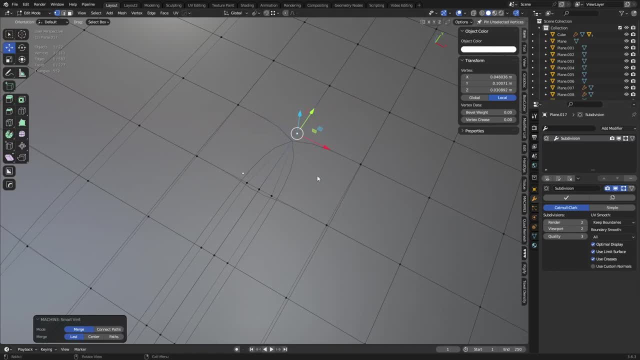 the end if this triangle runs all the way out this way, right, so we merge. it's kind of hard to see what's going on, but we're going to merge that vertex to this vertex and we dissolve that there. this is the same topology, guys. we just made it off of one single edge so we can grab that whole edge. 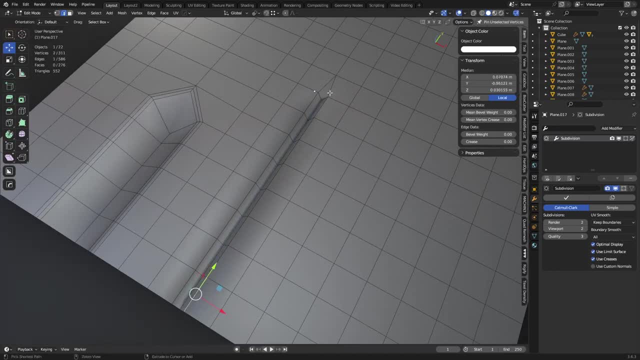 down the middle all s push it in, grab these and go all the way around with it. now we can control b, just control b. okay, mouse wheel up once and there we go. so we can actually create something like that as well. now, this may be a little bit. 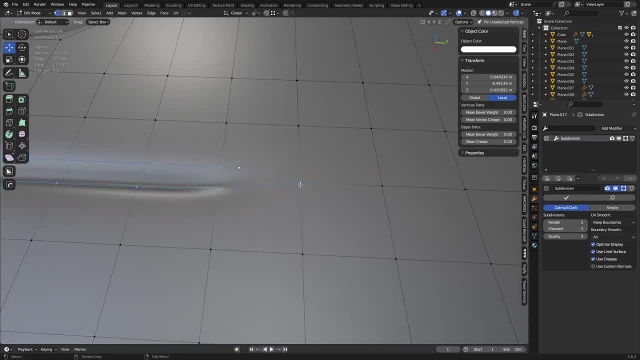 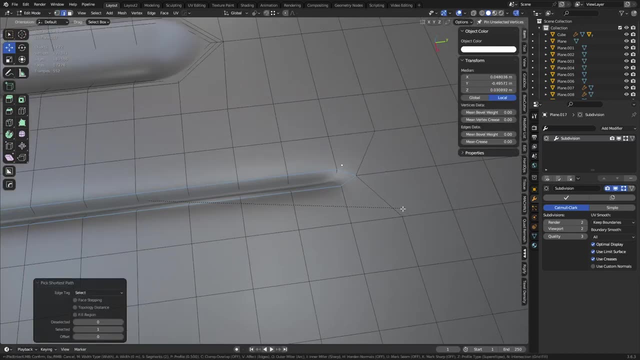 stretched out here at the very end. so before you do that, you might want to try to pull that back a little bit on y and try it again, see if that goes a little bit nicer. this is part of balancing. sometimes you just got to push and pull your vertices around and try to get them to. 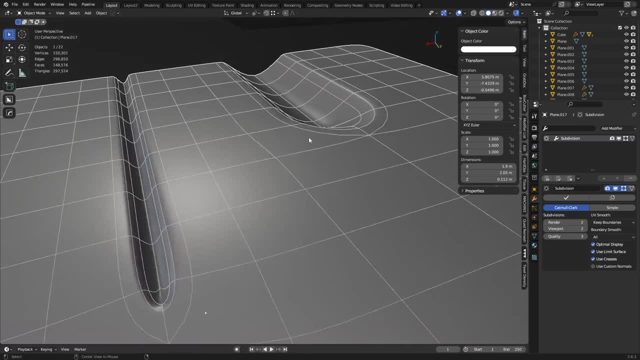 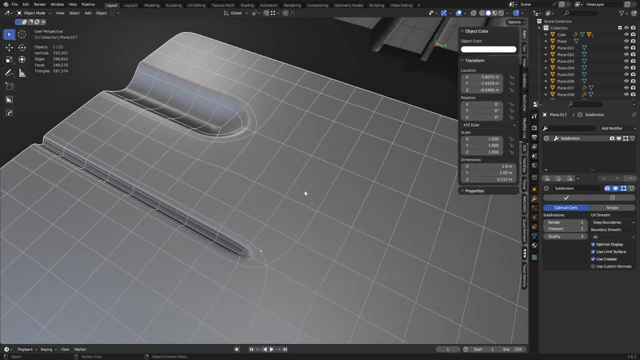 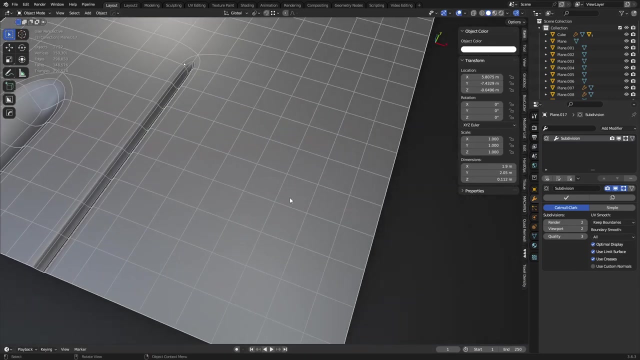 be in a correct position, or sometimes they'll turn out nicer. so do try to nudge things around a good bit and see if you can get them behaving the way you expect them to. so that's just one example of doing a reduction, perhaps, or creating this kind of shape anyways, but what we can also try is three. 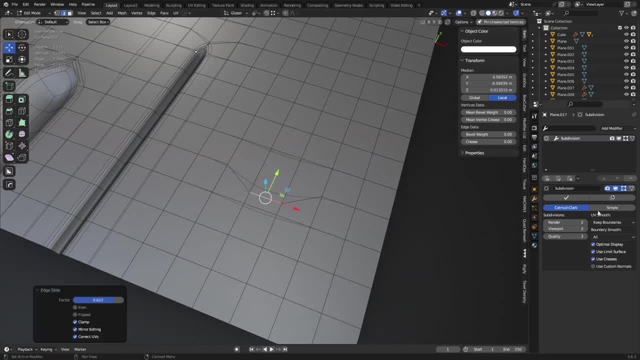 to one. so a lot of guys do this one. they'll press gg twice, so pull this back and turn off subdivision and edit mode. they'll take these two vertices, hit j and join them. now these ones right here we can control x and dissolve. so we can alt shift, click these and control exum and what. 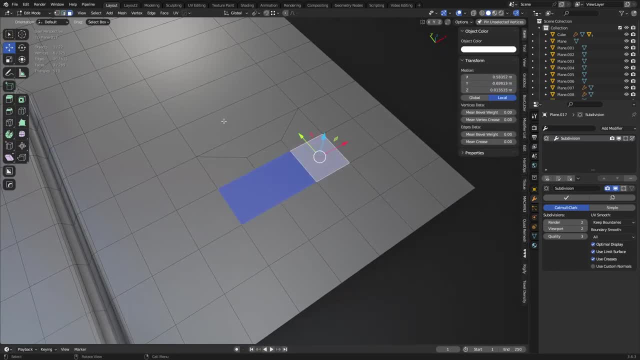 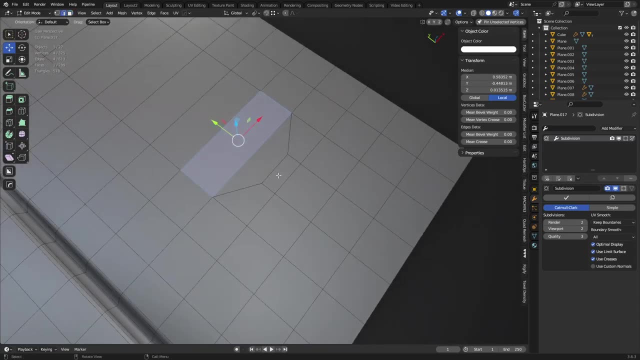 we'll see here is: this is now being reduced from the three faces to one face right, and so when you do that reduction there, it seems like it's really fancy how we went about doing it, but it's really not anything fancy. put a loop, cut down the middle, you realize these are two quarter insets. so 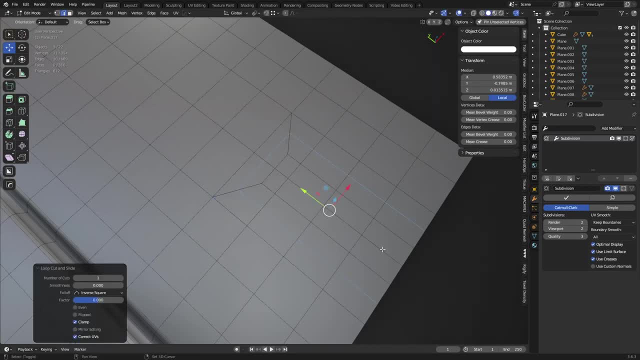 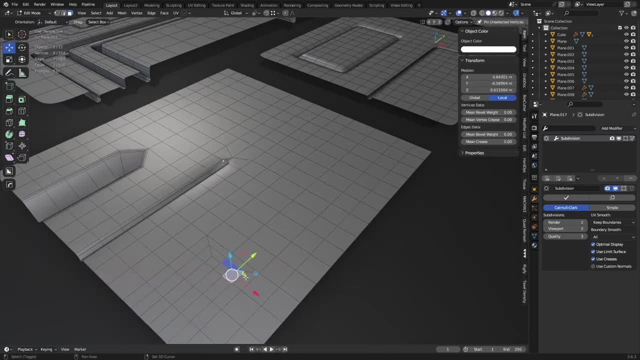 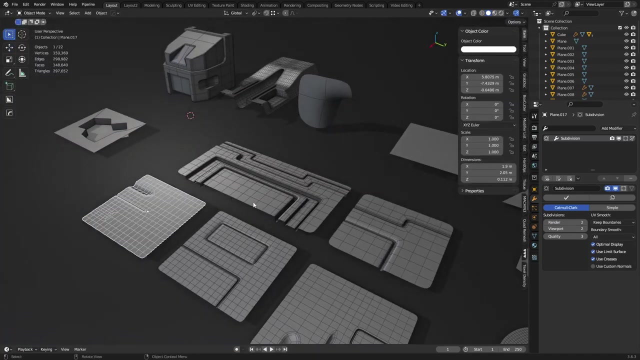 basically, we've created half of an inset, and so we can do these kinds of things, though as we're working on our models. it's just different ways of approaching, creating that- that same topology over and over and over again, basically so we can have better control over a mesh entirely okay. 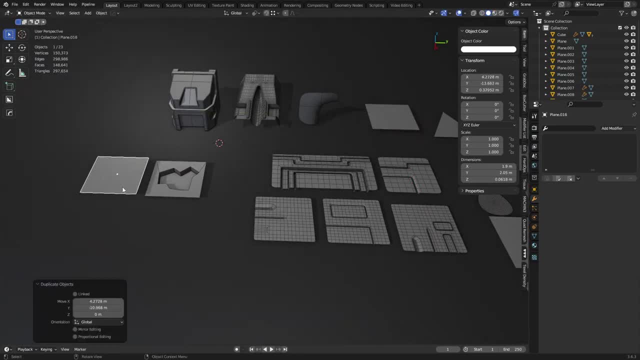 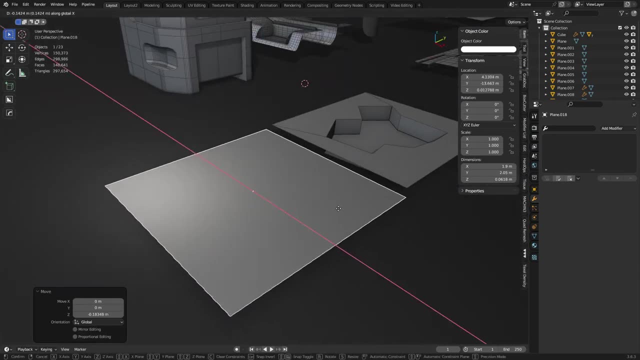 as we work through our projects anyways. so here we can see, we got a plane. now, as i was saying, you can use triangles and ingons on planes and as long as they're flat, they work out really well, and that's what's going on here. so if you ever want to just go crazy and take a knife tool and 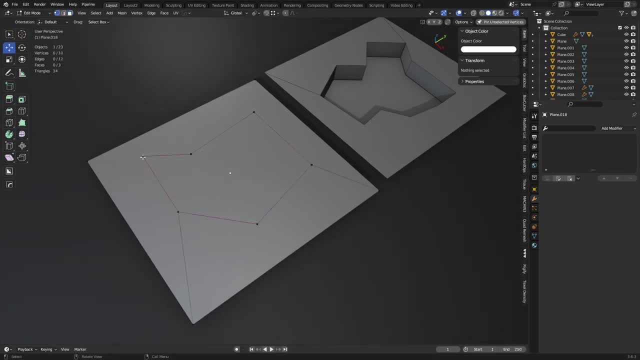 cut in a big shape or do some kind of weird cut like this. perhaps maybe you want to bevel a vertex. you can hit ctrl, shift, b mouse wheel up a couple times. you can do things like this. guys, you see, if we bevel that vertex we get a bunch of nonsense over here. we're going to play with that here in. 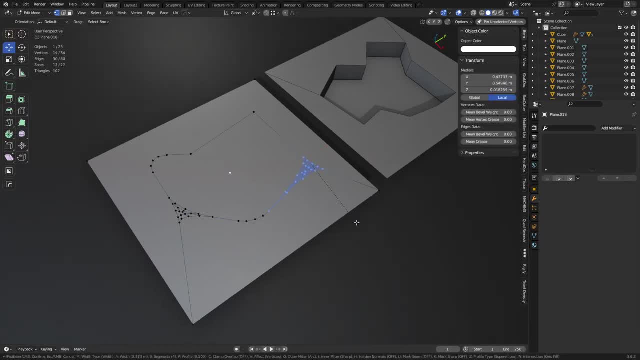 a second ctrl shift b, again ctrl shift b. that one didn't work out too well. let's see if we can dissolve that we can't, so we'll come back to it, because we're going to quickly bevel this one. join it to here. sometimes you have to have two edges throughout a shape, so just keep that in. 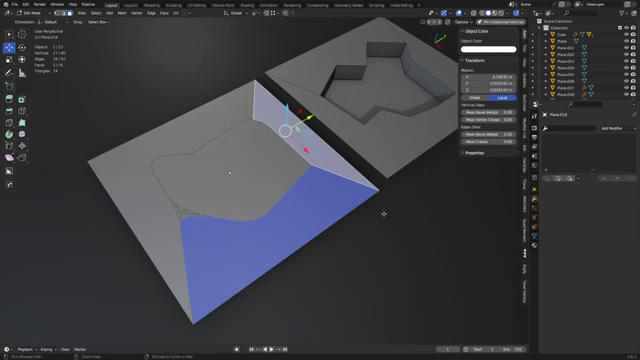 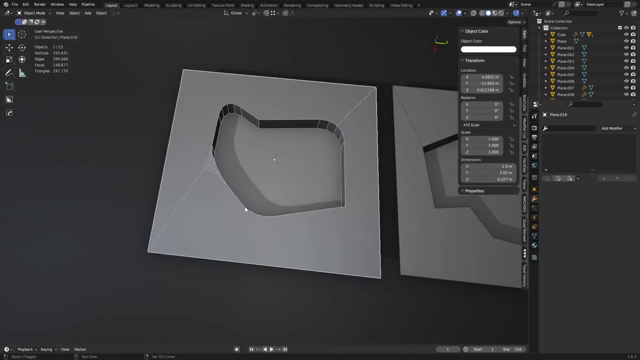 mind and you might be able to dissolve this now. sometimes you got to select the faces instead and hit ctrl x. you can see that went away, but we can't extrude this down and we have this going on in here now, which is quite nice. problem is is we have this mess over here, and so a quick way of 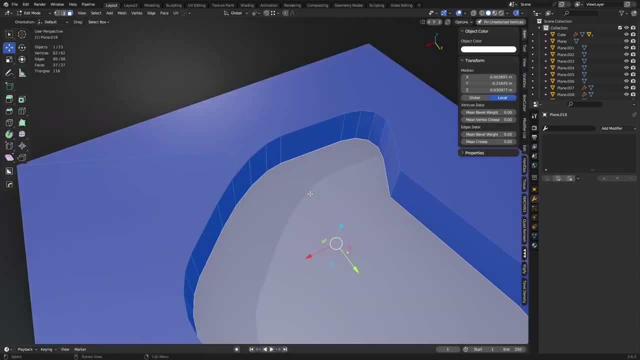 cleaning up a lot of geometry problems is you can press a x and do limited dissolve and limited dissolve is going to dissolve anything that's flat, so we pipe in 0.05 over here so it doesn't try to dissolve our curves here that we just created. you can see how that works out. it works. 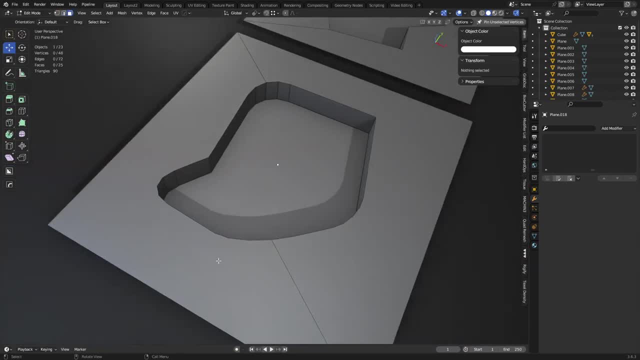 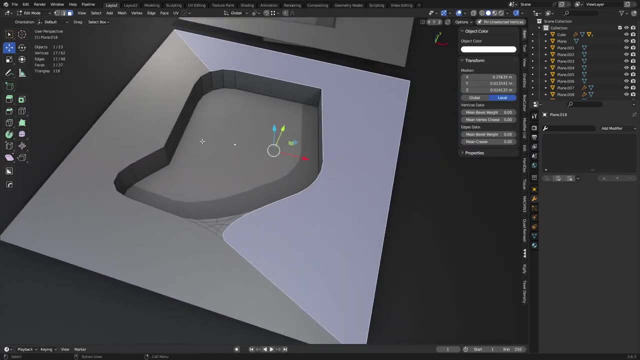 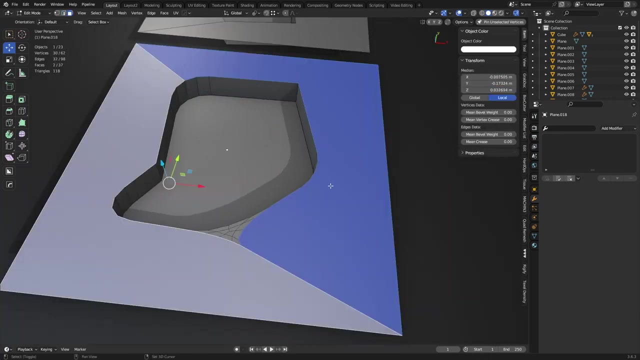 out pretty well in this particular area. now, sometimes you don't want to do the whole mesh at one time either. so, and let's go back just a second- let's say we had something happening in here where the bevel was much higher resolution, but we wanted to preserve that. we would want to just select these faces here, right? so what we could do. 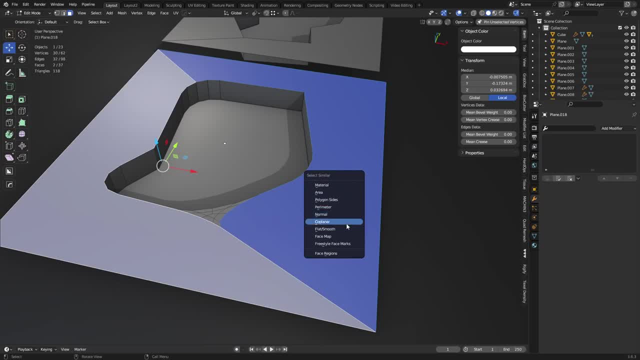 is they're flat, so we can press shift g and we can select co-planter, so planter faces, co-planter faces, and now we get that right. so, but now we can just limit, dissolve this section. instead, if we wanted to, we can always go back and we can do things like bevels still perhaps. so you might. 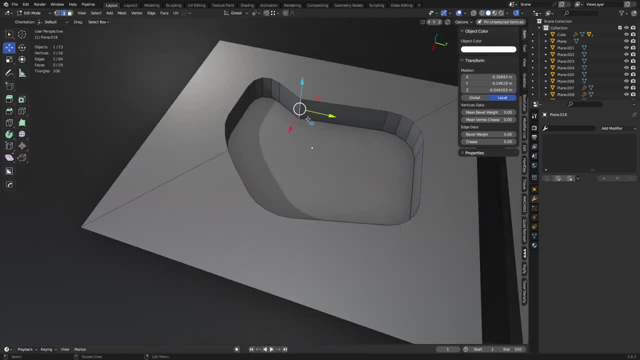 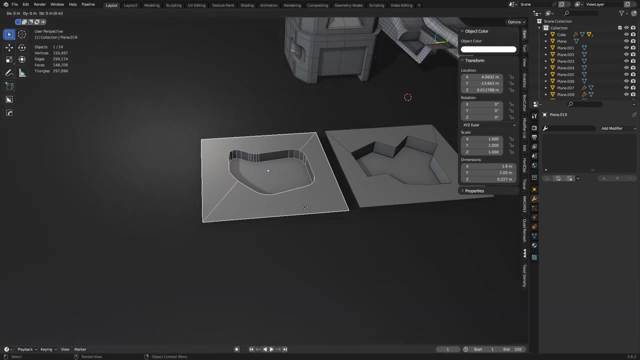 have to hit v to turn off the vertex and we can always go back and we can do things like bevels, but we can go back and tweak that as well. quite useful, so that's just a fun way of going about doing something like that. now, of course, you can always take a mesh, a m merge at center. i'm going. 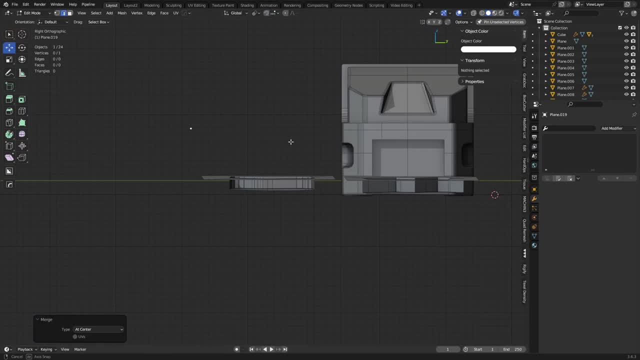 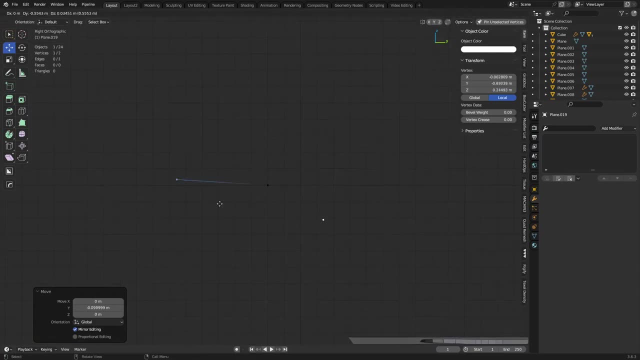 to turn on absolute grid snapping. so increment absolute grid snap. i'm going to hold alt while orbiting to jump into a side view and press 1. i can select that one vertex we have here. while we move this we can hold ctrl, snap it to the grid so we can start to lay out edges in this manner as 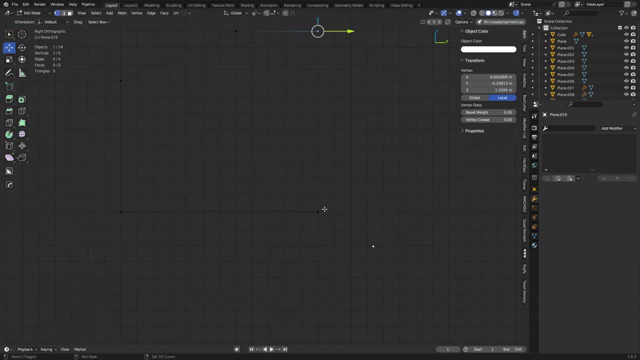 well, all right, or vertices, so we can create all kinds of cool looking ingons here. you can take an edge, you can subdivide it. when you subdivide an edge, you can hit ctrl b and you can actually bevel it, roll b and b. that is so. if you wanted to do that, you could. 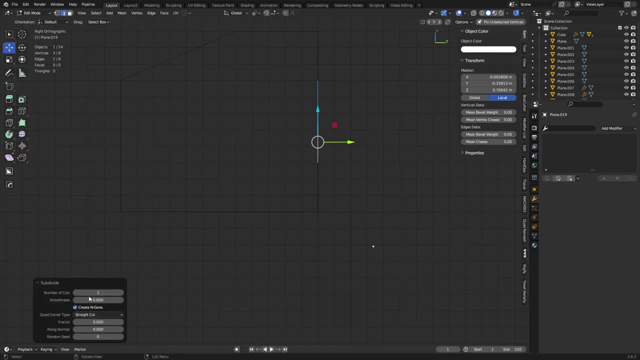 when you so- excuse me- when you subdivide it as well, you can actually increase the number of cuts, so you can actually bump them up. if you need more in a particular area like that, you can also loop cut these things as well. so that's actually a little bit more easier, do that. but 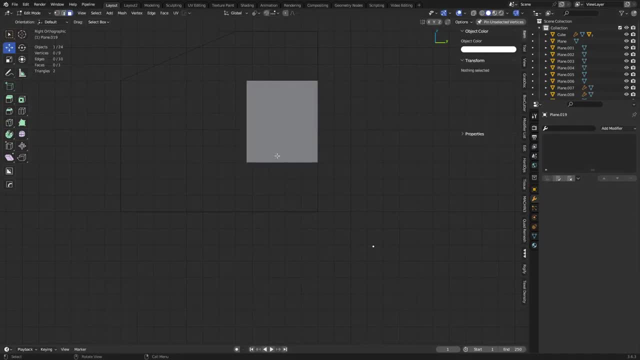 whatever the case, you can also extrude edges. you'll see it creates a face. you don't want the face. you can just delete only faces. maybe we don't want that edge, so delete only edges and faces. there we go. so we have this shape now, all right, so we created more or less. 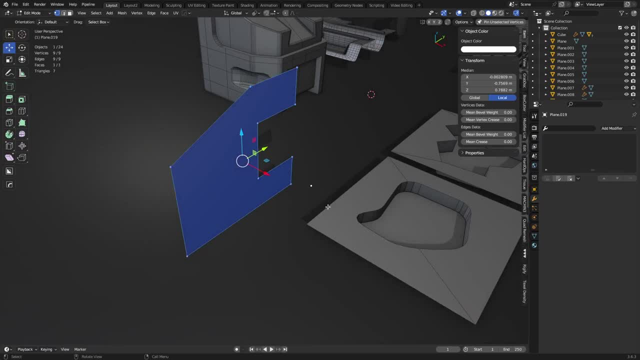 something like a string of vertices. now we can press f and we can just fill that. sometimes it won't fill correctly. you might have to add additional. you have to fill it in like little chunks and then add additional edges, perhaps sometimes ingons, just they're not able to be. 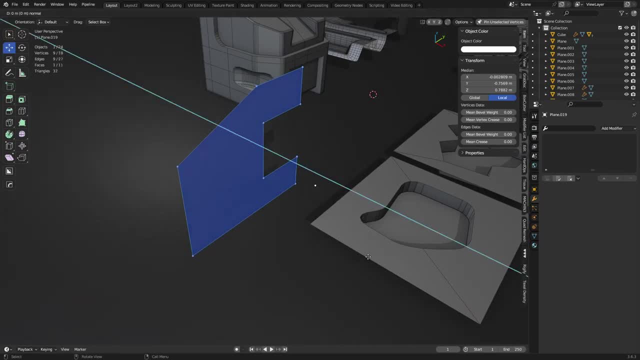 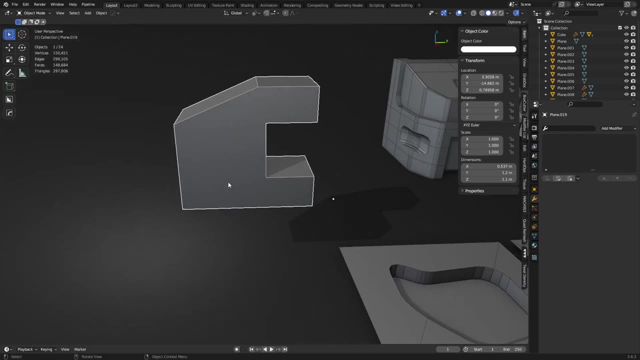 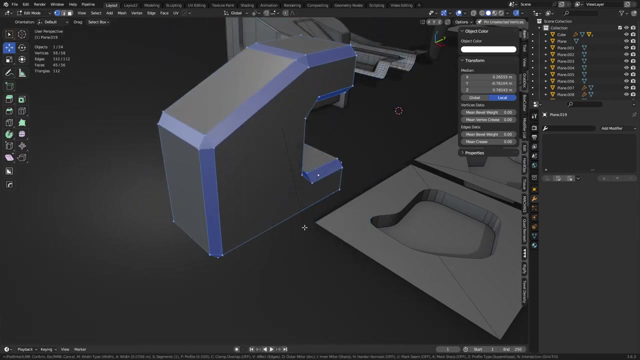 supported with just one face. but, um, we can press e and then x bring it out in this direction, so we could create blocking shapes like this very quickly, which is quite nice because we know how subdivision is going to work. we could get away with at minimum a chamfer on something like this. this is going to get us off. 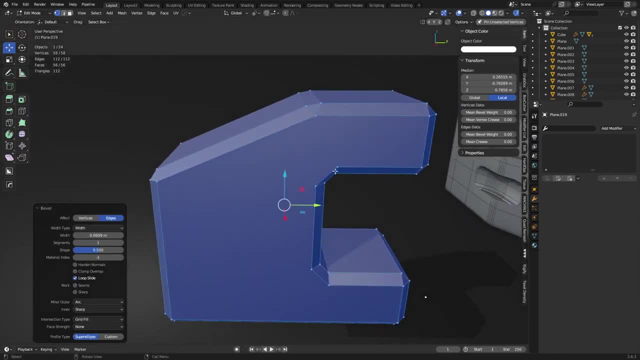 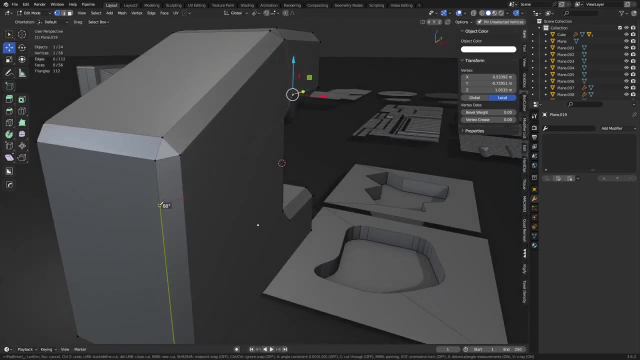 into the ballpark of working on this as a sub d mesh and we would have to start working with it, possibly and turning it into quads everywhere. and so now we're getting into the part of where you're going to want to run, possibly, your edges across symmetry, and this is going to save you a lot of time, but it's going to. 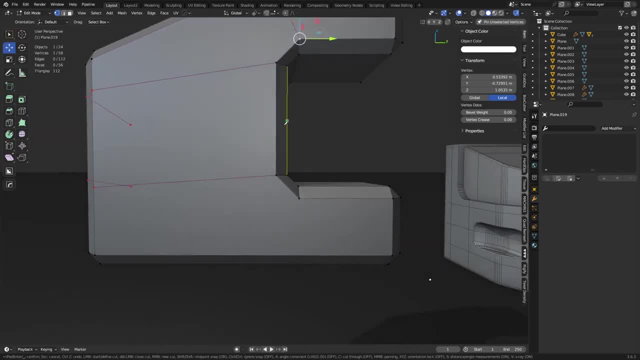 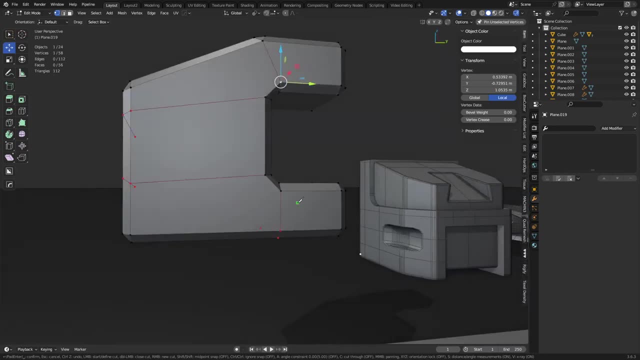 become kind of boring when it comes to a 3d model as well, where you start running across symmetry. you can see here this segment- because we did the chamfer creates a big end gun here, so it's a little bit harder to work with these sometimes, but sometimes they're not too bad either. so you 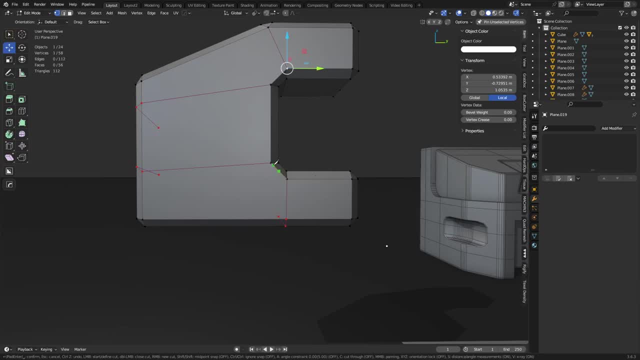 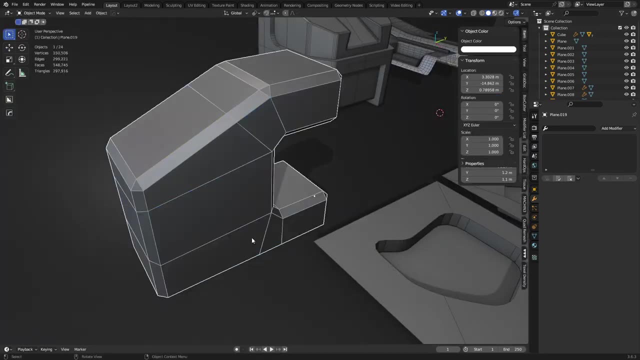 ever get stuck on the center of an edge. that's the shift key that does that. but, um, you just hit shift again and probably turn it off, so you can see we can start running across the symmetry here. perhaps our symmetry is actually all the way over here in the corner. so in edit mode i'm just 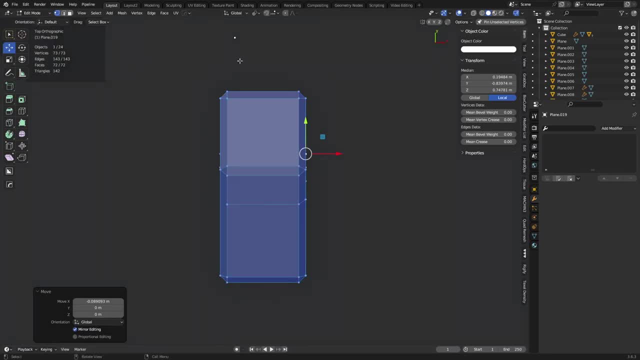 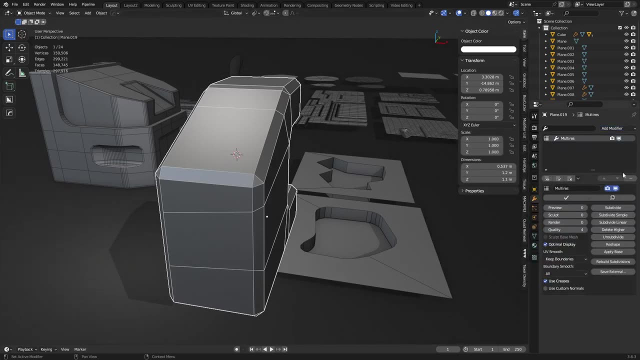 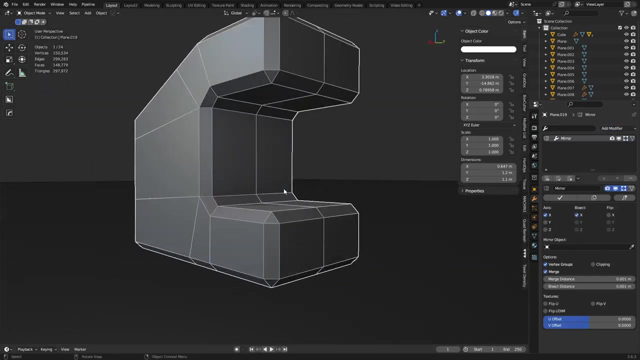 move it over a little bit, so our symmetry will be kind of like: right here we're just going to use the origin point and we'll do a mirror modifier. no, not multi-res mirror, we're going to bisect it and it'll do a number like this, and so this is what we have going on now. 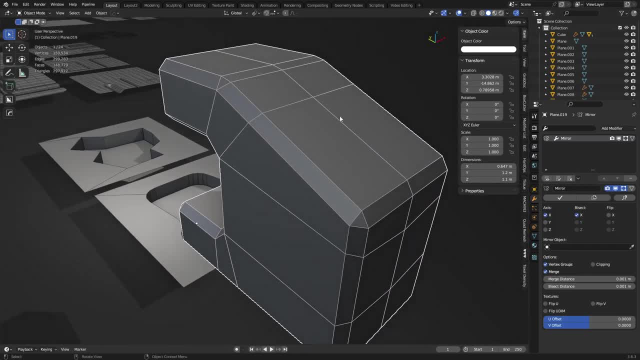 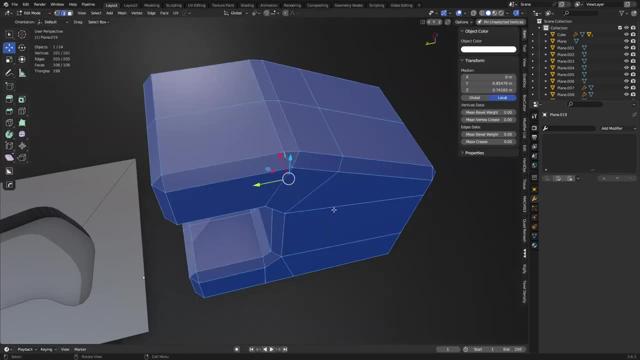 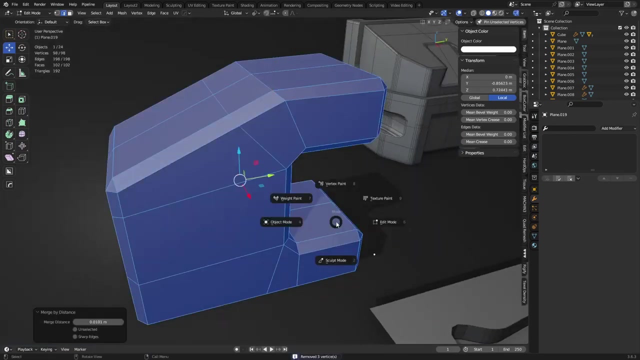 and this edge flow is just basically running around, but back around the um, the model here, so we can apply the mirror. perhaps sometimes you don't need these additional edges. push them forward, do things like that. so this may be an acceptable game model at this point if you actually shade this auto smooth and max the auto smooth out. 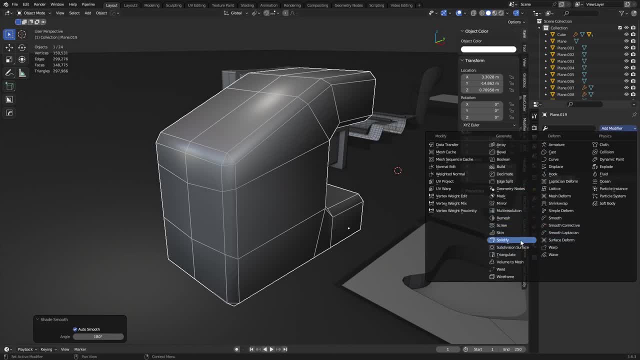 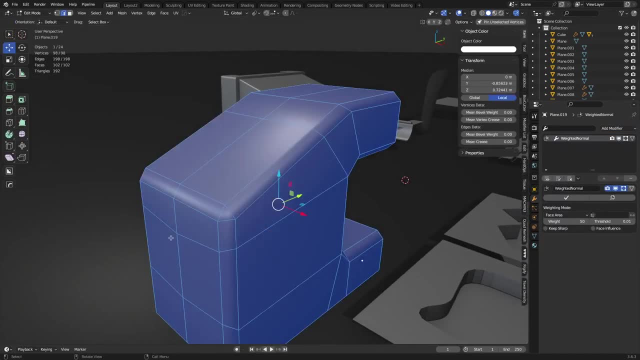 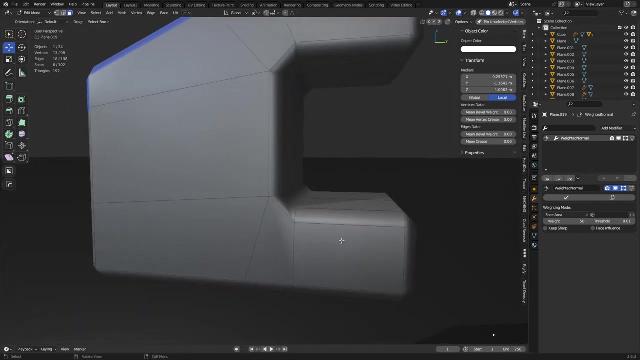 okay, and then you add a weighted normal modifier, the- uh. the best thing here for this, when you're using weighted normals, is you need at least a minimum of a chamfered bevel on the edges, generally speaking for hard surface shapes anyway. so that's going to help the shading quite a bit, but it 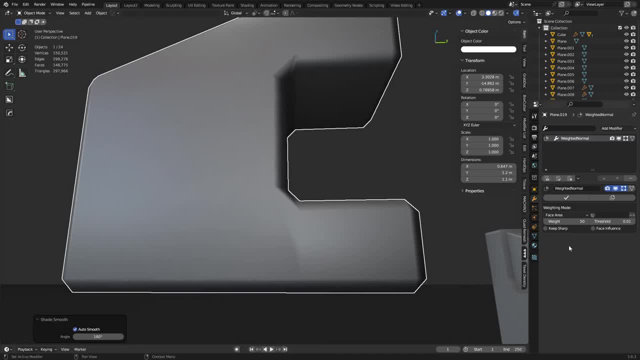 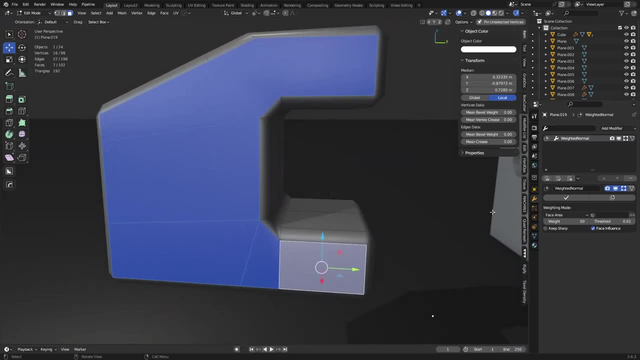 doesn't get everything perfect usually. sometimes there's just little nuances that are left, so you might use something like face weighted normals. i made a video talking about shading and how this, how all this works, but what you do is you use face influence. keep sharp, weighted normal, right. 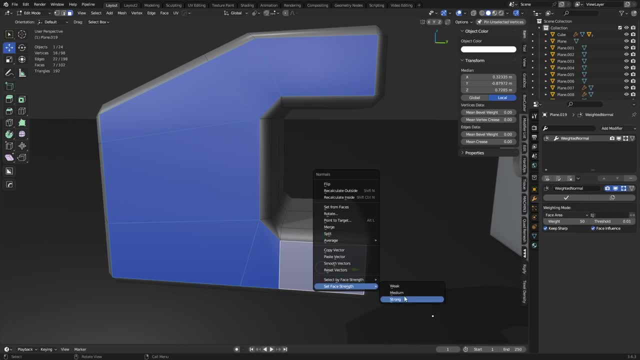 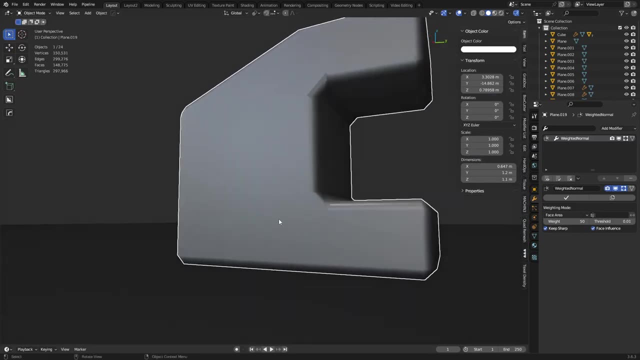 and then you select flat faces all in, set face strength to strong. all of them are medium by default, so you want to set these ones strong and that should clean up the shading a little bit, a little bit more, even if you have little errors remaining. so that's something that's good to. 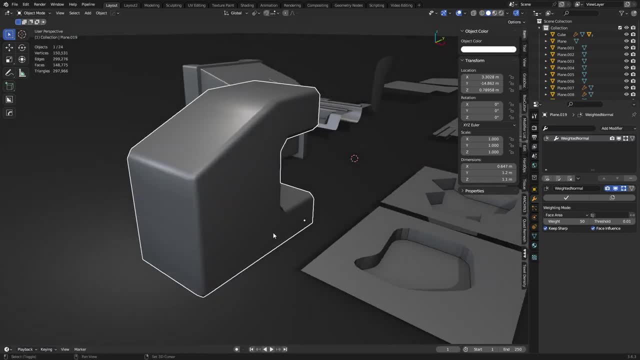 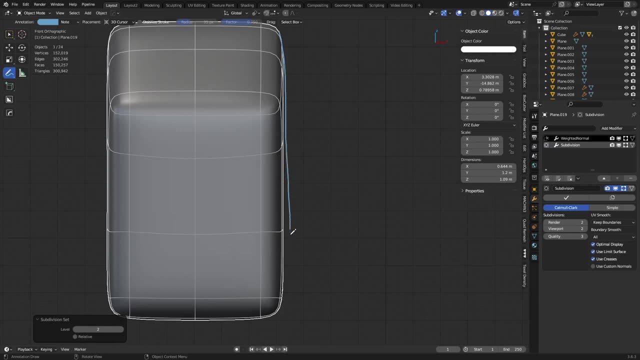 remember there all right now, this will subdivide with chamfers. unfortunately, one of the side effects of using chamfers is it kind of creates like a little bulging effect here, right. so it's going to be a little bit of a bulging effect on the side, and that's okay if you have things that are like. 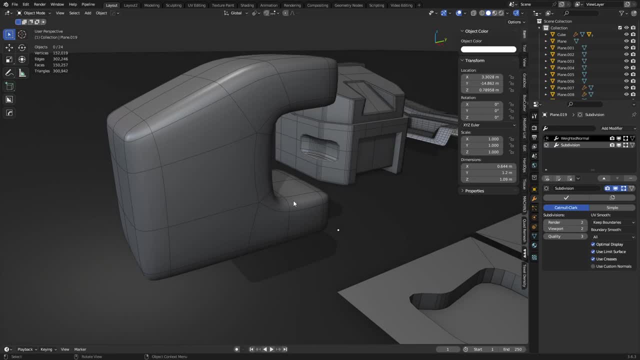 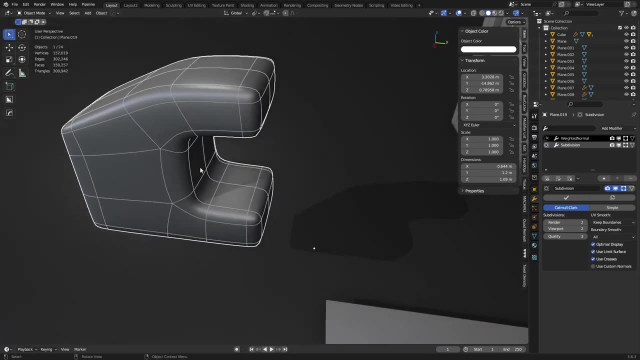 soft plastics or rubbery in nature. sometimes that actually looks good. or if you're trying to do stylized assets, maybe for uh film or whatever, you can get away with an old, away with those chamfers like that, and it actually makes things look a little bit more soft and 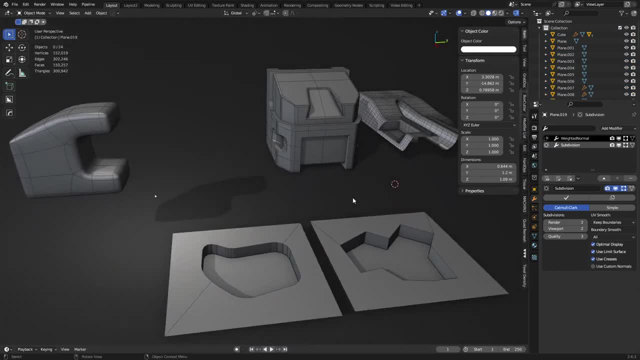 squishy, and you know they just work out a little bit better in some situations than doing the hard edges with three, three edges anyways. normally you need three edges to hold a, a sharp corner anyway, so that's what i'm getting at. instead, we're using two on that one. 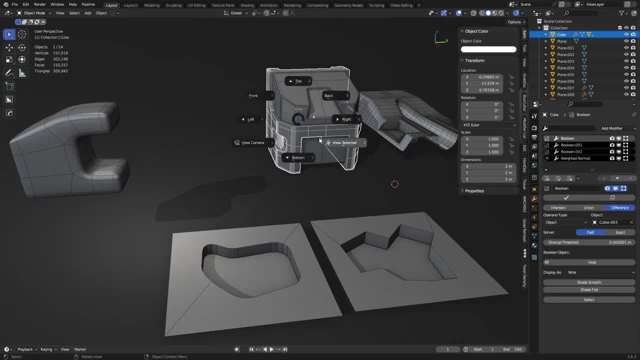 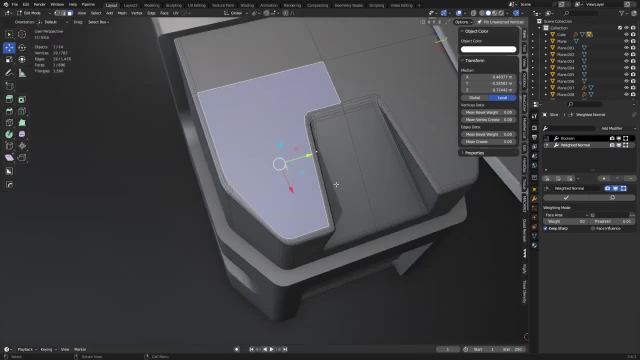 so over here i got a bullion ingon model that i had quickly tossed together, and so bullion ingons workflow. a lot of times you're using- you know- bullions, of course, but making big shapes and you're just cutting into them with the bullion. 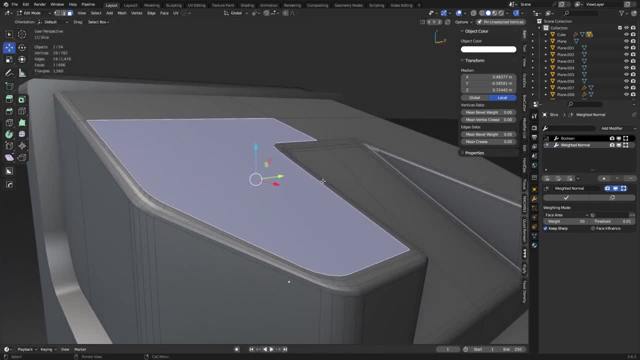 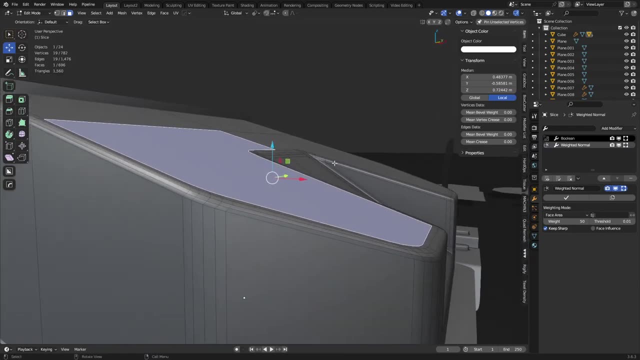 modifier. modifier. now you can use bull tools or box cutter add-ons like: uh, like those bull tools comes with blender box cutter. you got to buy. it's a purchase that or purchase add-on so, but you can see how this is behaving. we got these big ingons here. sometimes you have to support these things. 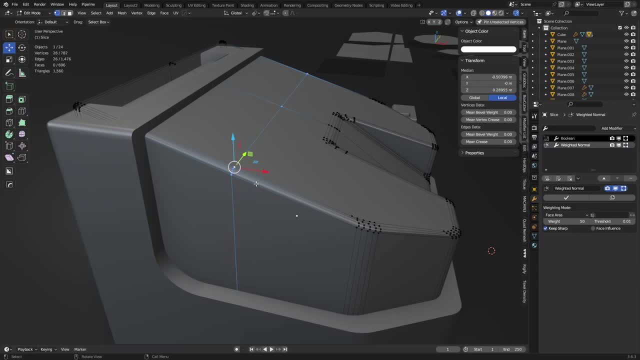 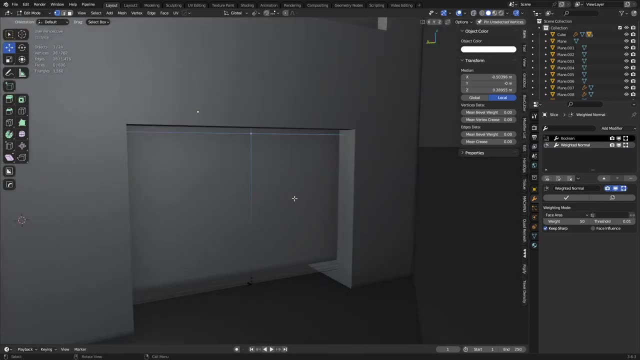 to keep the shading good and you might have to add additional loop cuts here or there across model or just knife cuts even because the edge flows here tend to die off quite a lot. you know you don't have like a continuous loop going around the whole model always, and so you know that's what. 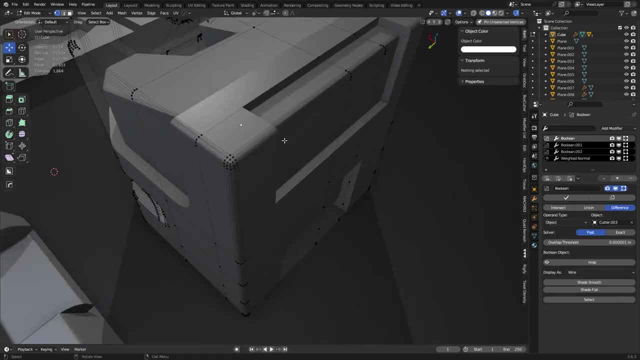 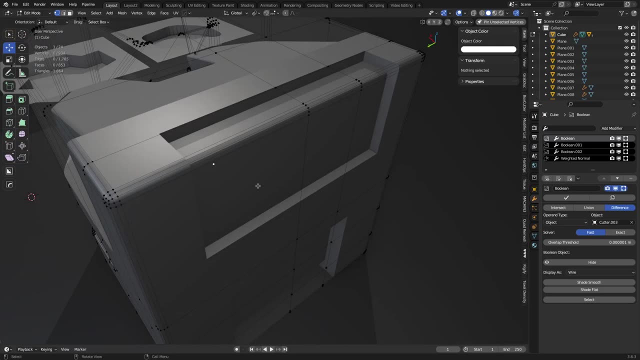 you're going to end up running into with with this workflow. now you'll get used to it, but it's basically you know, when you understand how edge flow works and you understand how to do loops, you'll understand how these are working as well. right like where they would you know. 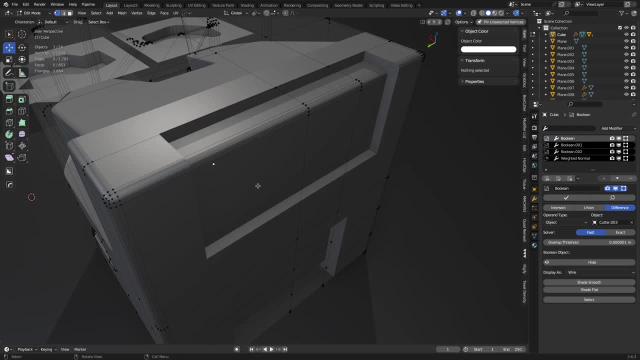 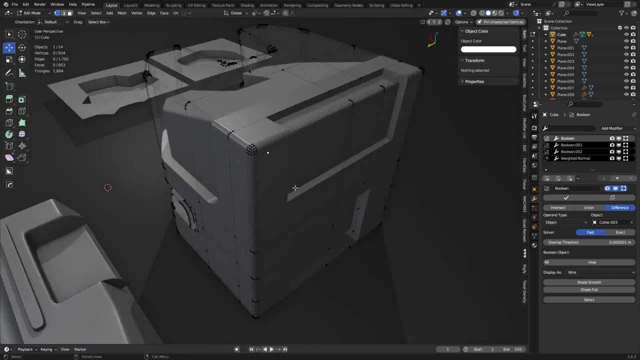 where they're supposed to come back around the model. they won't actually be able to do that, or they won't do that so, but they are placed in kind of the same positions as you would normally work with a subdivision model, so it's kind of kind of a um. it's basically similar, just. 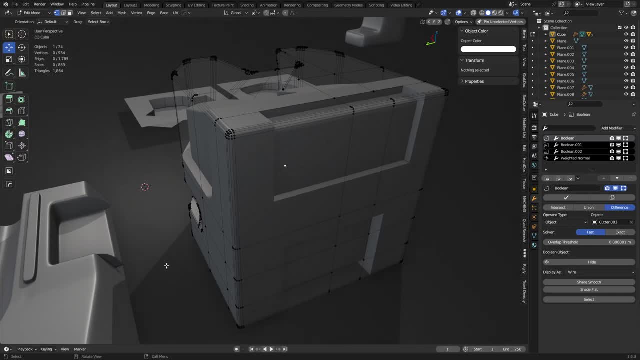 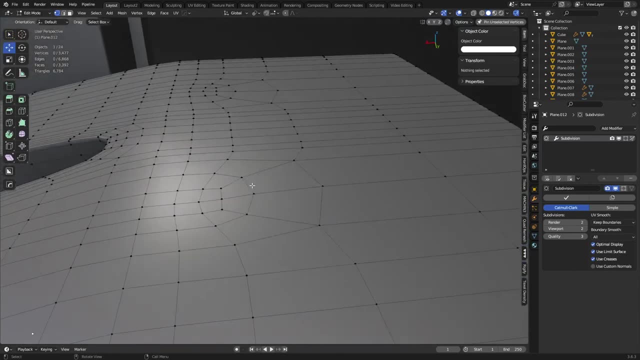 want to do that, whereas subdivision of course you know you run every edge and these do take a lot longer to set up and sometimes you can see when you don't have good topology perhaps, or it doesn't really matter if it shades correctly. you know, in this case we got a little bit of an error here, but 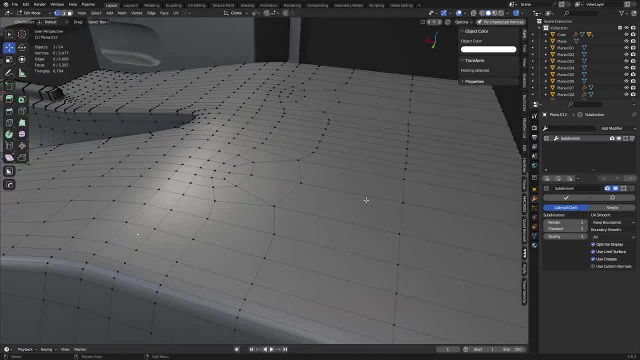 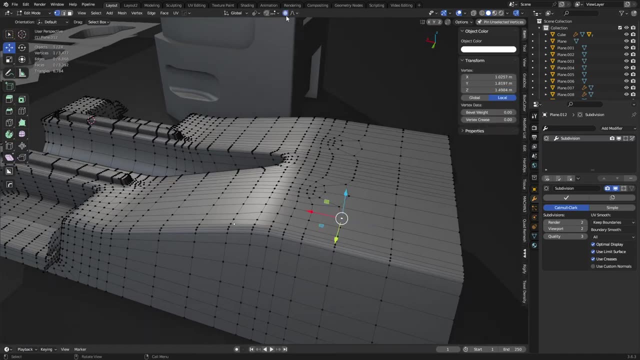 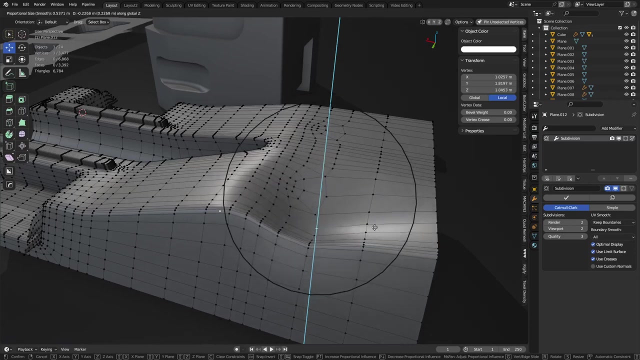 if it's shading correctly. in that area it's going to be a little bit more difficult to do that. so you can kind of check things with um by using the uh proportional edit tool. or you can use like a bin modifier if you're trying to deform your meshes. just give them a little test by seeing if they. 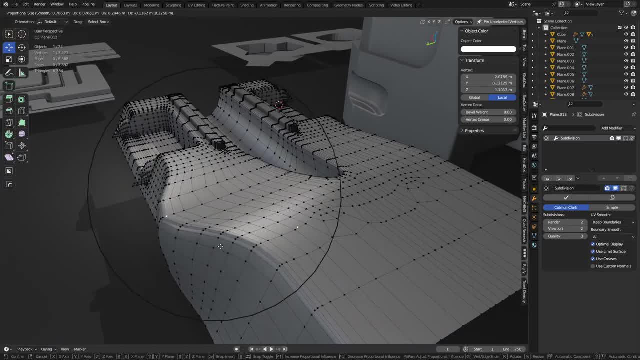 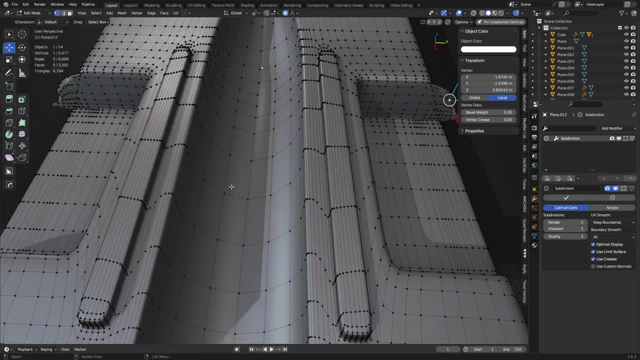 kind of behave the way you expect them to by doing the deformations this way, and so subdivision is not as limited as you think. you can see that's actually a big error, but, um, it's not as limited as you think, because if you set up a subdivision model and you're trying to do something like this, 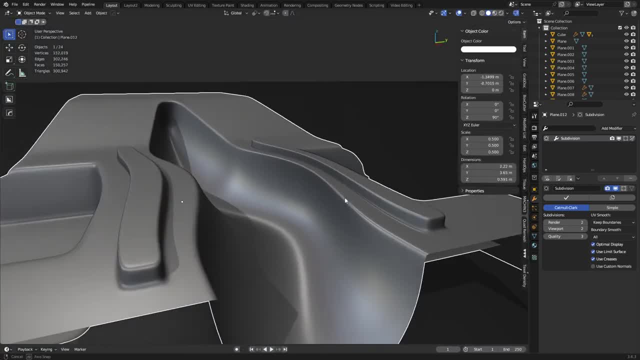 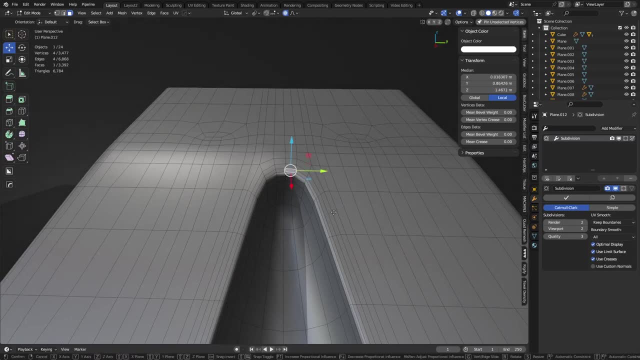 if you set up good quads, you can deform your mesh very easily- usually right, and so you can see what's going on here. when they're nice and perfect quads, it works well. but if you have something like this going on, it might still deform, but it's just um. it might give you different shading results. 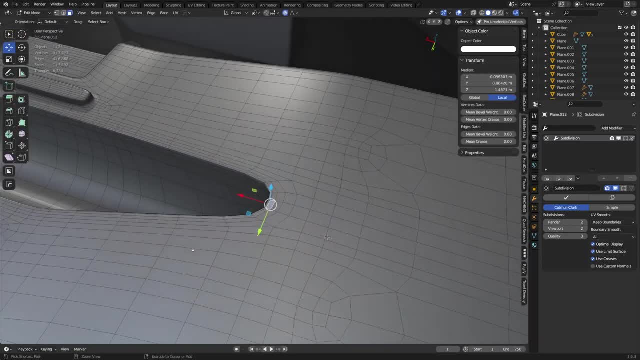 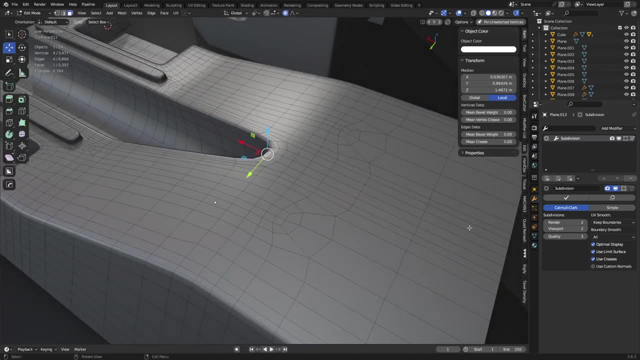 that don't look that good. that's what you're looking for. that's technically bad topology if you're trying to do deformable mesh right now. of course, what i had going on up here is i was just doing a reduction and i had applied a subdivision, so we don't see the original topology. 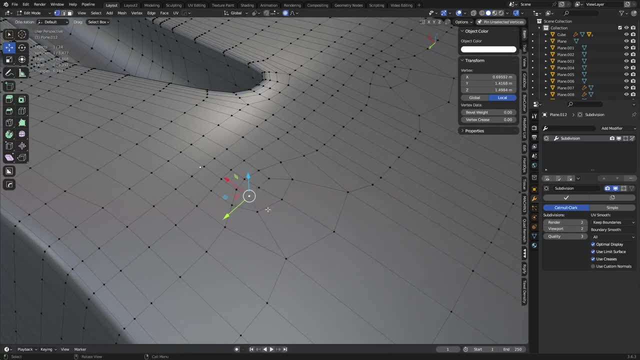 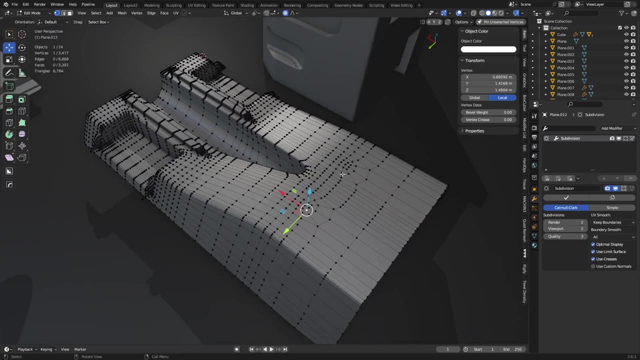 no more. but you can see here that we have the quads with the end pole. so this was basically doing an inset in this area or three to one reduction so you can see how that can kind of geek up your topology across the whole model possibly. so sometimes you have to be really 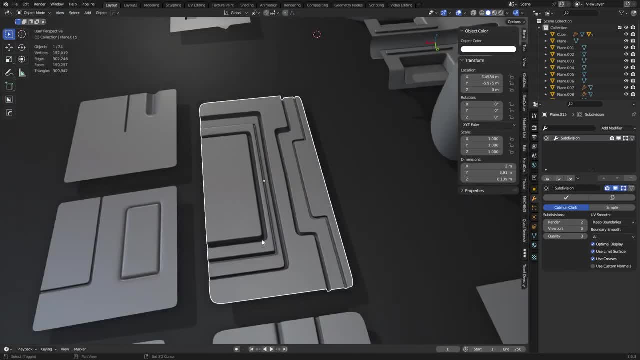 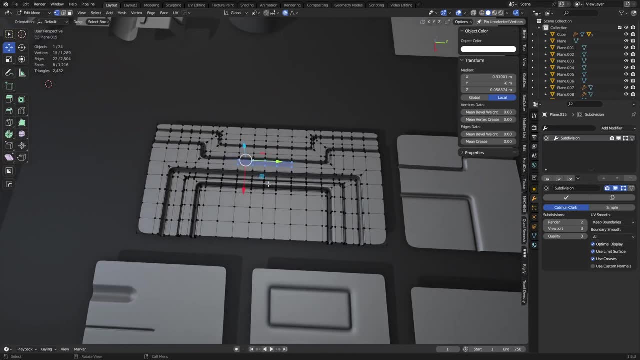 clever with how you're going to lay it all out and how you're going to work with it. this example we did earlier. you know it's very simple in nature. if you were to go ahead and keep working on that and mirror it across the center and create a little mirrored effect here. it's this complicated. 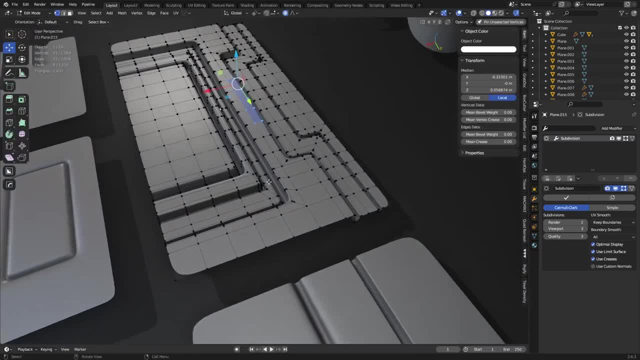 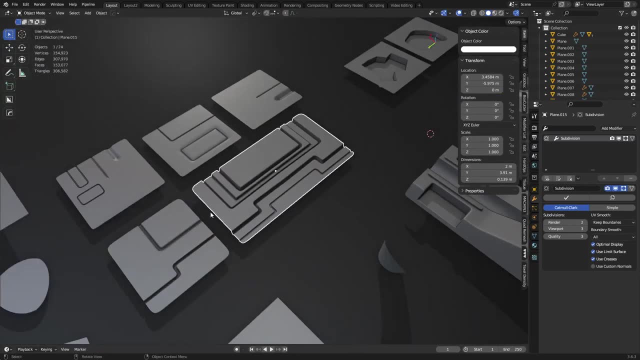 looking thing was basically this shape like. it's only a little bit further worked, it's not that much- and you can see it starts to look pretty nice. when you do this and you take your time with it and you have a little bit of fun. create some nice trim sheet effects or textures for environments. 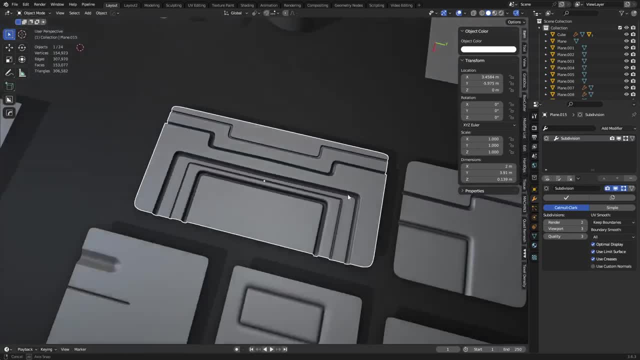 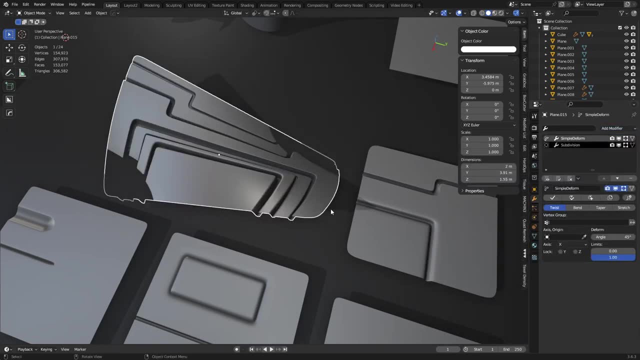 and things like that, if you needed to. or a hard surface detail, because even something like this, you know you could add a um, you could add a simple deform modifier and we'll put that at the top here. and for this particular one, we're going to do a bend and you'll see it: bends, all kinds of weird. 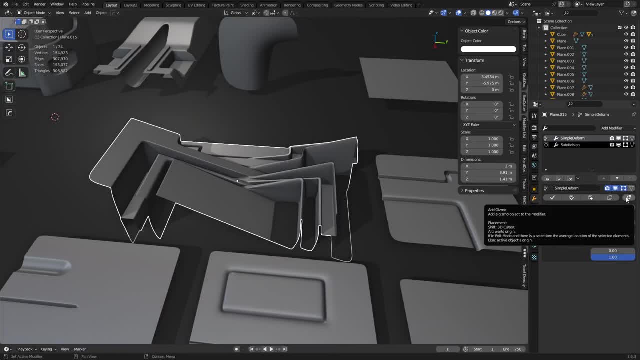 ways this add-on is going to be a little bit more complicated because it's going to be a little bit more adding on a little bit of initiative. we're going to do this here. you can see, click all really quickly and you'll see this add-on is called the modifier list add-on. you can create an empty with. 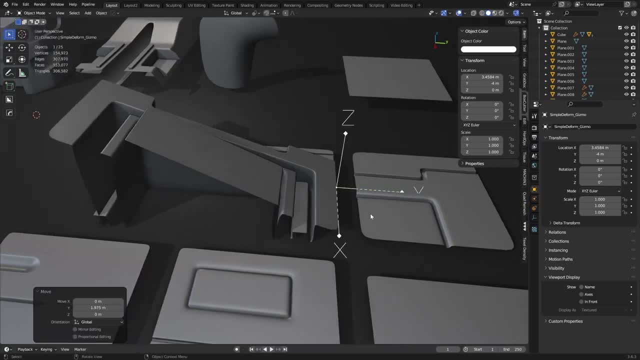 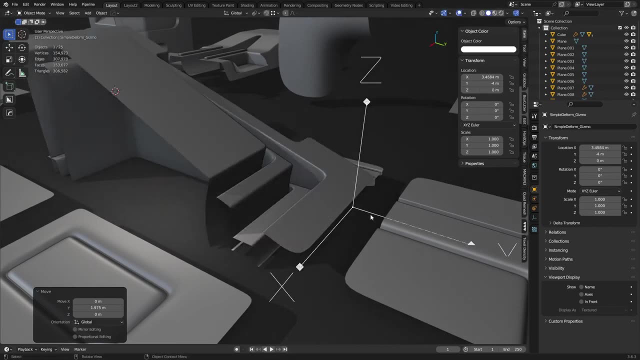 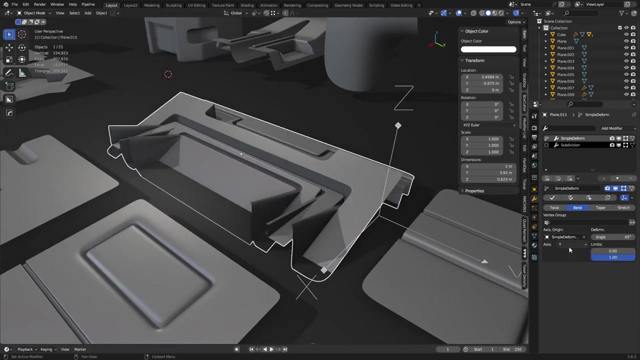 it real quick and it references the empty here. so all i have to do is pull this off to the side. perhaps I'm going to hold control and snap it real quick. i can actually snap it to the vertex, maybe right here. sometimes that works, sometimes it doesn't, but we'll get it close to the end there. 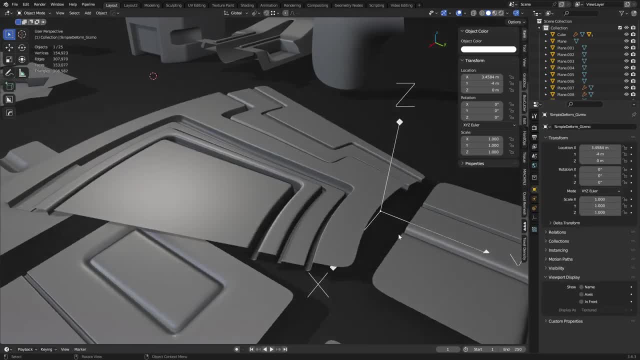 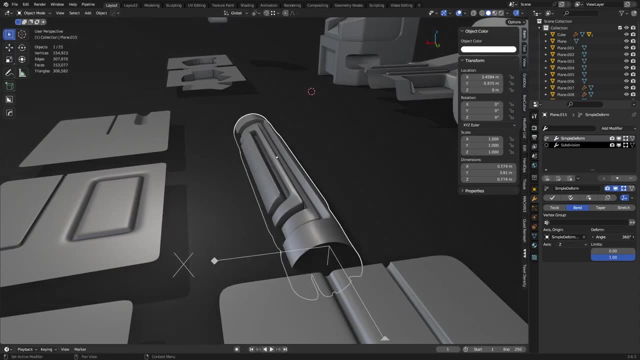 and what we can do is we can change the direction. now see if any of these are working. sometimes it Rotate it on X negative 90. perhaps You can see now it's bending in this direction. So that's cool. You could bend it up in that manner. 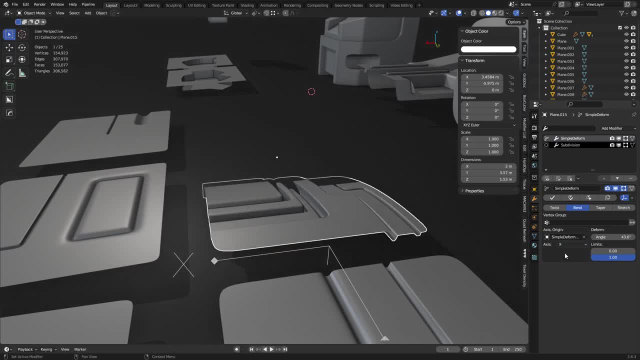 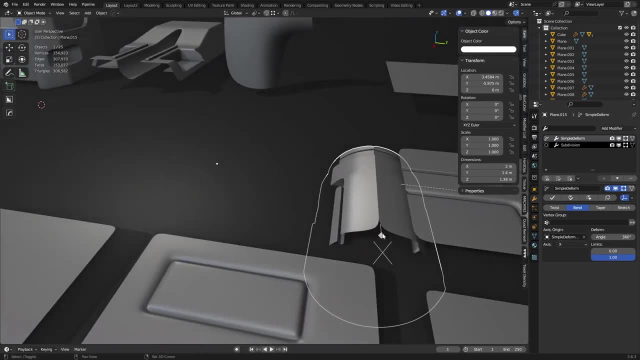 But we could also maybe bend it up on one of these other ones. So we'll do X And we'll bend here and wrap it around into the shape of a cylinder, So we can do things like this. I'm going to move it all, the empty and the shape. 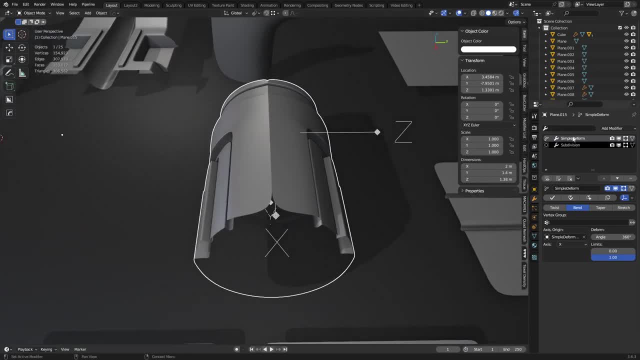 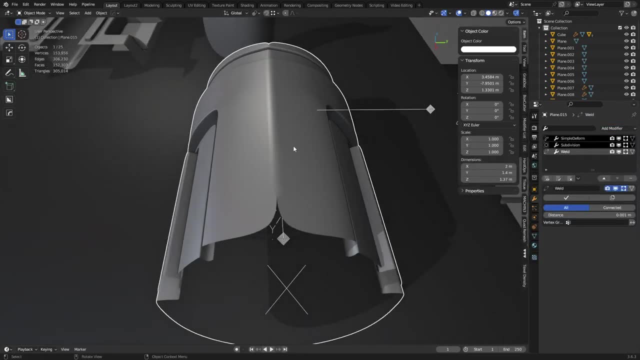 And you'll see there's this nice split here. So, after the simple deform, you add a weighted or, excuse me, add a weld modifier. You can see it welds it back together. Put this weld before the subdivision And there we go. 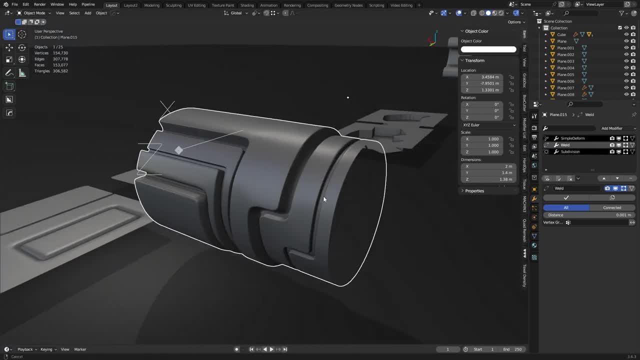 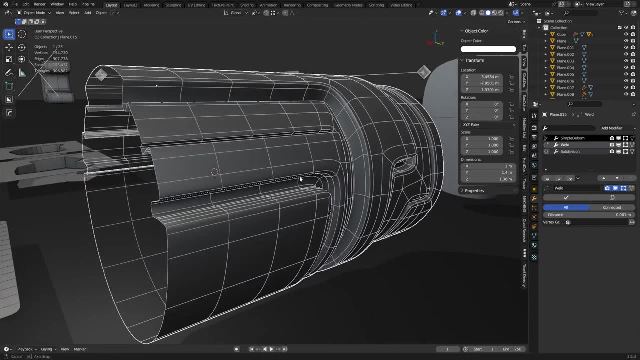 Closes it up, It looks good And it's all pretty much non-destructive. Well, the bending of it's non-destructive, at least So semi non-destructive, But the base shape there when you create nice, even topology where it's mostly all quads. 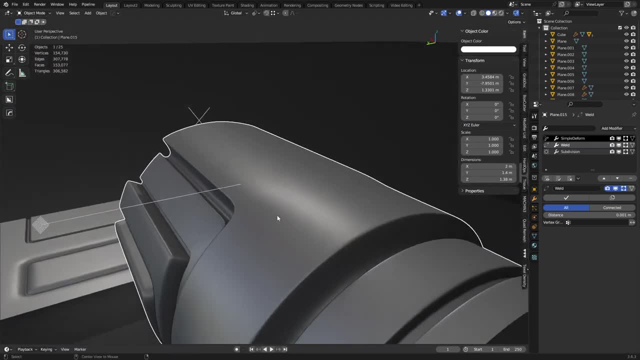 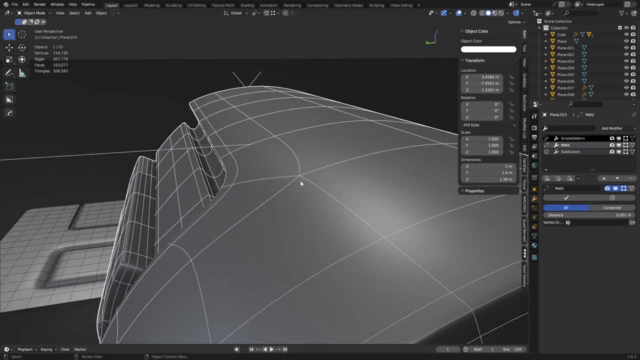 it has good edge flows And you can sometimes get away with E-pulls on curves. Usually- You know this- This is a E-pulls, and N-pulls on curvy shapes can cause problems, right, But in some situations they work out just fine. 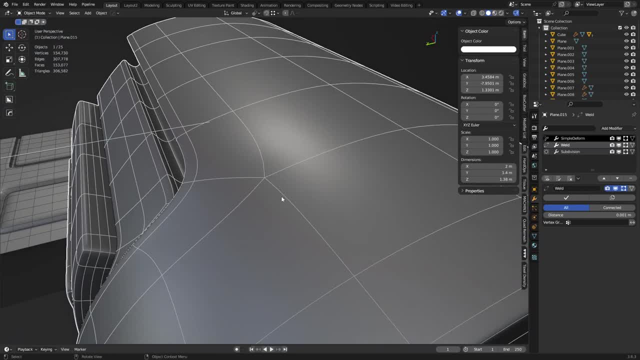 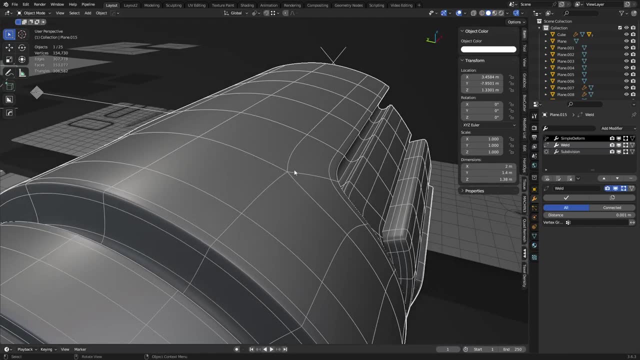 And you'll have to kind of figure out how to go about doing that. That's going to be one of your most challenging. things you'll end up doing is trying to learn how to work on cylindrical shapes and spherical shapes and using E-pulls and N-pulls. at the 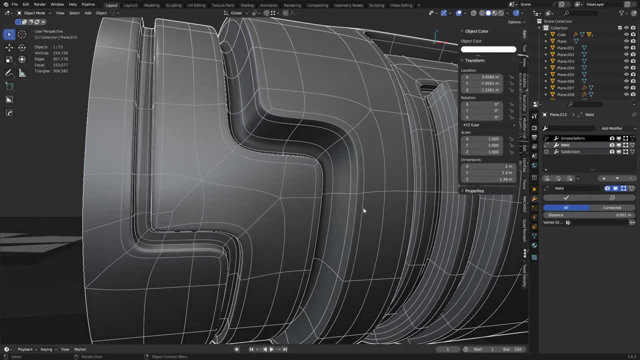 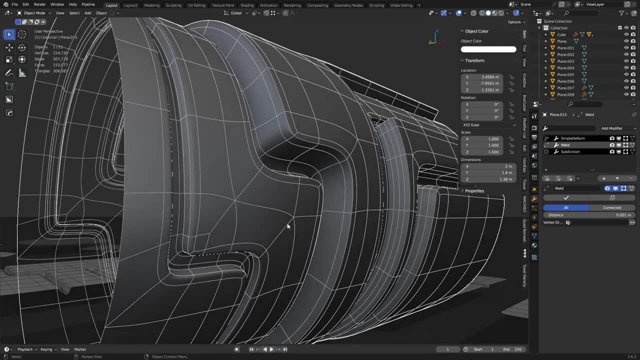 same time, But this is just a good example of that. You can see when we use that simple deform, all of these are being pushed out into the correct spot. It was a cylinder, Whereas if we were modeling on a cylinder, we probably would have a hard time matching. 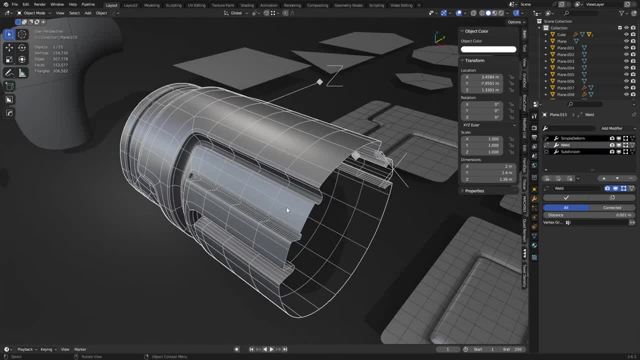 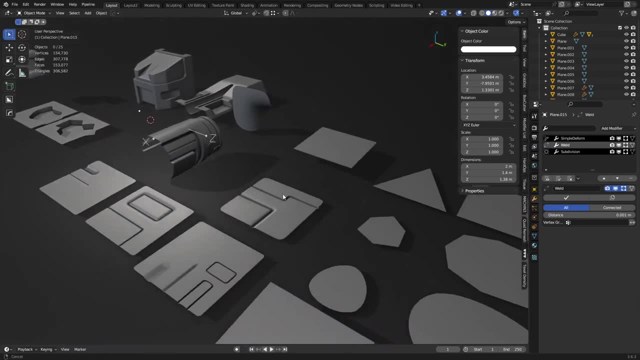 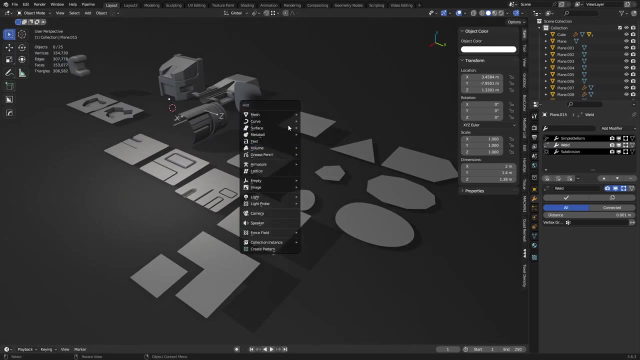 that. So this is an excellent technique that you could utilize to get pretty good results here. So this is one that is commonly used in game art especially So, and I'm sure any other type of 3d modeling as well, but overall, let's just make one shape. 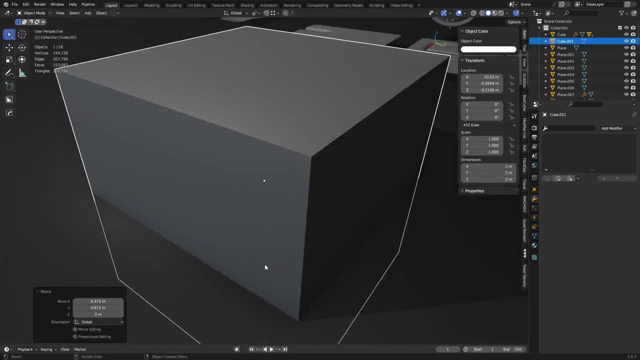 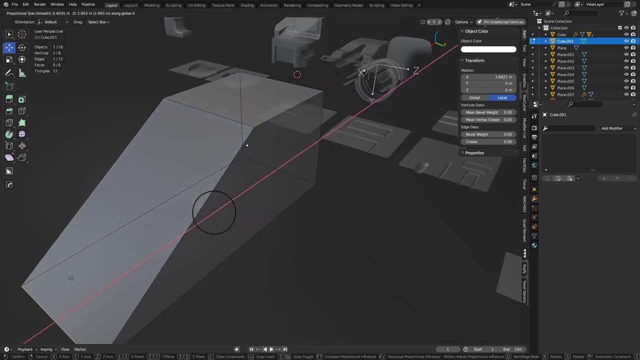 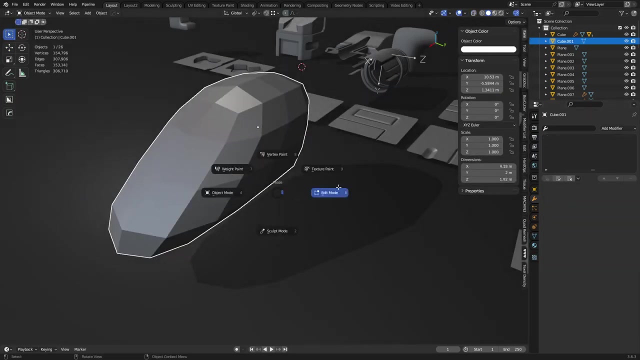 real quick. That first one was kind of a little bit rough, but let's just do one more shape And see if I can't add some loop cuts in here. most subdivide at one time. apply that Okay, And so we have this shape going on now. 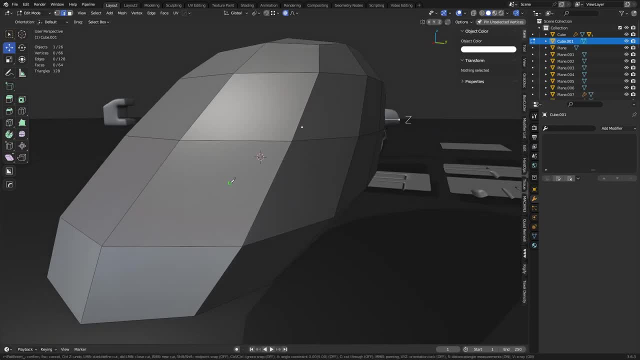 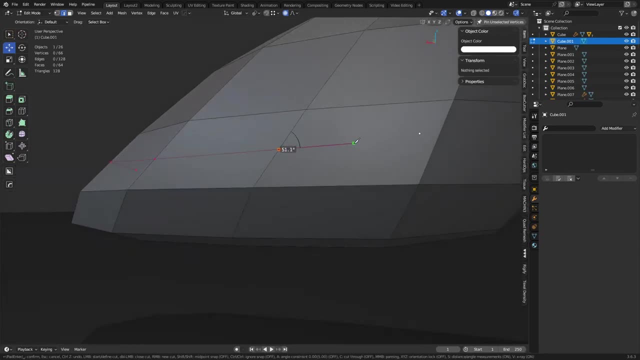 So let's say we wanted a scene going around this thing, just like we did the cylinder there We can cut wherever we need to go. We want to do an N-pull, We can do that and we can send this down below it. 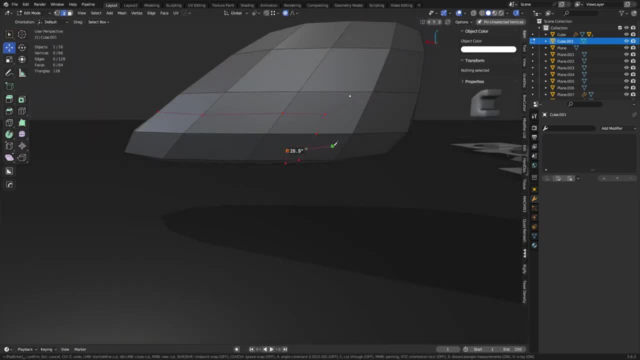 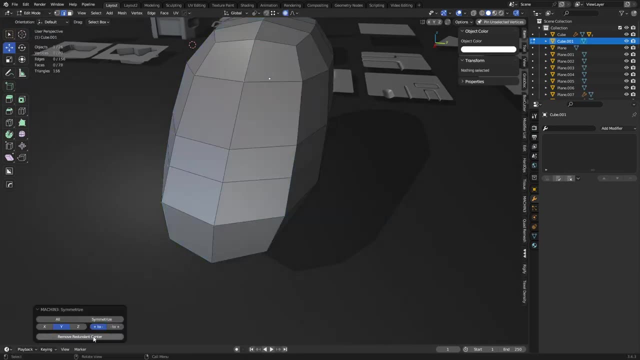 We can do that and we can send this down below it. Okay, Go across the symmetry And what it'll do is, eventually, when we add that mirror, I'm going to symmetrize with mesh machine add-on and then turn, remove redundant center off. 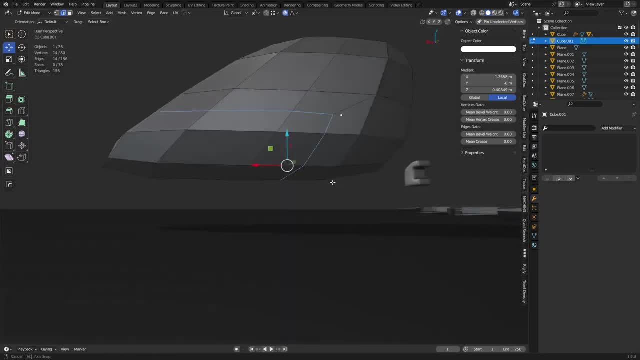 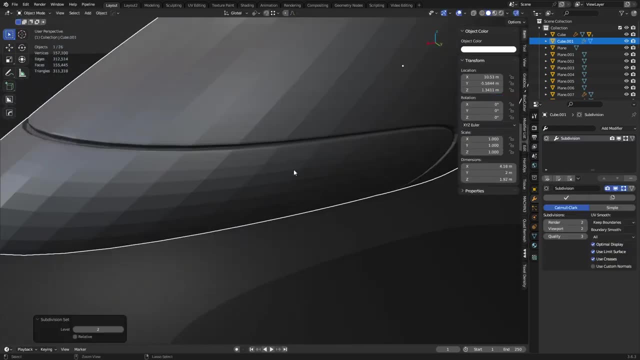 So we have an edge now, going exactly where we want it. We can turn this into guess it: hit control B, inset, inset, hold, control bam. So when we subdivide this again, we get this result, All right. 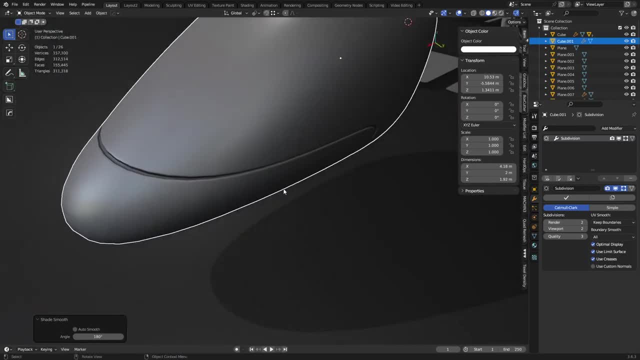 This is something you might want to do at some point on your 3d models. It's going to be up to you. It's going to be a judgment call Now. this is just one way you could have went about doing it. 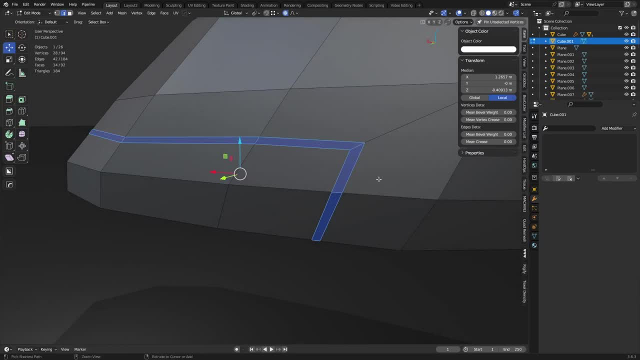 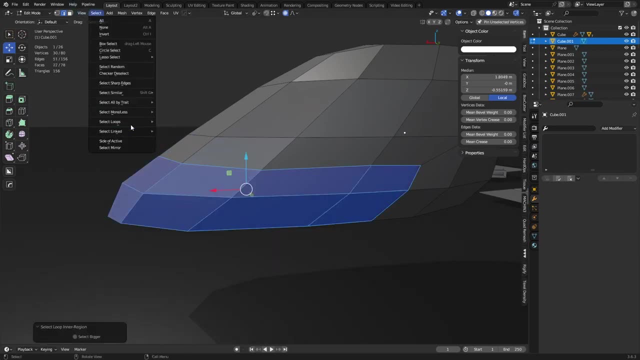 You could actually do the inset like that, but you could also maybe do just the edge here, possibly, And you select everything in one side. So you do selection methods, loops, edge loops, rings- These are all useful: Loop inner region and loop boundary loop. 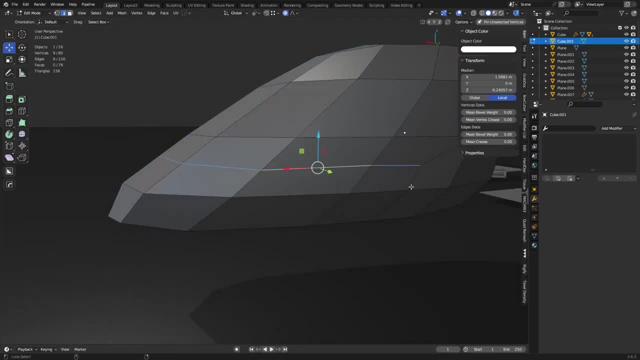 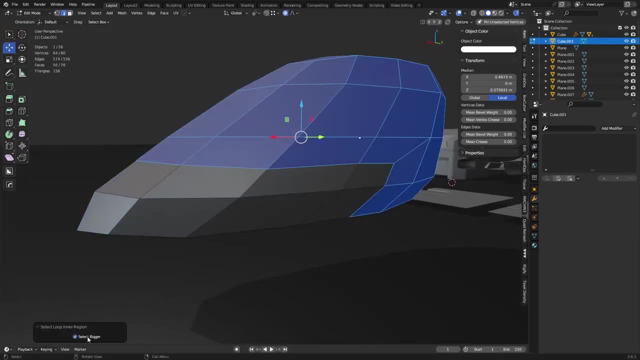 What I just did was the loop inner region. So you can select a set of edges like so right, And now you do loop inner region And then Now you got that If you want to switch it, you can go to the other side there. 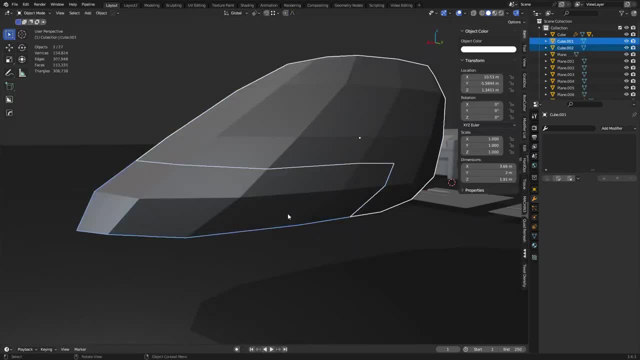 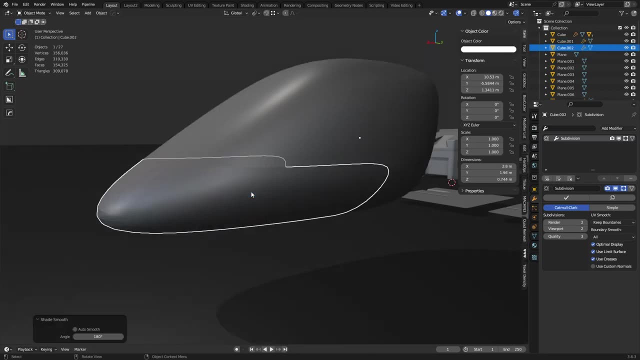 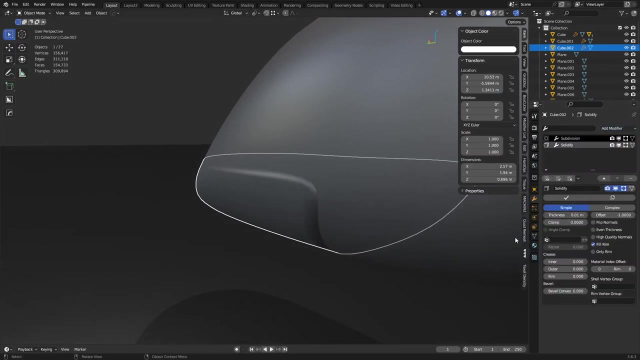 So that one's really useful. but we can separate that perhaps at some point. If the subdivisions match here and the vertices match each other, we'll have a really clean uh meet up between these two shapes, Right? So later on we could do something like add a solidify modifier and we might 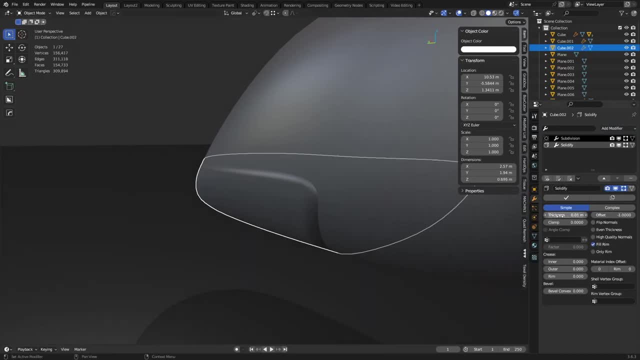 be able to push that out a little bit, If I can get it to work. I guess it's not going to work for some reason. Let's do it before the sub Division, All right. So if we push that out, I'm going to copy the value here and we do another: solidify. 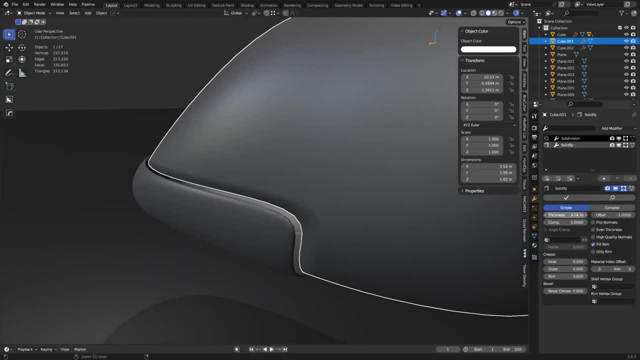 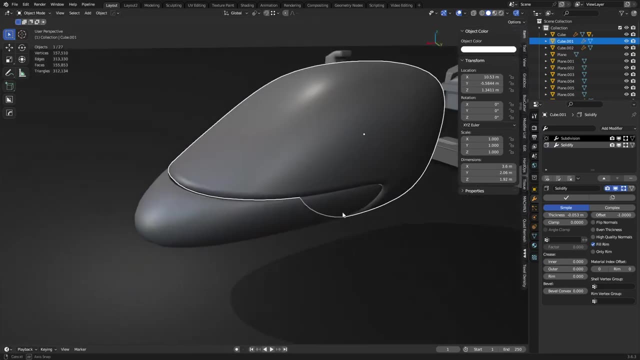 modifier and we can paste that value. So control C and control V as you hover over a field. So control C copies, control V will pace All right And the subdivisions kind of curl in the edges. here A couple of ideas on how you can deal with that. 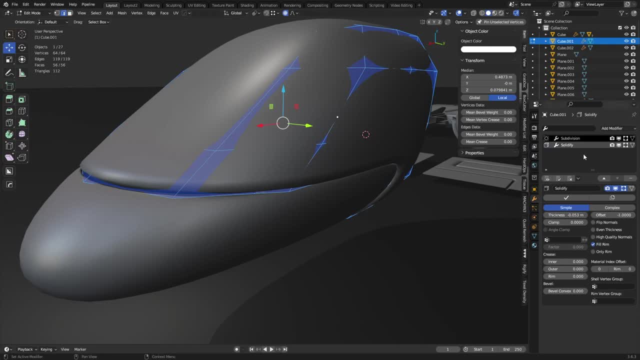 You could try using a weighted bevels, which is a level modifier with weights applied to it, which I'll make another video on later. But there's also creases possibly, So you can do something like select loops, uh, boundary loops, and you can. 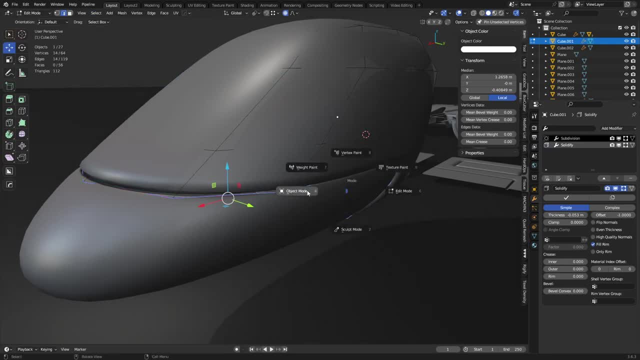 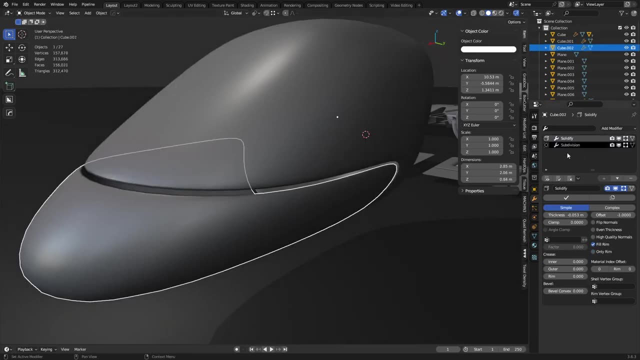 maybe add creases to that whole thing, And sometimes that'll hold it in place as well. Um, a little bit better in this case. a lot of times you're going to end up having to use the solidify, So you put solidify before subdivision. 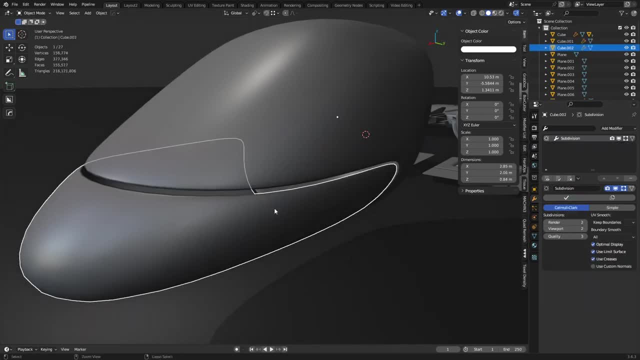 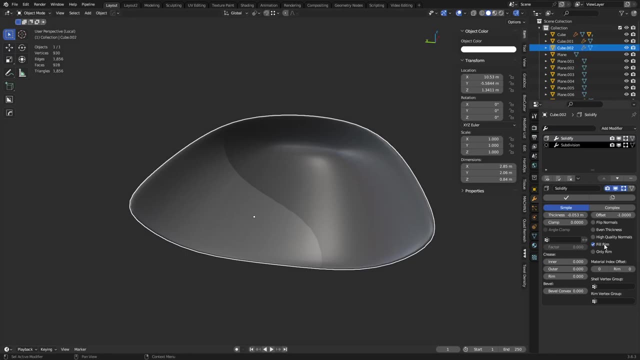 And then what you're going to do is you're just going to apply it later. Oh, side note: here It's forward, slash a second, isolate it. It has an interior side. Now, if you want the interior, you can keep that. 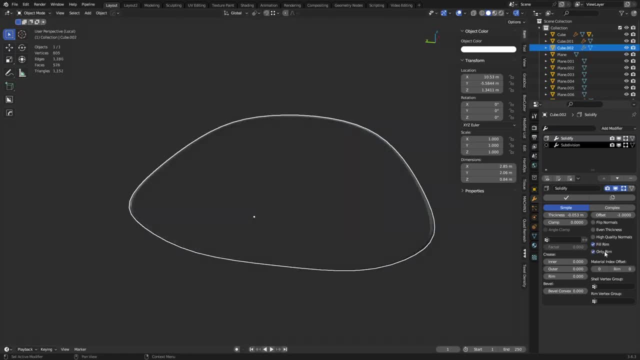 Um, but you don't necessarily have to have it. You can do only rim right, And so that also is useful if you want to keep it non manifold. Oh, a solid mesh, by the way, that's completely airtight, is a manifold mesh. 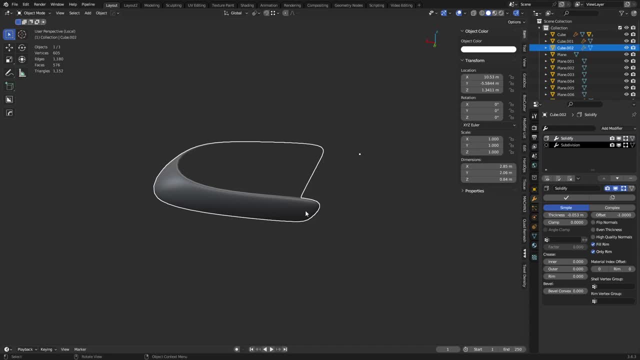 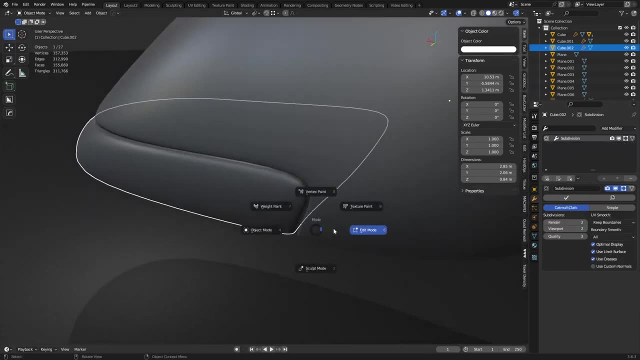 If it's got empty, uh, it's got spaces on the edges of it. It's a non manifold mesh, Okay. And so what ends up happening here is that once you apply that solidify, you could try adding loop cuts if you wanted to, but you'll have to make sure they 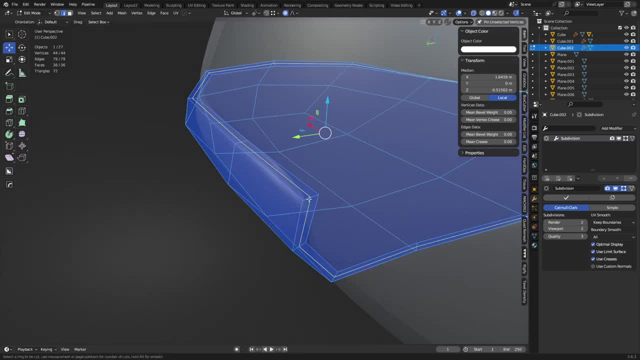 kind of match between the two meshes, Um, but if I just want this to be Sharper in this area, I could just add maybe a loop cut through here, and I might be able to do that as well, So we can apply that solidify. 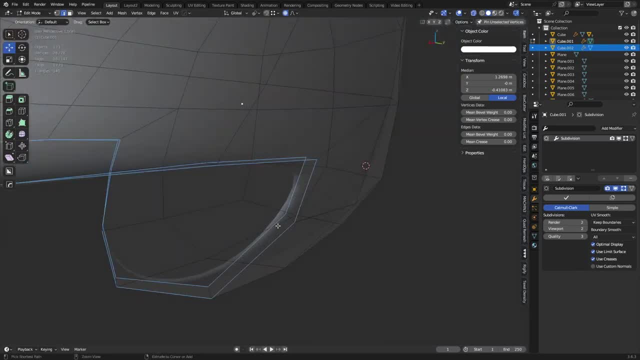 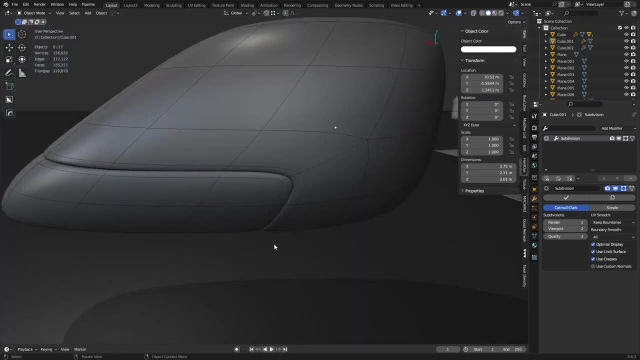 We'll do that on both sides, here And um. now we'll do this one, And that should just keep it a little bit sharper in that area If we could also try beveling the edge. that's another, another technique. but 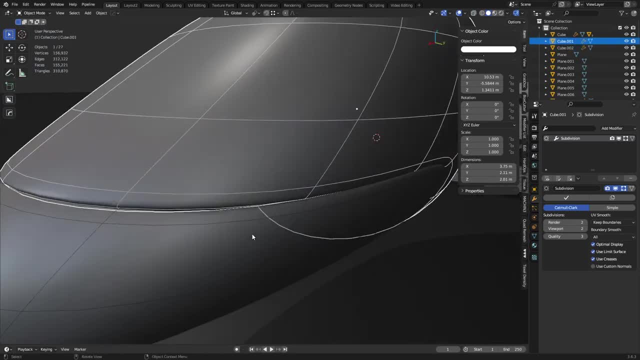 if we want to keep like a little bit of softness to it, just adding that additional loop cut uh should work out pretty well for you. You might end up with a little bit of a gap with this, though Sometimes that does occur. 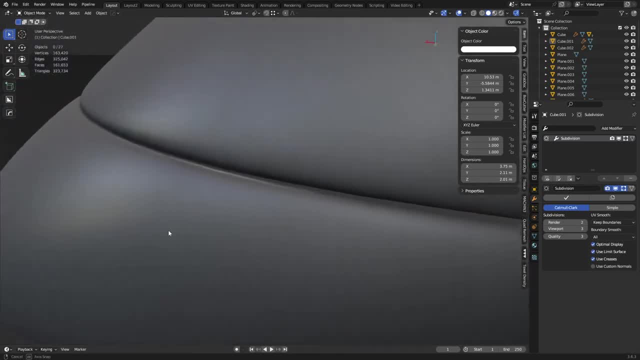 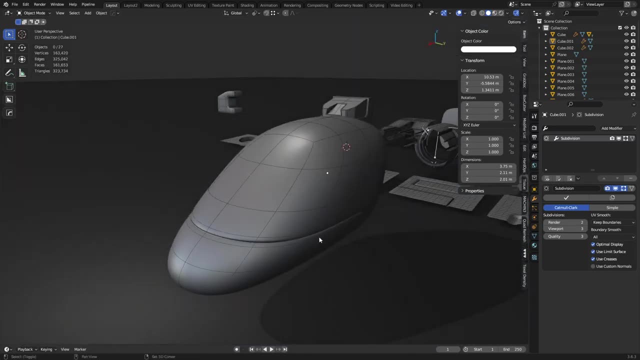 You might have To shift things around just ever so slightly, uh, to get that to go away, but you see, it's not too bad right now, So I think we can work with that one. It's all kinds of ways of creating panels and whatnot, but this is what. 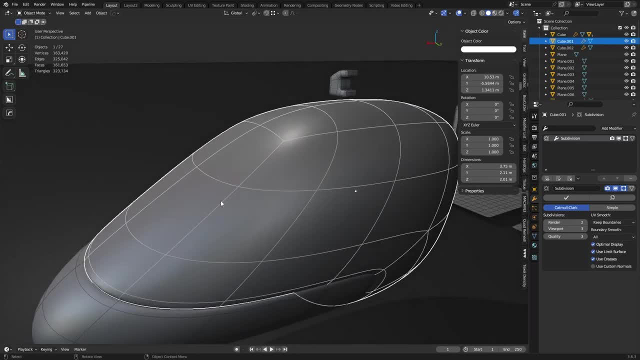 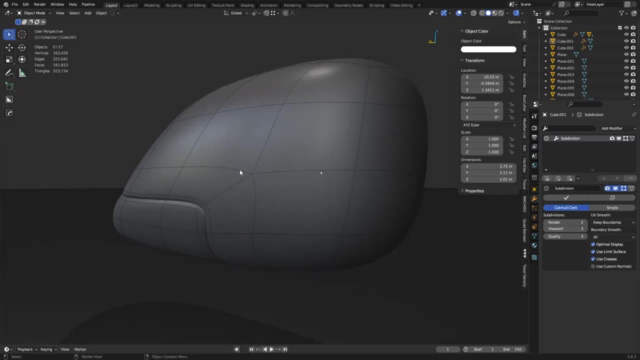 you're looking for, with good topology. You're looking to create nice, clean edges lines as simplified as possible. It's not always going to be possible, but the better- uh, your mom, the better you're at at doing this kind of work like this, this is going to be better for. 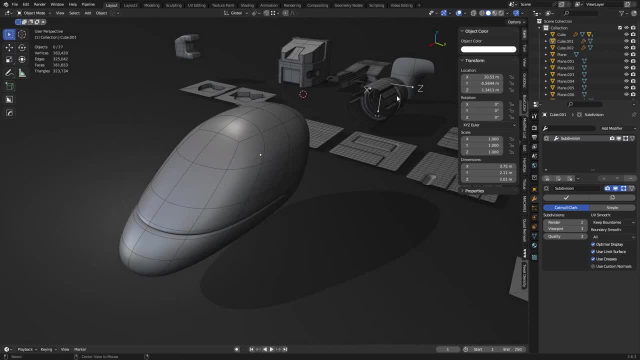 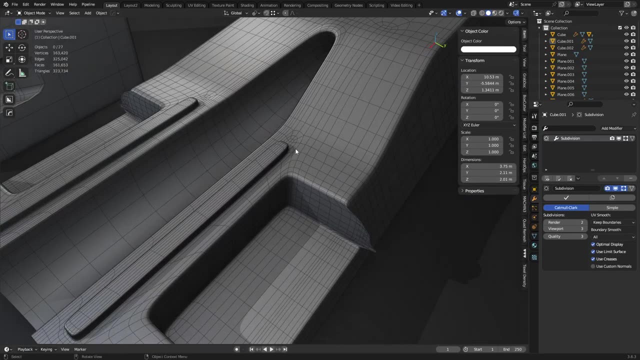 um, like your topology is going to be better over, Generally speaking. So practice creating really clean, nice meshes first, before you get into a bunch of chaotic messy stuff like this. This is something that is, um, you know well, it's. it's important to understand. 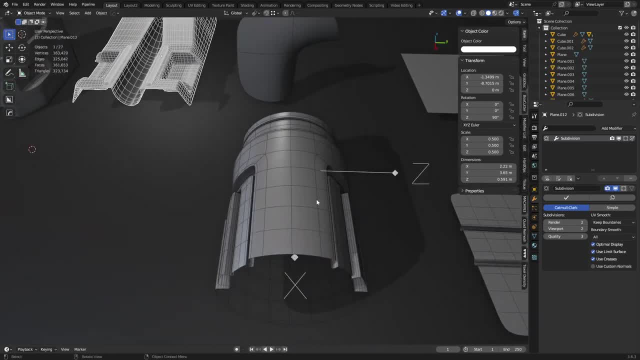 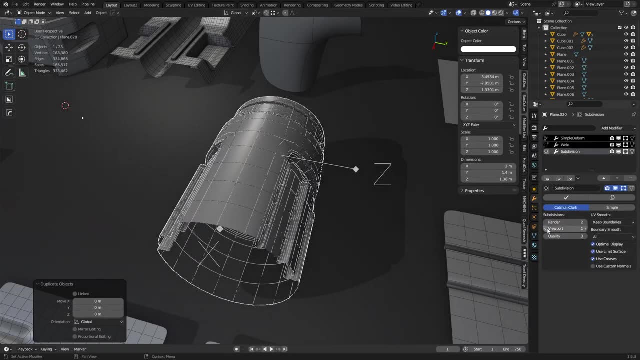 what to do when you start increasing detail on models and you start increasing the polygon counts, because a lot of these shapes later on you might take them And you might do like a level one subdivision on it. You might convert it to a mesh later. 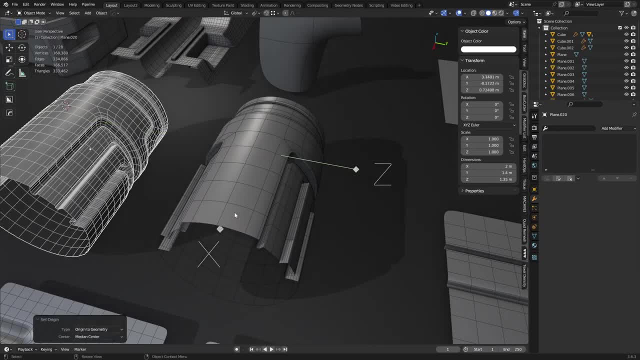 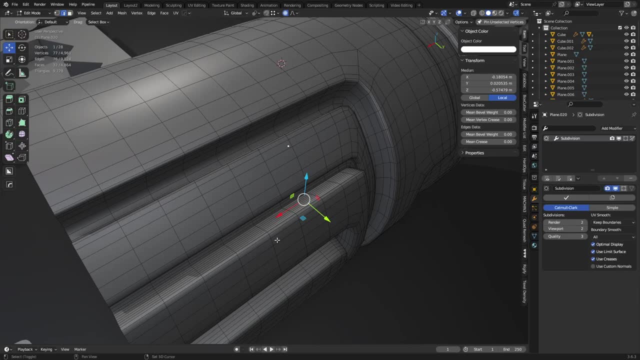 Right, And so now we have a more Yeah, Detailed mesh here, but it's the base topology that we once had as well, And so we can go in and start adding additional elements later when we want to do things like that. one little uh bevel. perhaps remember that a day. 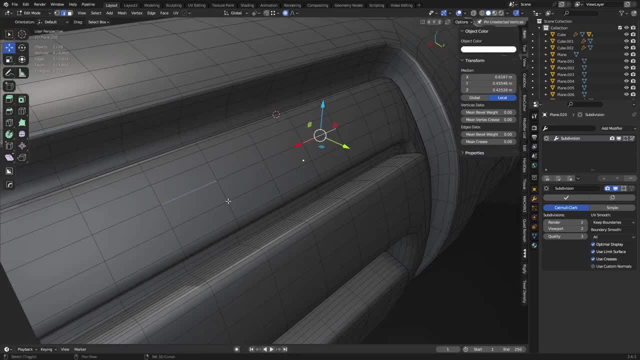 earlier. uh, so we might be able to get away with doing that in here, this area. They pull this portion of it off. They would pull that one in a little bit. We'll merge these two right here- Well, that went in a little bit- and then merge them. 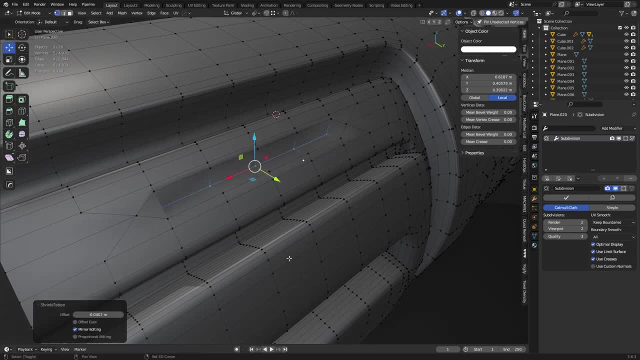 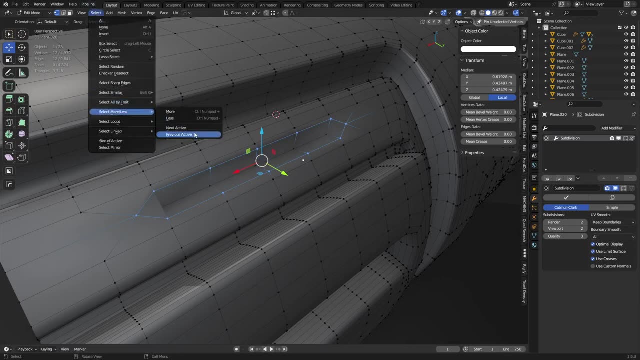 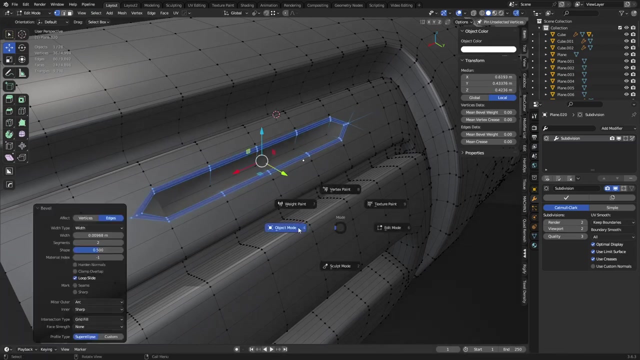 So loop cut all, S, select more control and we're pad plus to select more. Now we're doing the boundary loop, which have hot key select loops, boundary loop, And we can do a bevel here as well. Okay, And so when that subdivides again, now we can start adding additional. 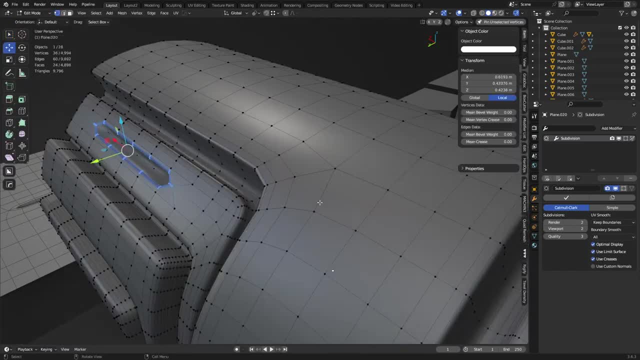 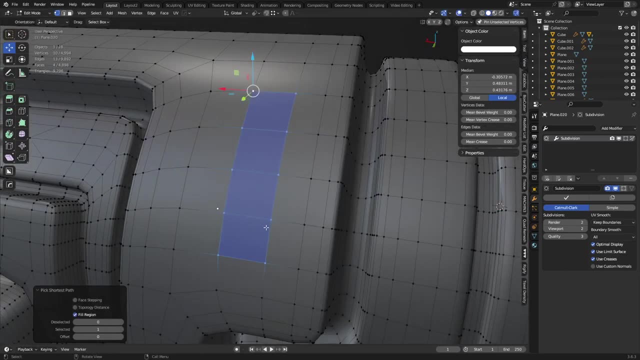 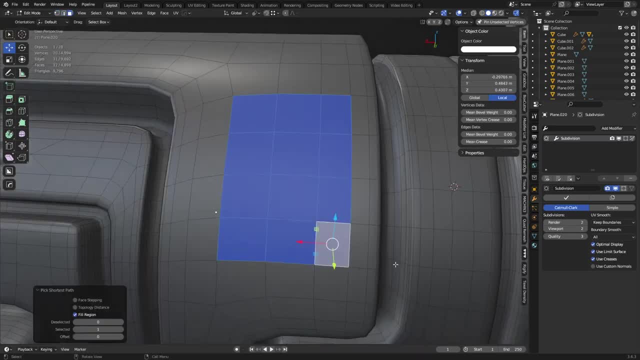 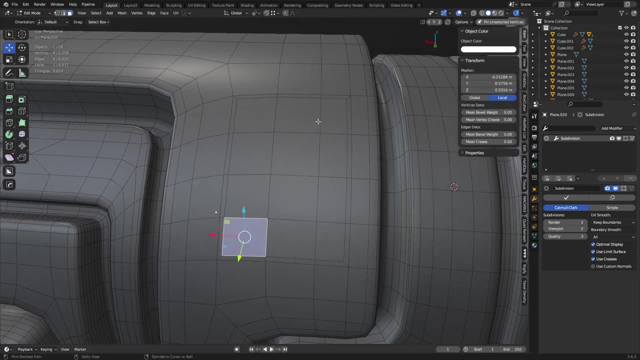 To support that as well. So if you wanted to do like a push in here, you really need to have two additional edges at minimum on the inside here And two on this axis as well, because if we start to do an inset when we insert, 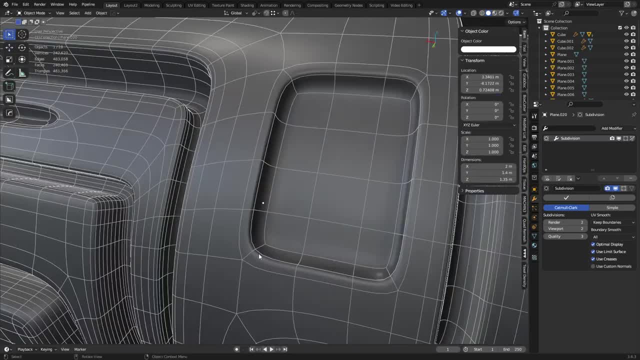 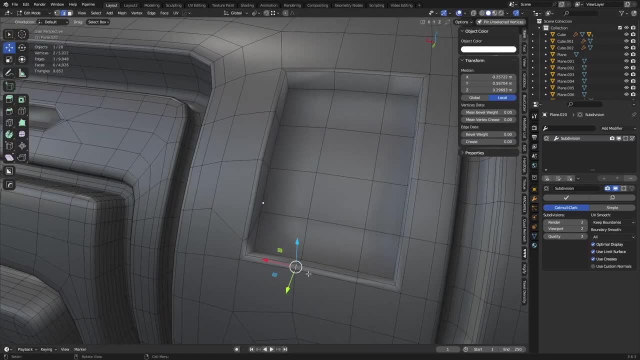 again and hold control. push that in. you'll see that these are going to round here And if you don't want these types of edges rounding out a lot of times, you're going to have to take these other edges and slam them over like this. 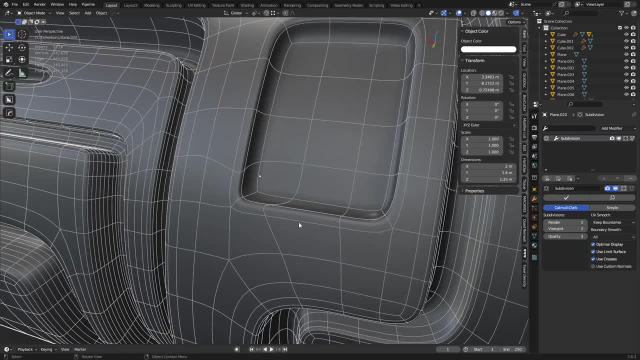 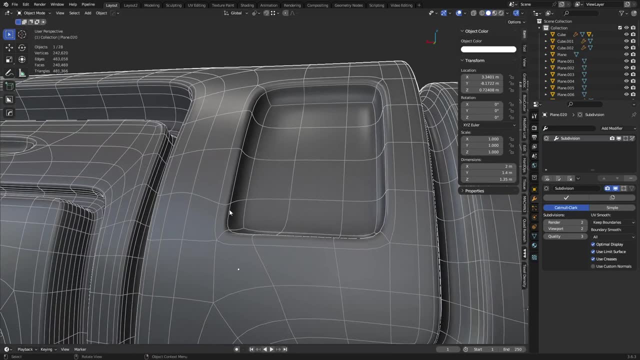 And so what ends up happening is you can tighten that bevel up. basically Now it will shift the topology A little bit, So it's technically getting a little bit flattened here now because of such a dramatic shift. So you want to do these at the right resolutions, right density. 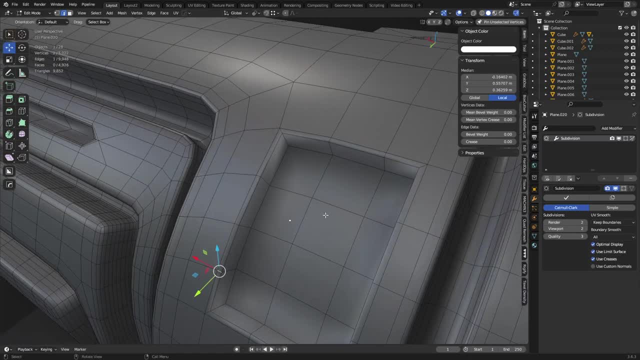 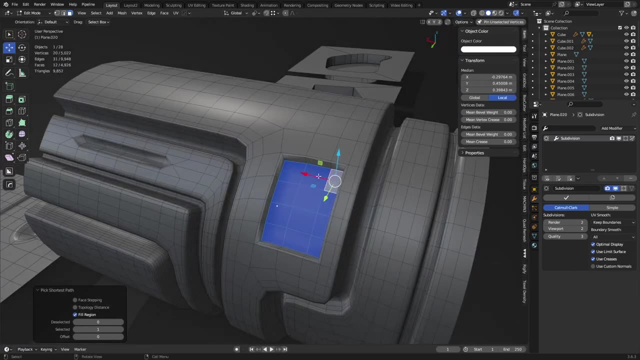 So that way you can utilize these kinds of edges to tighten up corners perhaps, And you want to make sure you push this in at the right density as well. Now our base mesh, our base geometry, there right, Is going to dictate um, our edge flows for the most part. 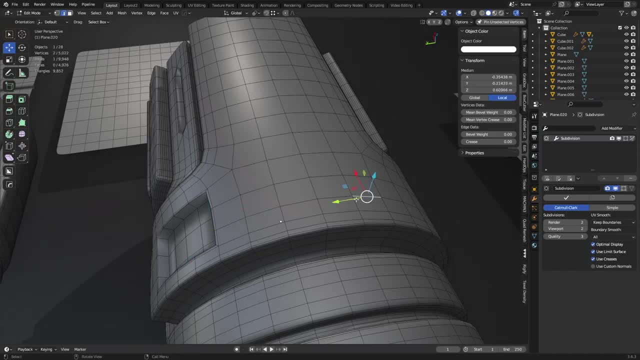 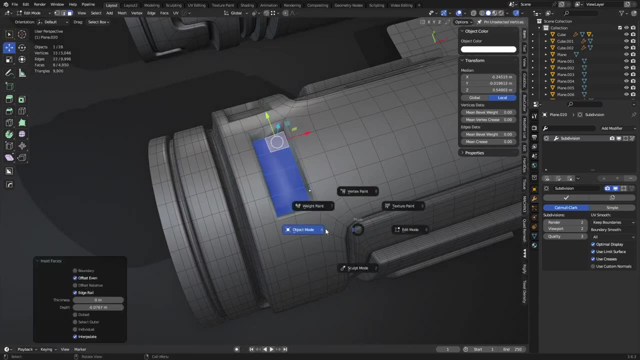 So if we don't want to do spend a bunch of, but we don't want to spend a bunch of time cleaning up edge flows later on, We get them right from the start. We won't have as many problems. We'll be able to go through and do the- uh, the additional edits that we need to. 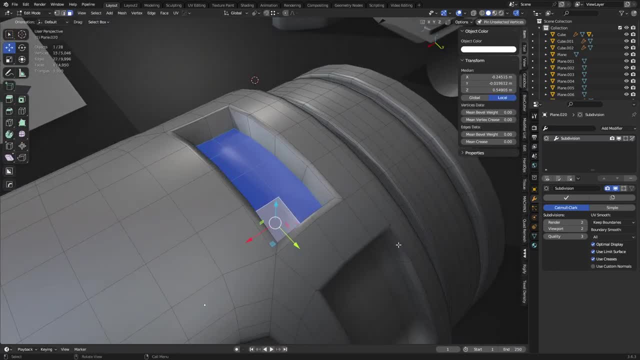 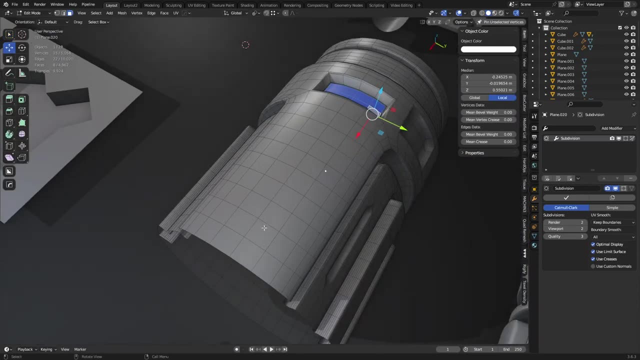 do so, we can start creating some really complicated looking stuff out of those base meshes, even if it's not really all that complicated, because it's just some more push-ins and whatnot. on a side note, you can always grab a set of quads like 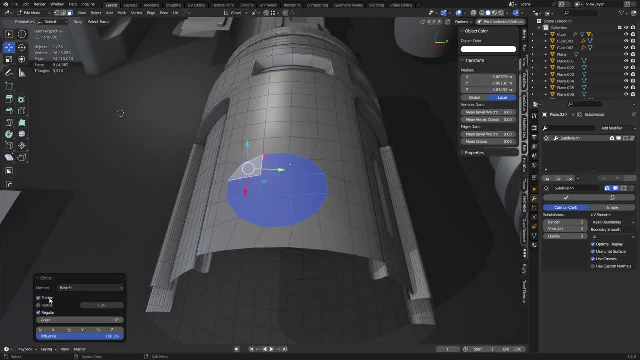 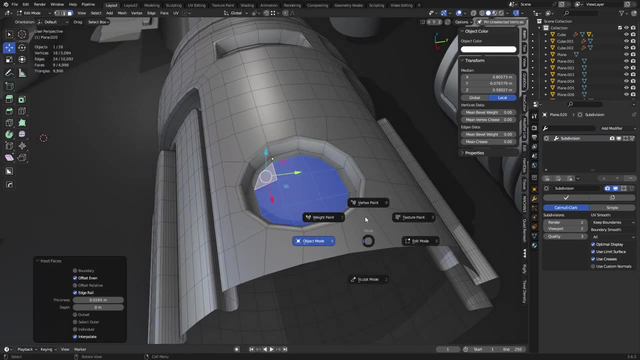 this and you can also do: loop tool circle. You could turn off, flatten, and a lot of times that'll try to preserve the shape here. It doesn't always get it right And we can inset, inset, hold, control and say again. we can also do. 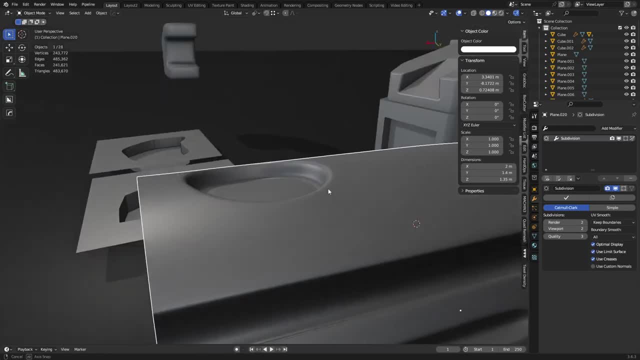 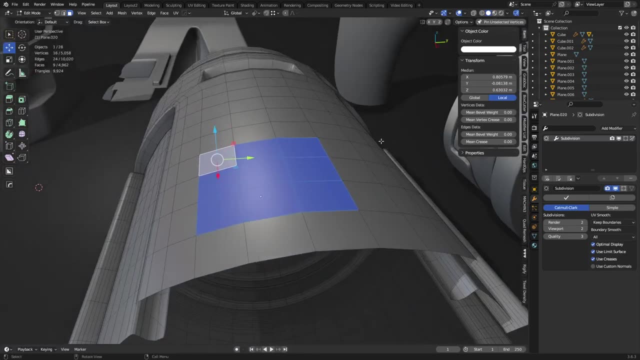 things like that possibly. Okay, That's just what the vanilla Okay Blender tools, But you can see it delivers a pretty reasonable result there. It's not big, not a big big deal. Uh, what I personally like to do, though, is I use the machine tools, add on. 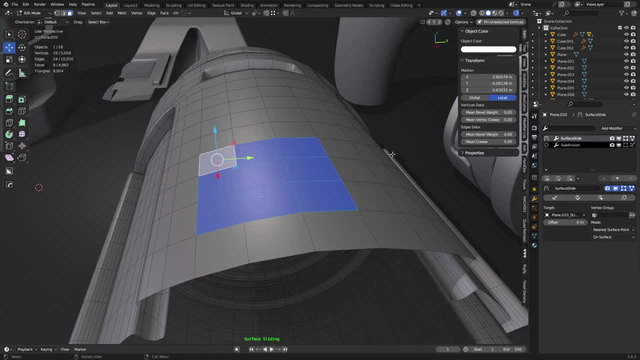 and I'll turn on surface slide. Okay, And this is like a temporary shrink wrap modifier. So then I can just go ahead and do loop tools in circle and even flatten it- It wouldn't matter, because it's shrink wrapping basically- And so if I do an inset or something like that, I can always add another circle to. 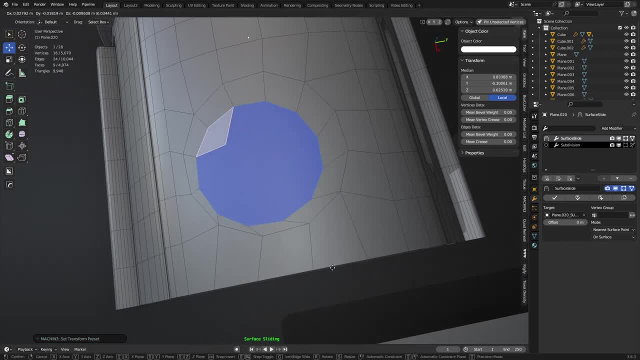 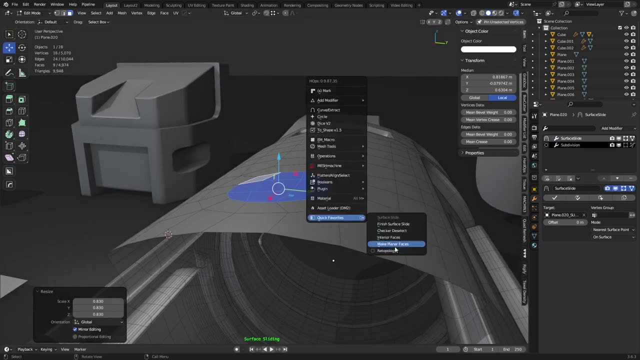 it. I can keep working this, I can rotate it and move it around and do all kinds of fun stuff here. Now it may distort the mesh A little bit, but you'll see here, Once I turn that surface, slide back off. okay. 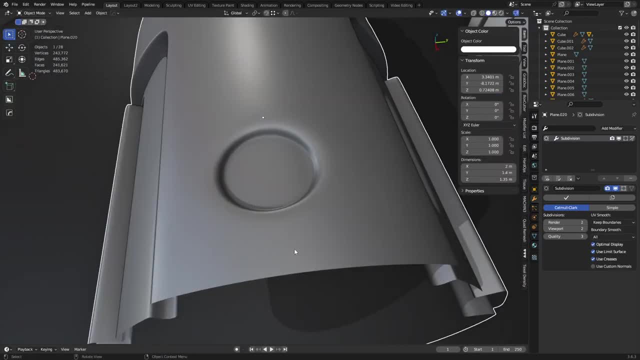 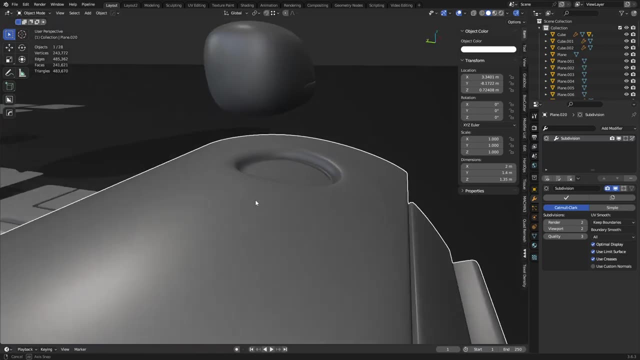 And I inset that whole control and setting in. uh, we'll get a subdivision like so, And for the most part this delivers a pretty reasonable result as well, Especially if you need to shift things around a little bit perhaps. So do check out the machine tools. 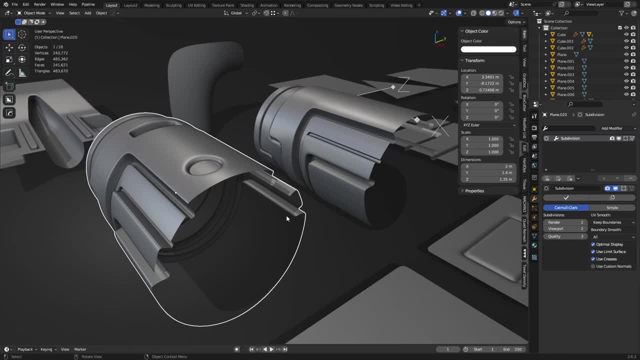 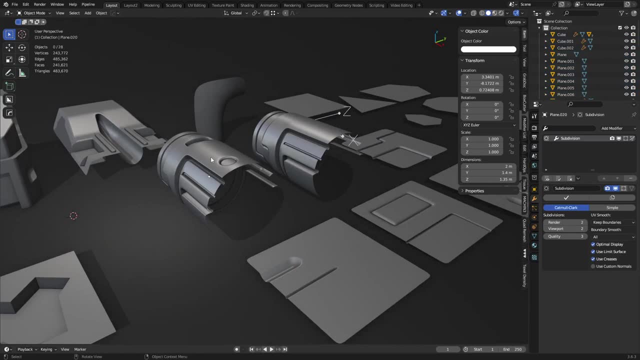 Add on: surface slide is on the modes pie. I have it shortcutted to my quick favorites, but um, it's on the modes pie. So when you're in edit mode you hit the tab key, Uh, you'll have the modes pie, and as long as you turn it on in the 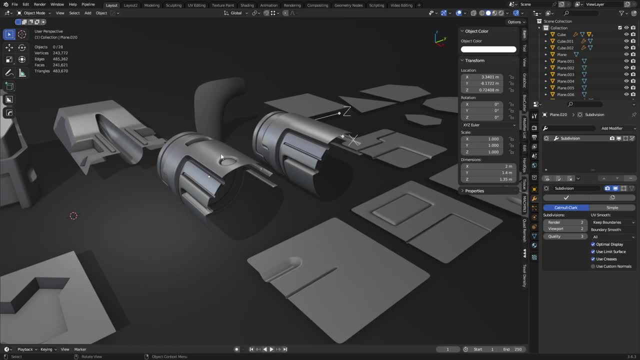 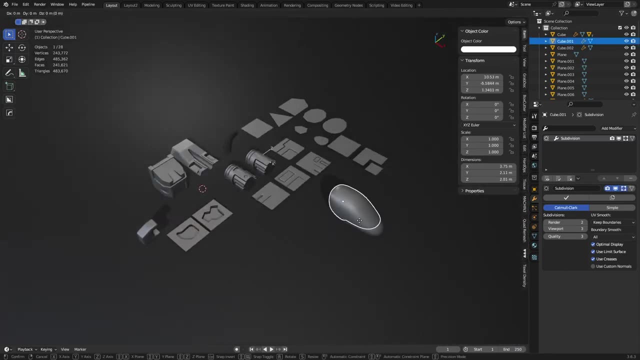 Preferences of the add-on and you'll find surface, slide on that modes, pie and edit mode. So your edit mode, hit the tab key, It'll be there, Basically what I was getting at anyway. So that's topology in a nutshell. It's really uh, you know, like I said, it's not going to be a fully exhaustive video. 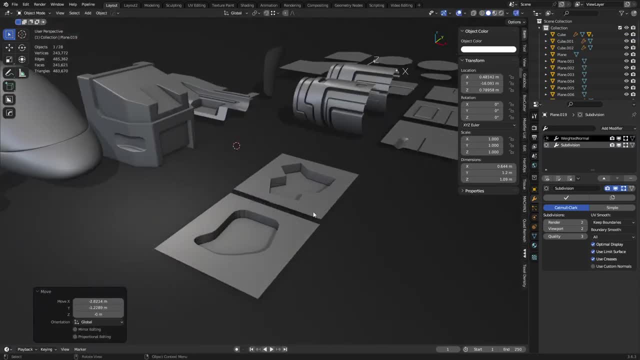 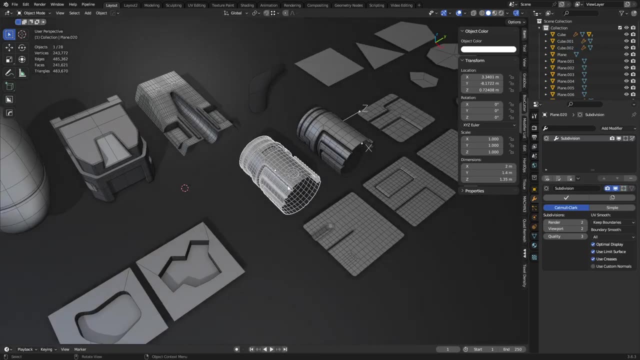 We're not going to jump into every aspect of it, but it's really the balance and the relationship of your geometry. to create a nice clean geometry, uh, is ideal. pretty nice clean subdivision models is a good way to practice that. 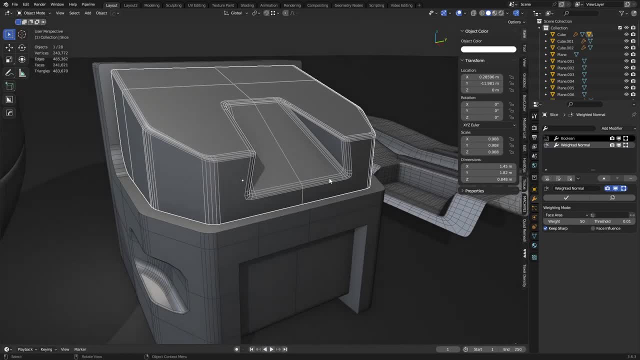 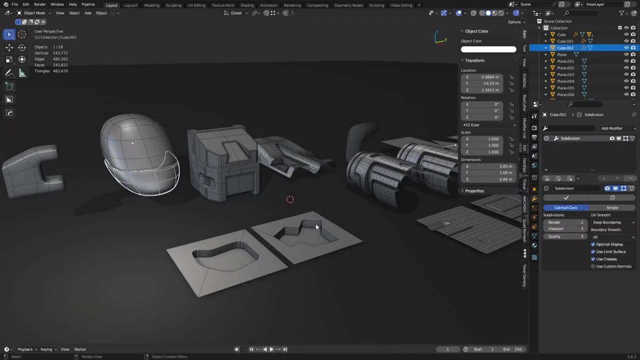 Um, but also it comes into play with Boolean and gun as well, right, And you see, this just has different rules for that topology compared to a subdivision. perhaps to some degree they're very relatable though, And so as you go through all these little practice exercises, or you take careful note. 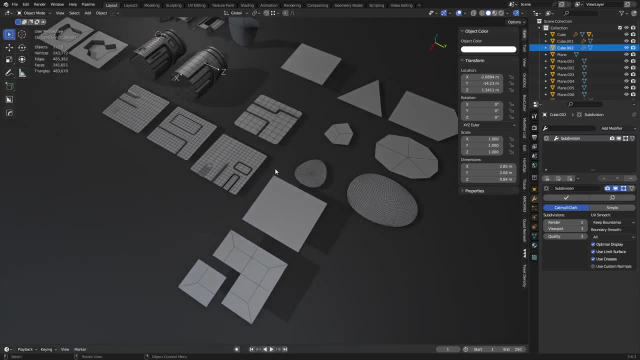 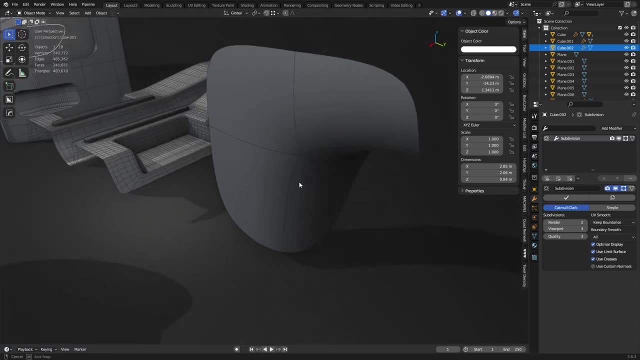 of the impulse and the equals, all that fun stuff. you know this will make more and more sense as you work with your topology and it'll actually become kind of easy to deal with after a little while. So one last thing I want to mention. 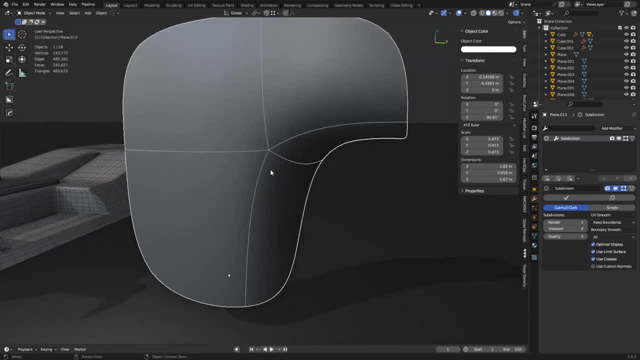 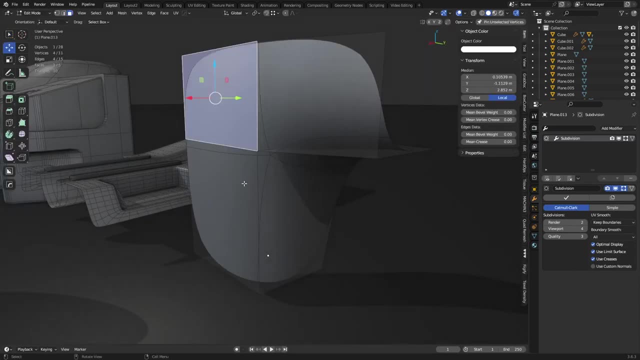 The EPO. a lot of times it's used in what's called saddles or where, like I was saying, that the geometry wants to kind of all flow together into a certain specific shape. So a lot of times this happens on like the chest of a character near the armpit. 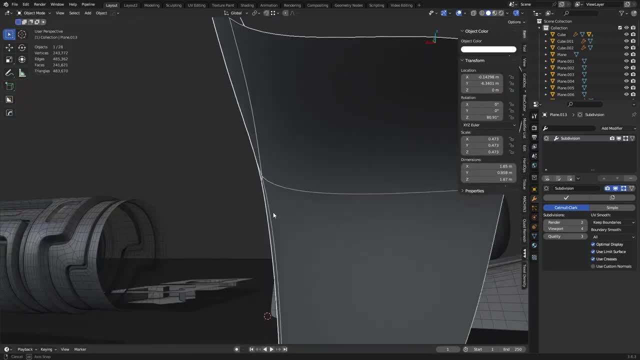 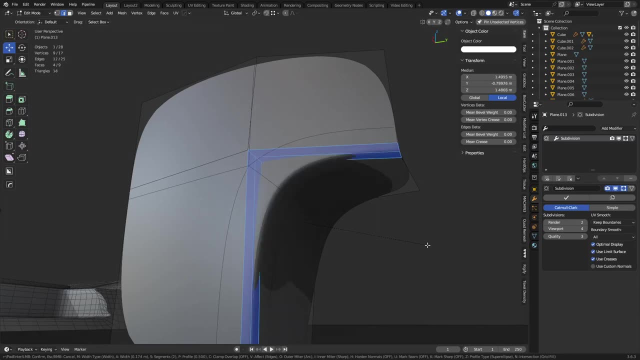 And so you can see here, the EPO here on this kind of curve also works out pretty well. But if this was a hard surface shape, on the other hand, you know you might want to do your bevel and do a number like that, right. 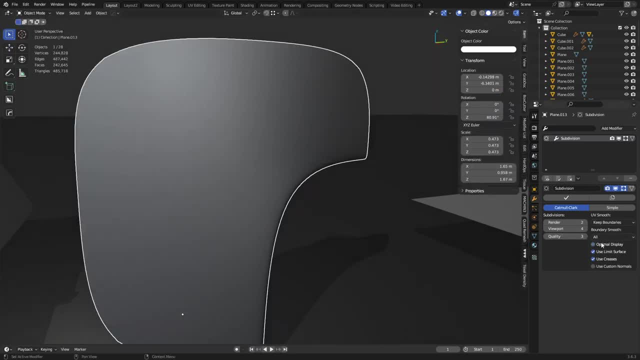 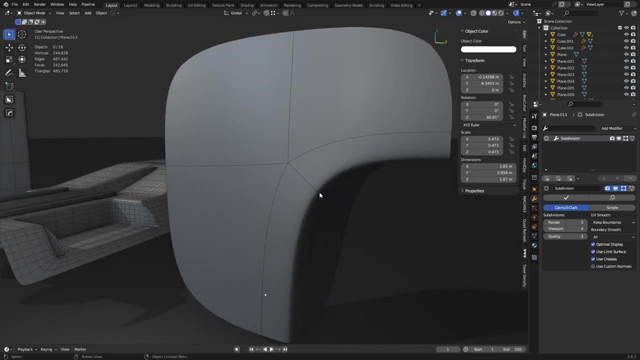 So that way it pushes that EPO a little bit further away. You can see when it subdivides now, Or the optimal display here you can see it pushes that EPO back away from that edge a little bit. So that's a good thing to recognize as well. 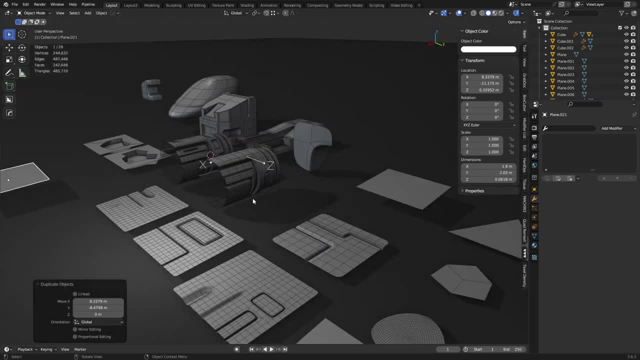 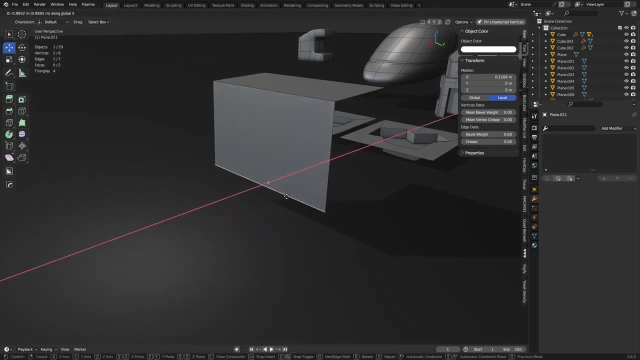 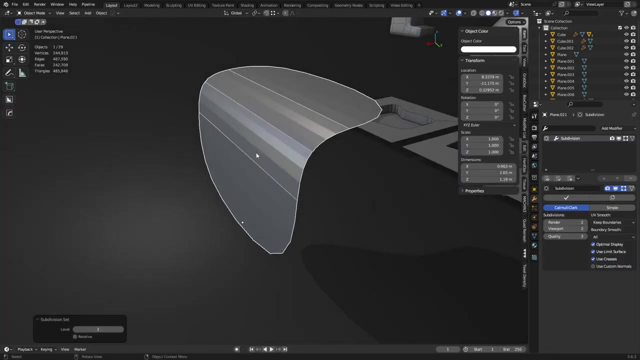 One last thing I kind of skipped over. I'm going to talk about bevel shape. So when you're working on a model- and it's a hard surface model in particular- You can do bevels like this right And subdivide them and you'll get that nice smooth curve there. 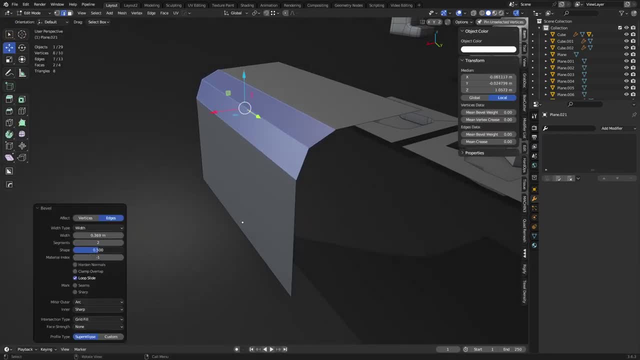 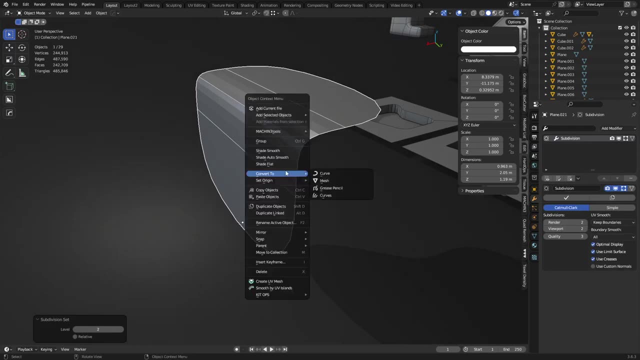 That's fine, But you can also do bevels with a shape of one. This is going to be known as a Korean bevel, And so this is going to be better if you want to keep your edges a little bit crispier, right? 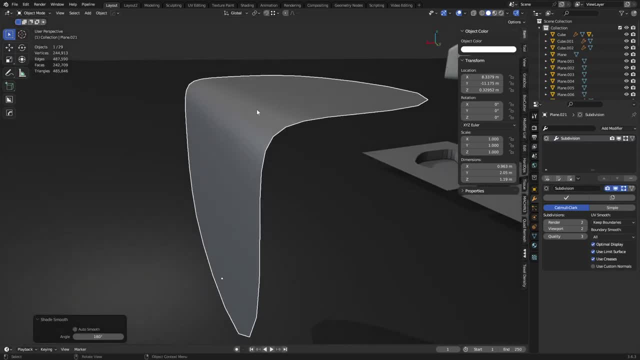 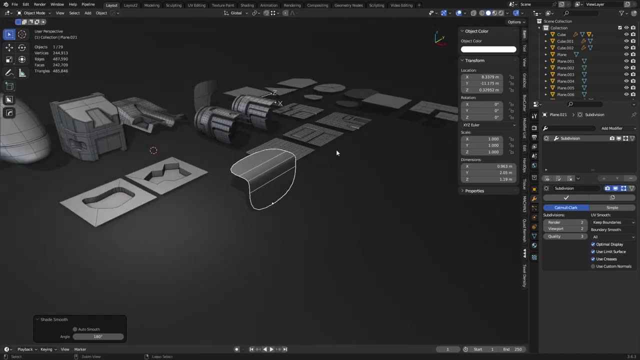 So it's just keep them a little bit tighter in a sense, And it'll look better on hard surface shapes, generally speaking. So if you want to go with that, you can in fact use it in that manner. Now, once you start understanding all this stuff and subdivision kind of becomes fun for you. 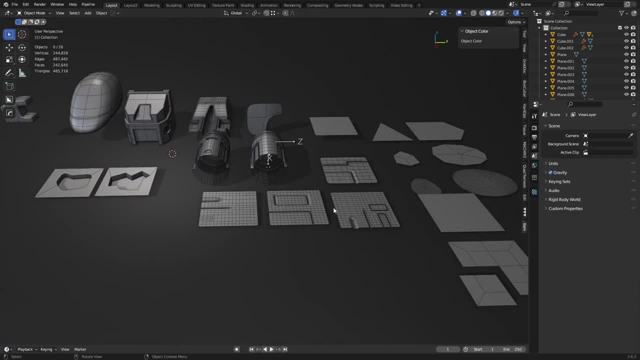 you'll realize that you can employ creases into subdivision workflow. So you know you will be using creases possibly, or the weighted bevels, And if you can get used to using weighted bevels and creases and working with the topology in this manner, 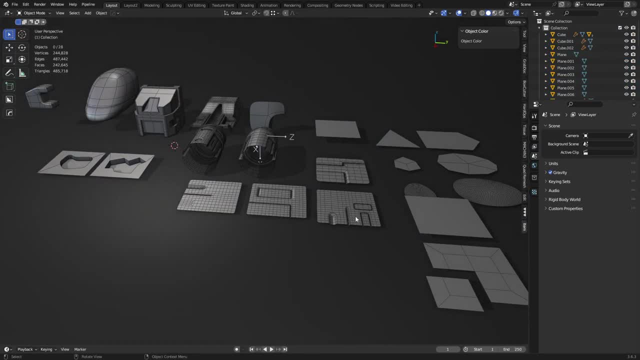 you're going to feel a lot more comfortable creating any 3D model. for the most part, The only other thing I would say is: Boolean Ngon is kind of like a different way of working that has its own peculiarities to it, So you would want to play around with that one as well. 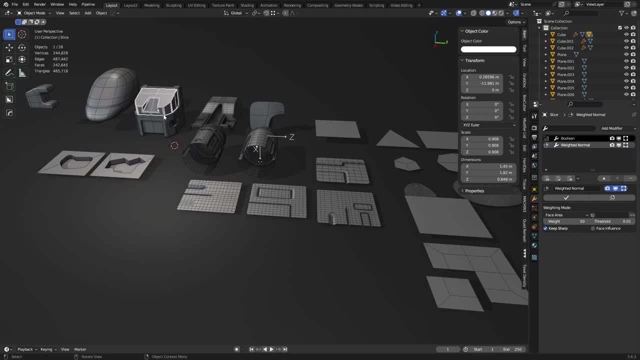 So I think subdivisions or standard modeling is really the base of everything where you're working with triangles, quads, Ngons, But subdivision is like an extension of standard modeling. Boolean Ngon workflow is kind of an extension of standard modeling. And so when you kind of play back and forth with those two ideas, 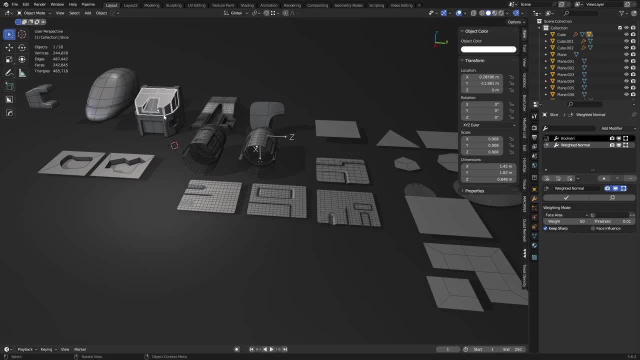 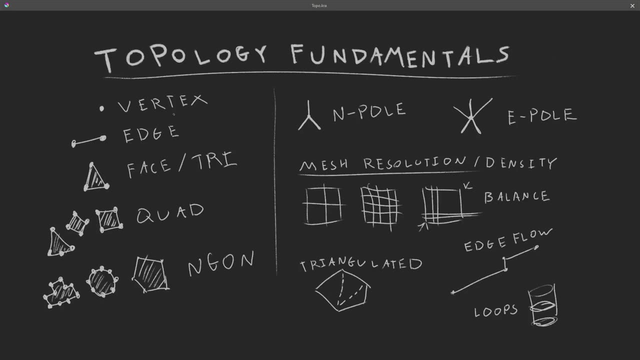 you realize that all of what I'm showing you here is more or less standard modeling. in a nutshell, You know you're using these faces- These are your kind of like your Lego blocks- to your 3D model. You notice that we're not seeing anything outside of this. 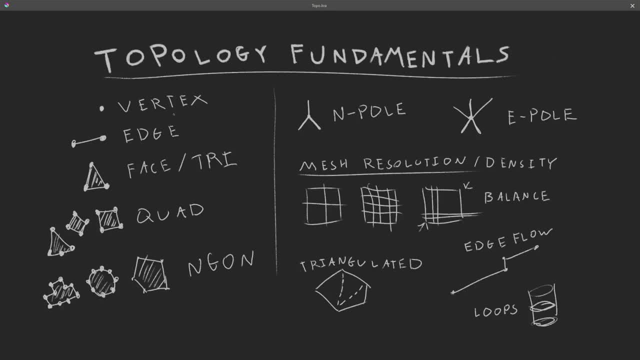 We're seeing vertices, edges, Triangles, quads, Ngons. We're not going into complex Ngons. We're trying to stay away from things that have many, many edges coming out of the EPUL. But when you keep your models as simple as possible, 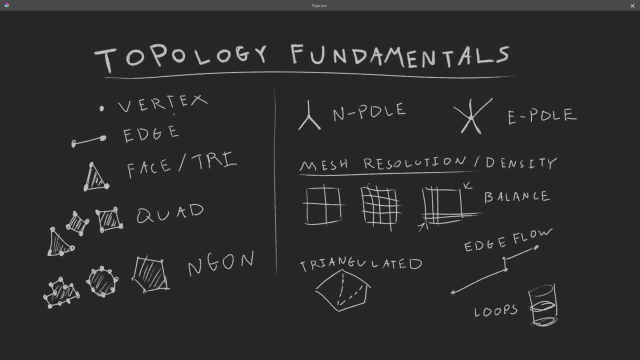 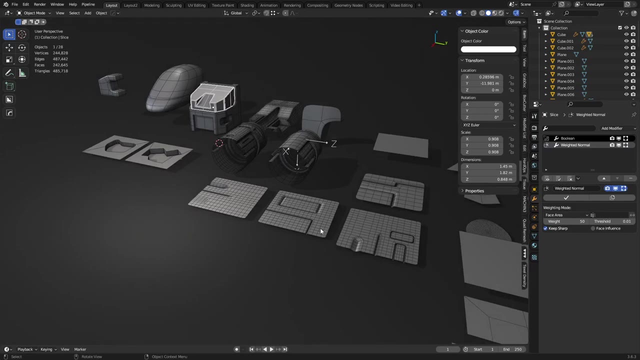 you're much more capable of managing them and working with them, And so- but these are your foundations. This is why I wanted to show you these things in particular, because with this knowledge at least, even if you know you're working on a project and there's not a tutorial on it or something like that- 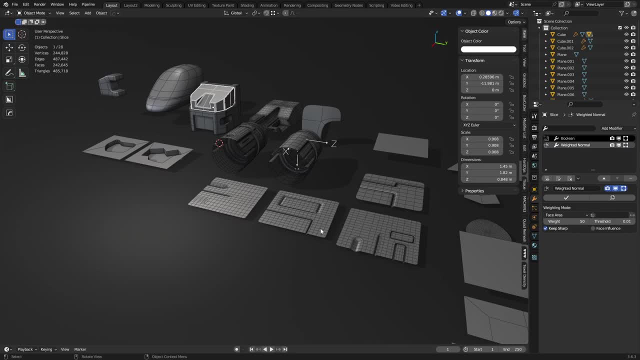 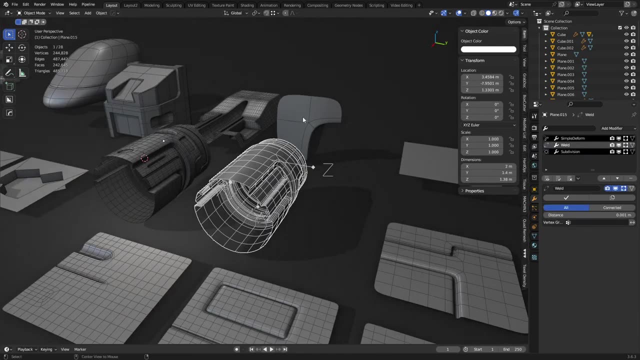 hopefully you can take this information now and you can start to look for those things and start to piece it back together on what you need to do or accomplish on that model that you're working on. And so one last thing I do want to mention, though. 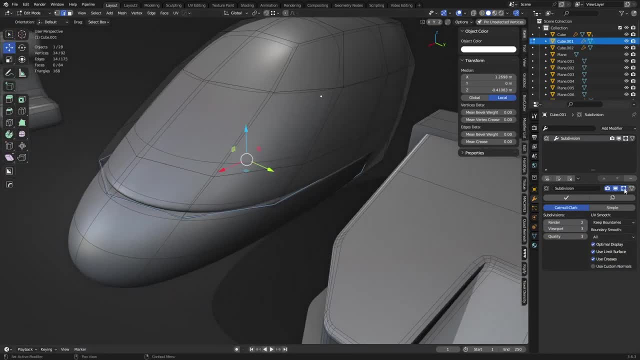 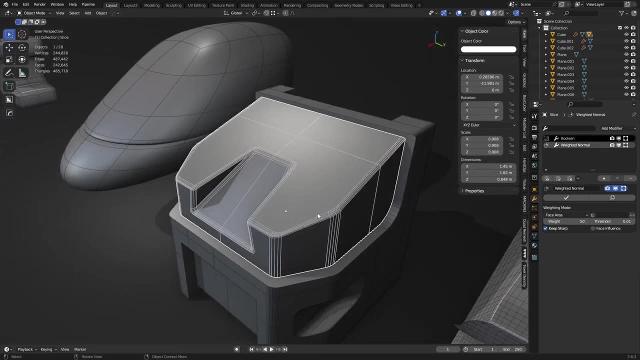 whenever you're trying to create anything, it does not start pretty. OK, it doesn't always start pretty. Sometimes you got to do these blockouts. They may even look like this, but you probably wouldn't want to do the bevels everywhere. 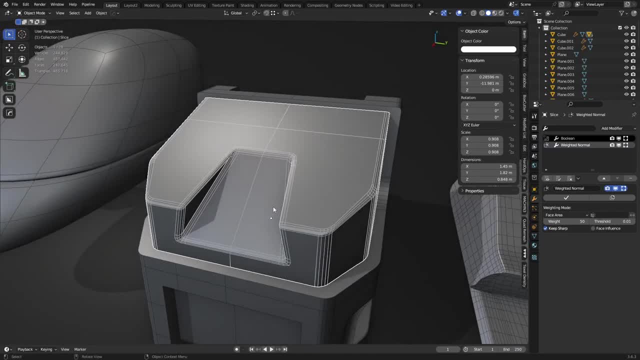 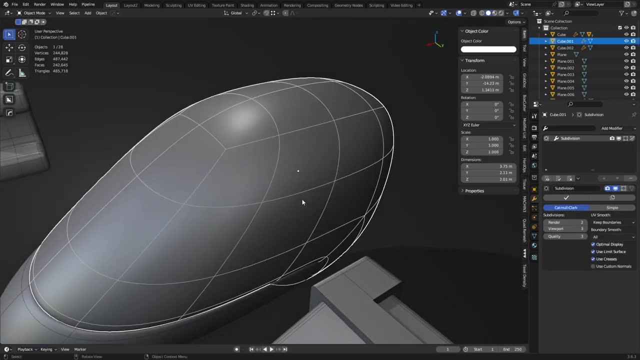 You might just want to use like the standard sharp edges, And you can Convert this to a subdivision later on much easier that way. So it might start with like bullions and a bullion and guns, and then you might have triangles and all kinds of other fun stuff going on. 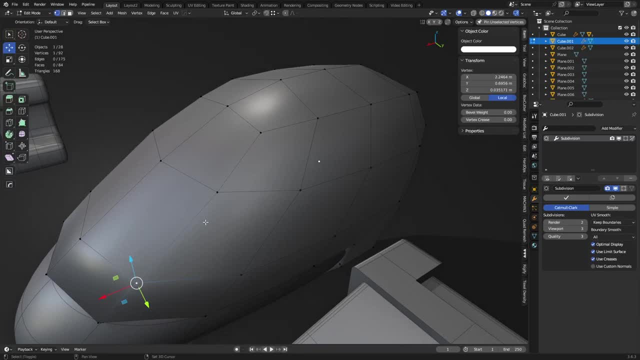 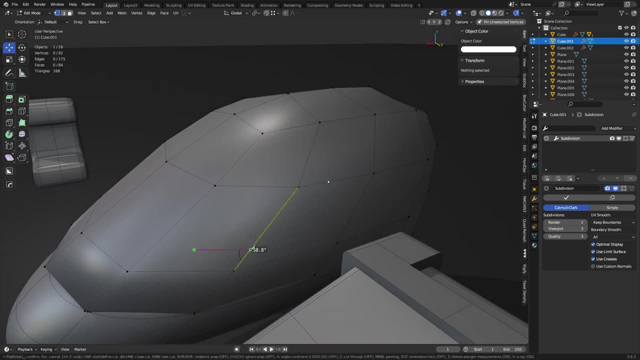 But when you're working your models, don't pay attention to what you have sometimes Like, don't focus so much on what you have. Focus on what it is you want to create. You know, if I want a shape through here and I'm in the blockout phase, I'm just going to create exactly the geometry I want, even if it's a little sloppy. 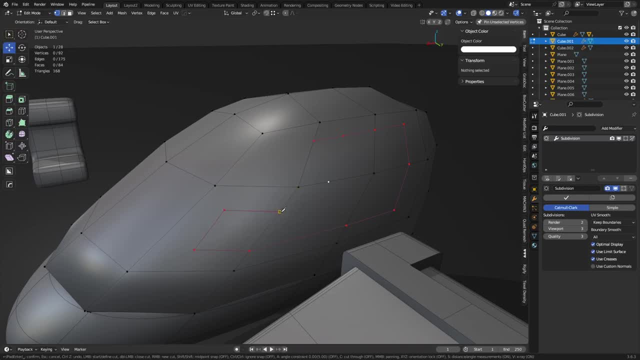 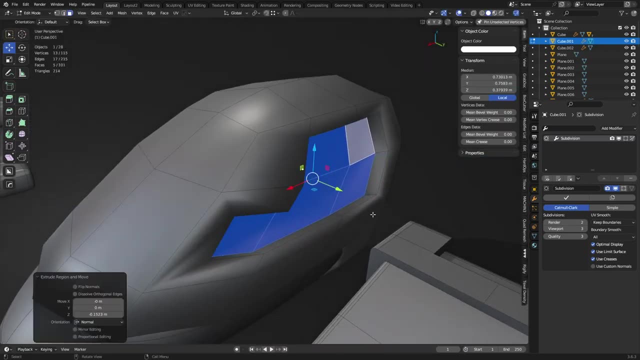 And I'm just going to make that happen. OK, OK, And then I'll figure out how to do a subdivision on it later. So if I needed this pushed in here, for whatever reason, I might push that in And you might have to rebuild the model from scratch. 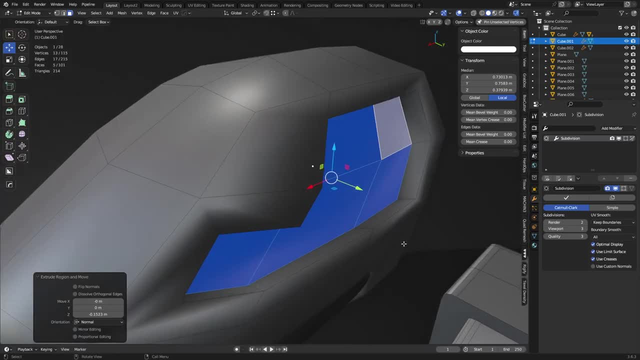 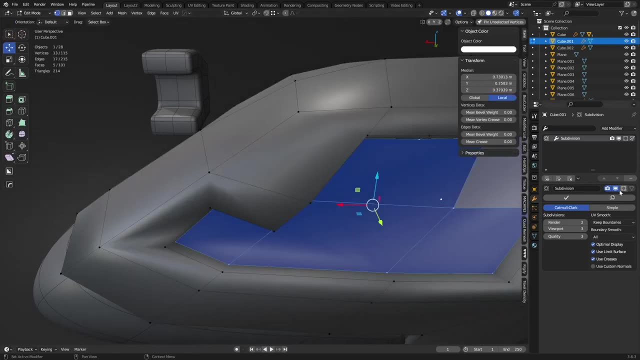 You might be able to work the one you have into the subdivision model that you need. So just keep that in mind. You might be doing this. I'm going to shade it auto smooth kind of sharpen those edges real quick, hopefully. Nope, that didn't work. 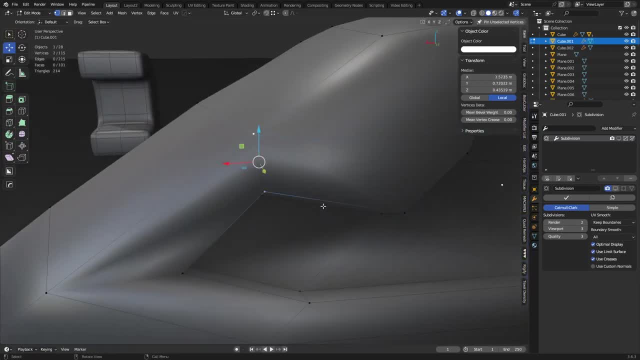 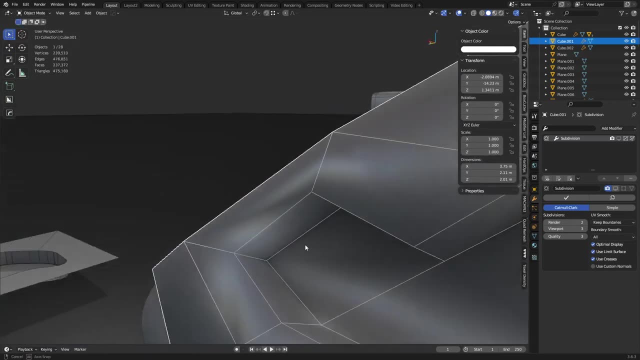 Anyways, we're going to ignore the shading for just a second, But we can start to see some areas where we can start to maybe like combine things. So if I press J through there And J through there, You might end up with something like that: 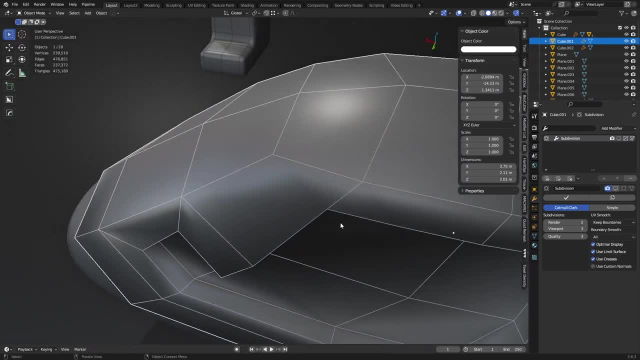 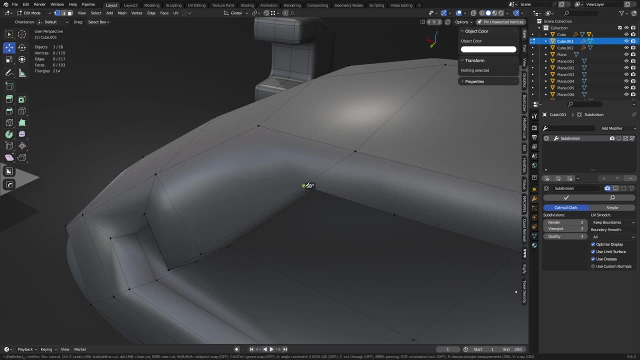 OK, And we'll see this edge here. Maybe this one needs to run around in this area. I don't know why I'm having such an issue on this one, but it wasn't cutting for some reason. All right, So maybe we need to run that one around a little bit. 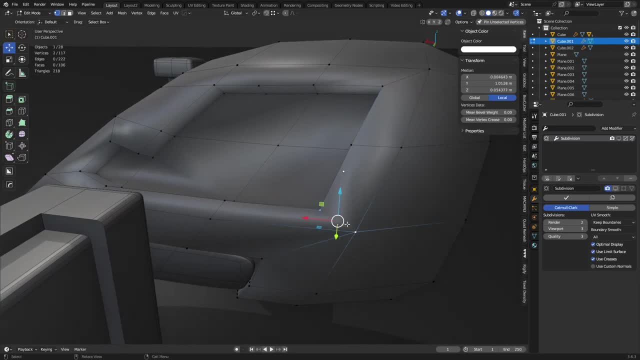 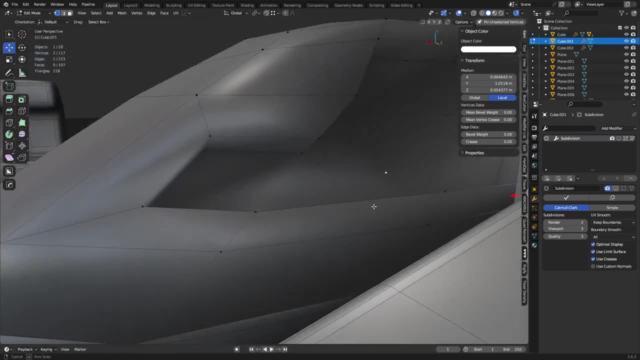 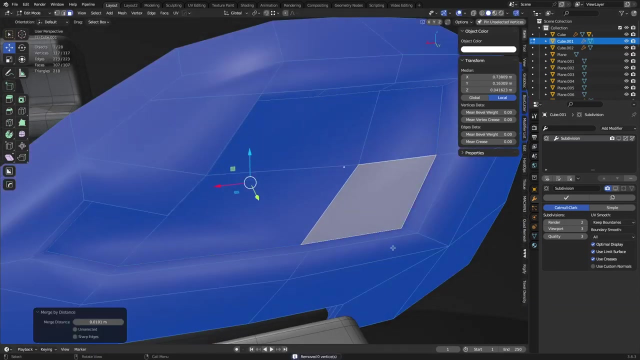 This can join here And this can join here. This is going to get harder if you start doing like weird glancing angles that go across the model, But for the most part it doesn't get much more difficult. I'm going to press A M and merge by distance. 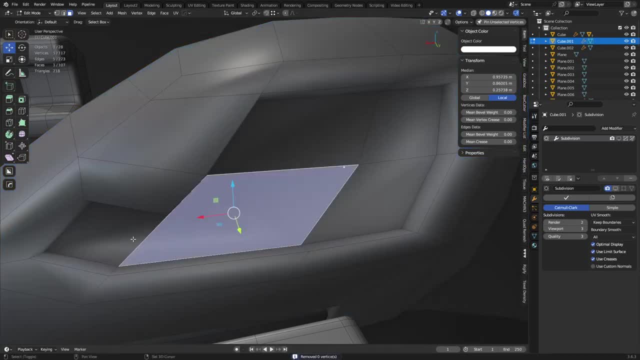 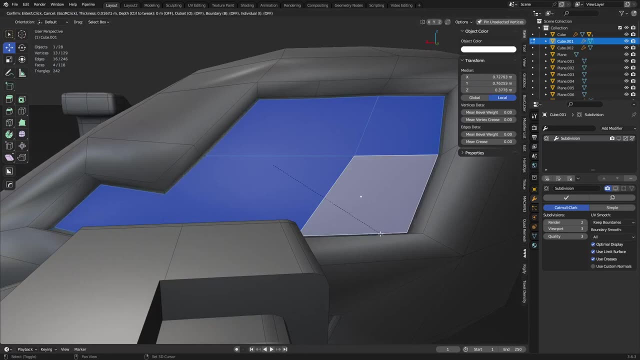 I think we've got a couple of vertices hanging out in here somewhere- Should it be able to inset. but that's not working there, So I'm going to dissolve that real quick and inset again, So you can dissolve an edge if something's not working or add an edge if needed. 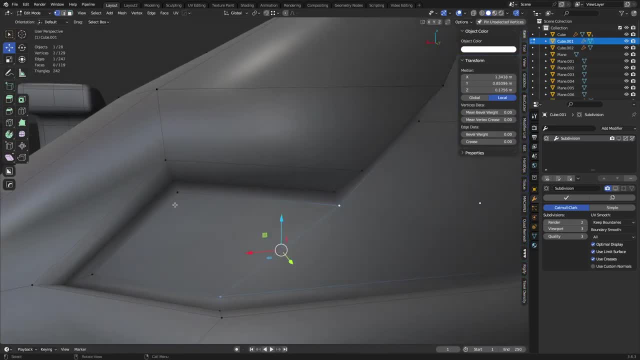 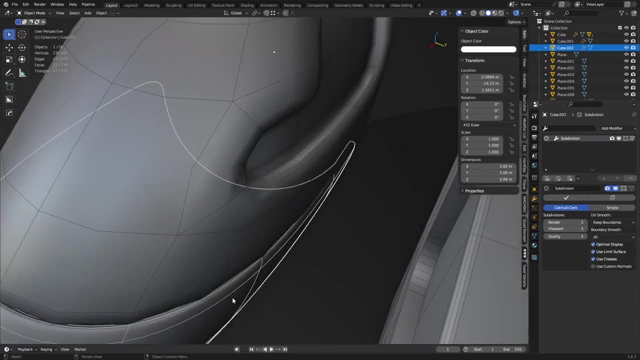 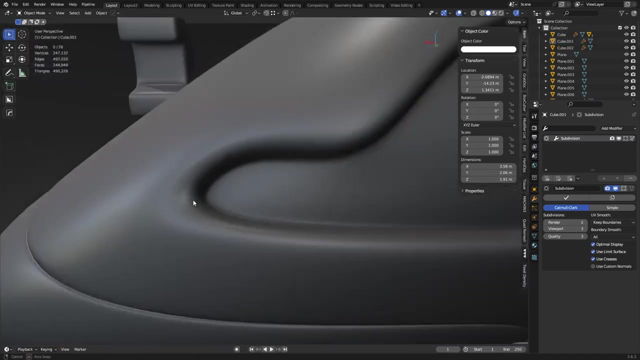 And then you can add that edge back, if that also makes sense. OK, So This subdivides. now Turn it back on. We're doing level twos, I think Level threes. OK, So if we don't mind it being soft like that, we can leave that perhaps. 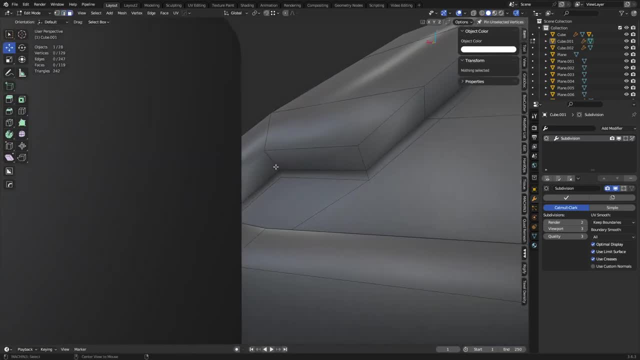 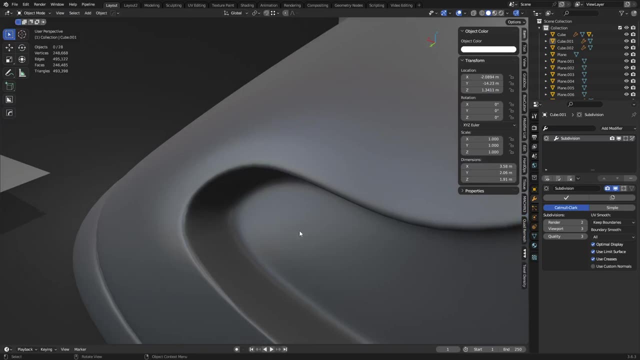 But we can always go back through the shape And try to do maybe like a bevel here, And so we're using that shape of one, So it's going to be a little bit sharper, All right. And then other times when you're really trying to hold these edges, 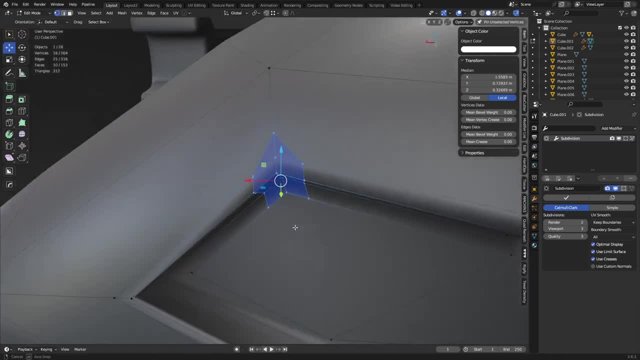 You might have to bevel them or you can use creases sometimes. But you'll see, here we're going to get kind of a very different thing going on here. We're going to have to increase the resolution to support some of this geometry. 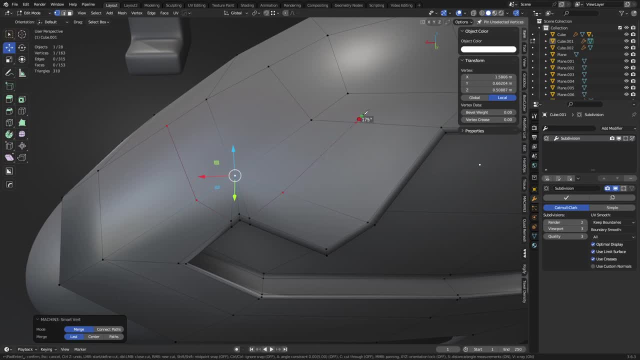 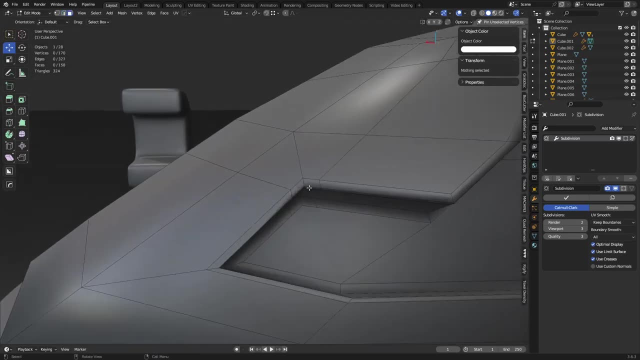 And so when you're working on curvy shapes, this can oftentimes lead to like little flat areas. OK, So you want to watch out for that. But you can see we have to work these kind of in this manner, where we go out from the edge here like this: 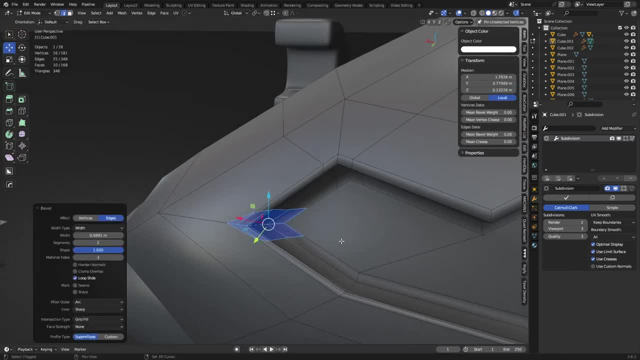 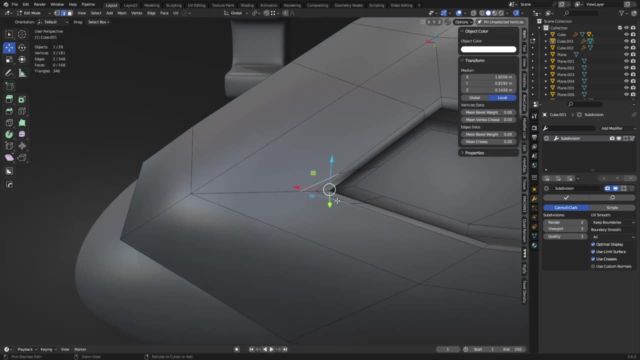 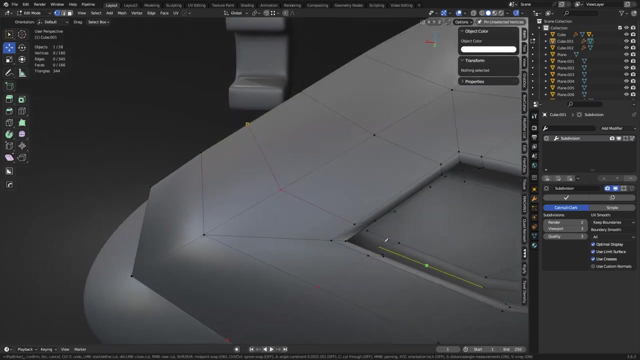 There's a lot of little tricks along the way on how you approach certain types of corners and stuff like that, Which I won't be able to cover in this video entirely. But these little tricks when you're watching other tutorials now you'll start seeing what they're doing and how they're working that mesh. 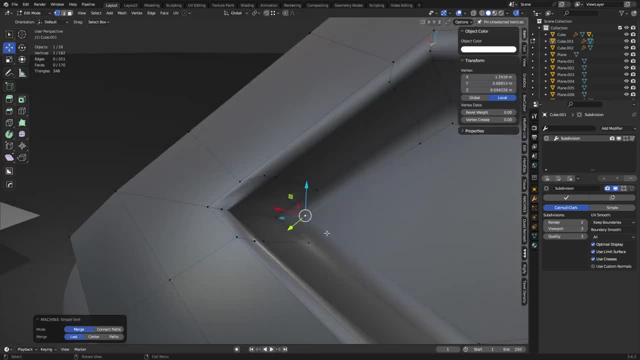 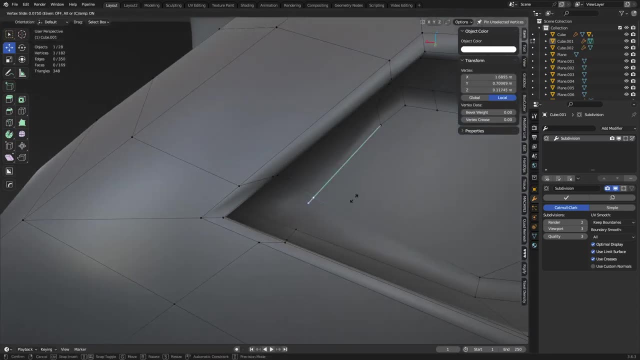 And you can see little things like this. We can merge these back to here. We can GG twice out, GG twice out. This can be a quad. So you're looking for little ways to work your mesh like this? All right, And so now we're starting to work this little front section out. 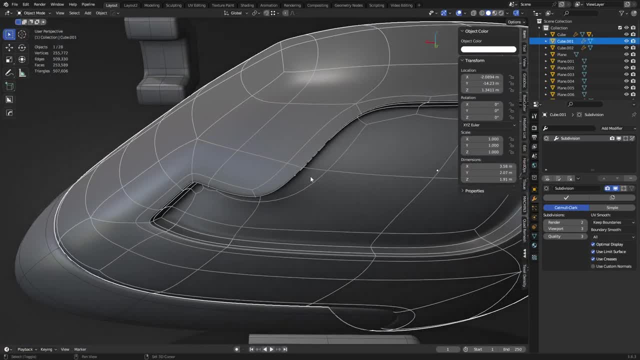 It's starting to look a lot better than it once did, And unfortunately we would have to go through and maybe do the other ones as well. Sometimes we've got things we don't actually need, Like we probably don't need that one. 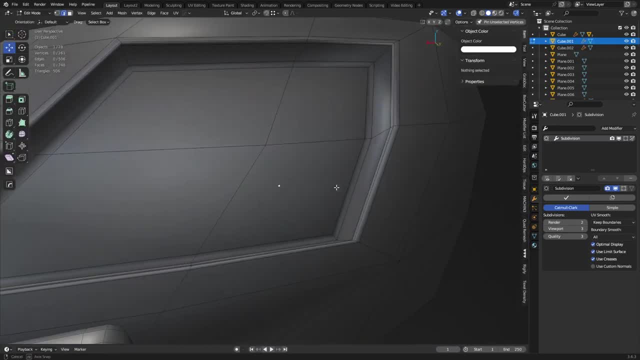 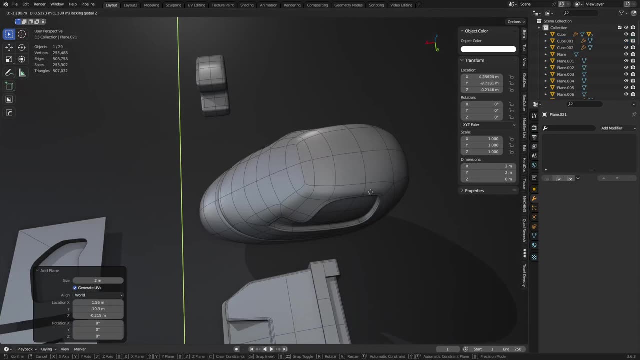 We can get rid of that. So there we go. So we can work this into quads as needed. basically, And just for the heck of it- I know we were going to end the video some time ago. Now we'll just keep going. 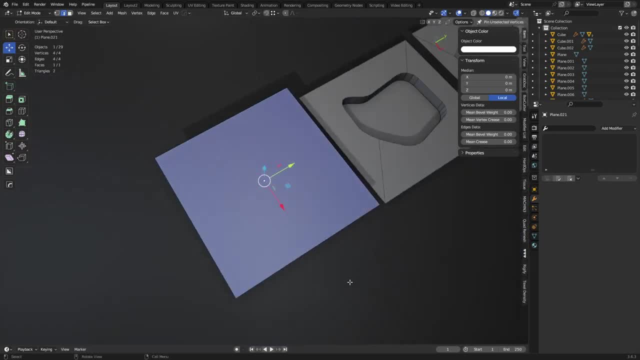 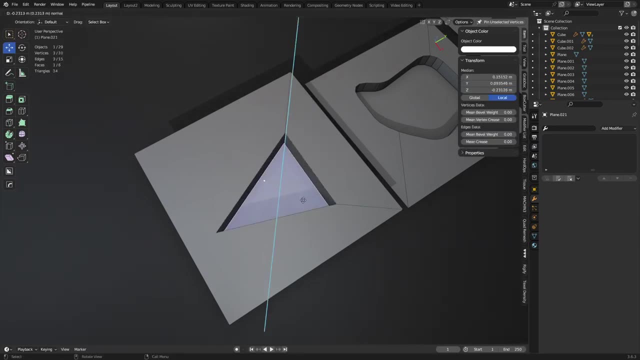 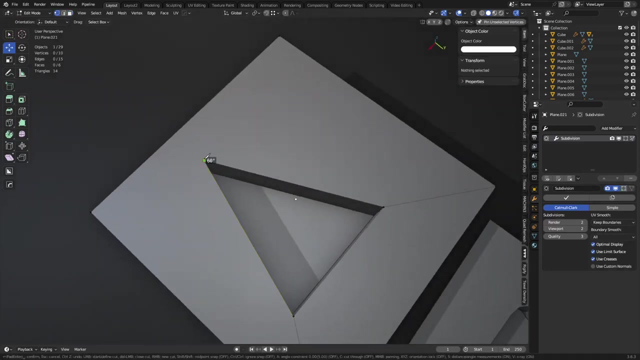 Let's just do a triangle real quick. I just want to talk about it. When you are working a mesh, You want to create a triangle, You want to subdivide, something like this. There's a couple of things that may or may not need to occur. 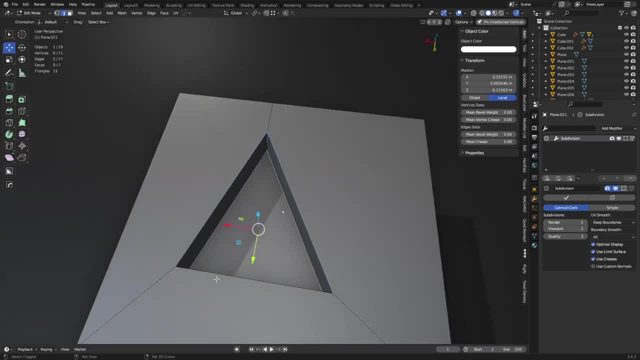 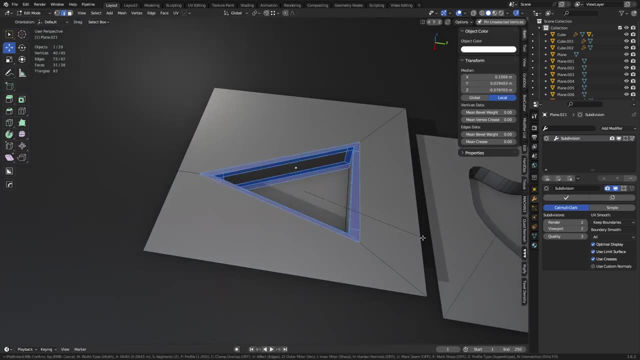 But a lot of times it's simpler than you probably thought. When it's weird to bevel this whole area real quick, You'll see kind of the topology that you need. Okay, It's not as crazy as you probably thought it was. 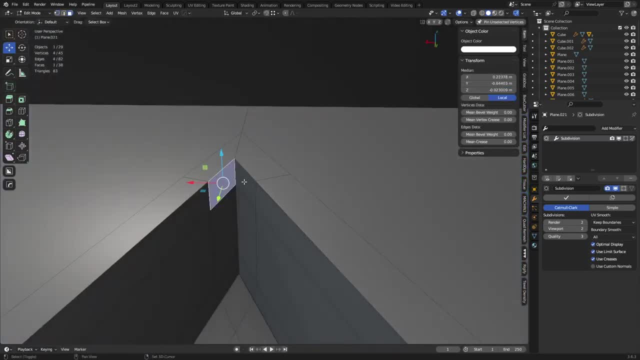 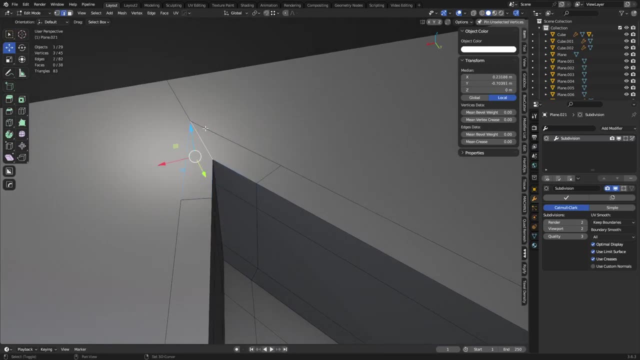 So we have, More or less We have four quads here, So Kind of see what's going on here. One, two, three and four. All right, So, And then this is: one, two, three and four. 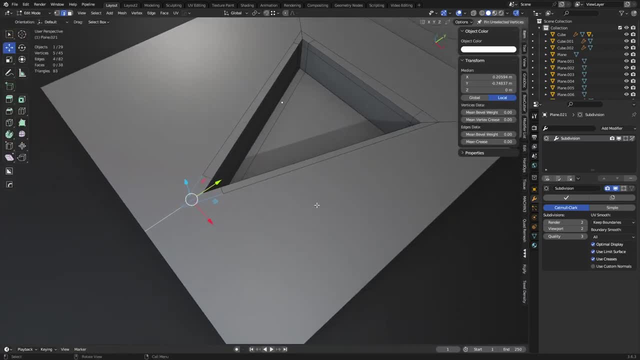 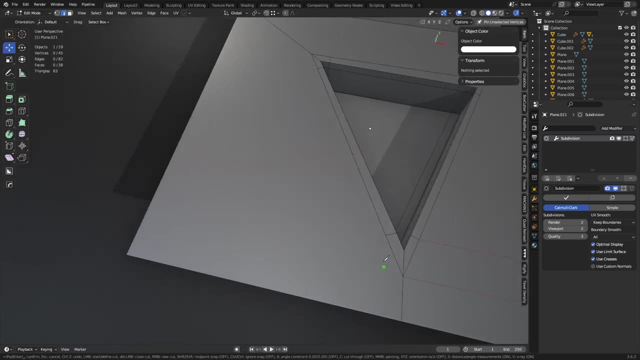 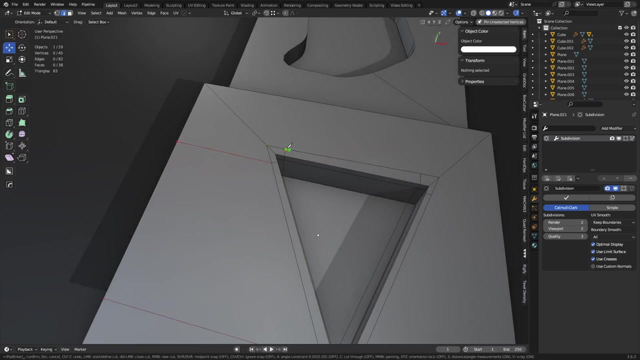 So we get this kind of subdivision going on. In a nutshell, Now, the reason it's split apart like that Is because these need their additional edges Going out as well. You have to support that topology, Okay, So don't overthink your models. 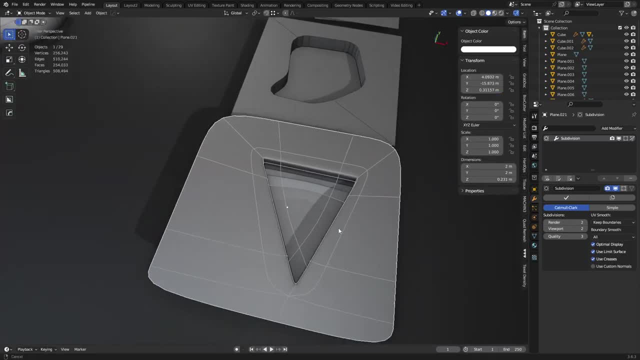 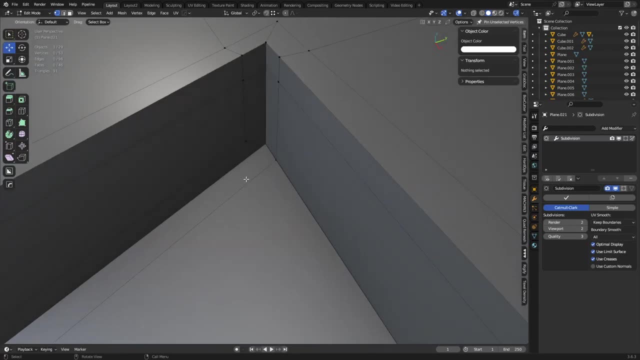 They're really a lot simpler than you probably thought they were. So it's like: oh, I added a bevel, Okay, That's great. Nothing complicated about that. This one here. I'm going to run through the shape All the way to the other side. 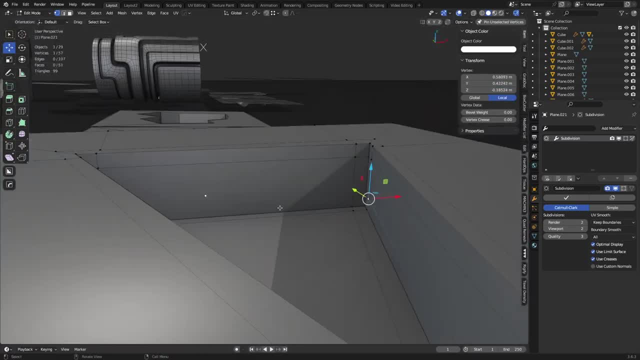 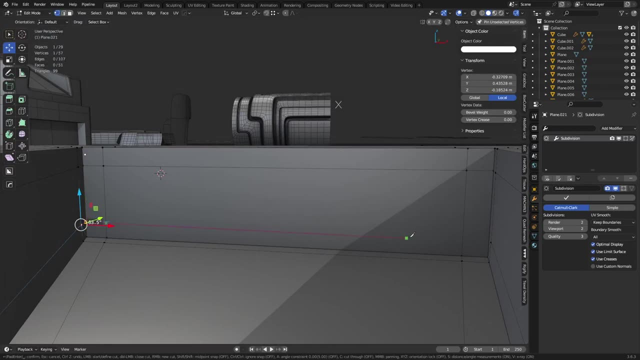 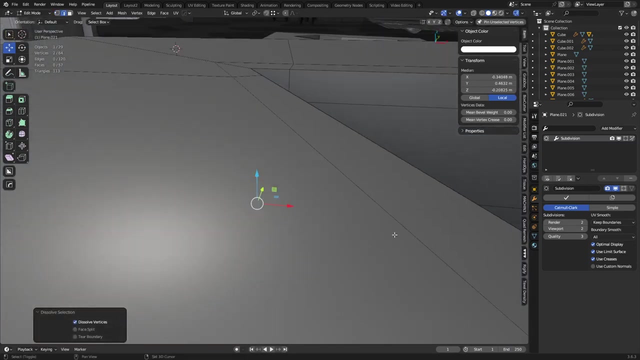 Okay, And this bottom one here, I guess I didn't select the edge or something. I don't know what I did exactly. We're going to have to run back Through here to this side, That side, And we can see. we worked that out as well. 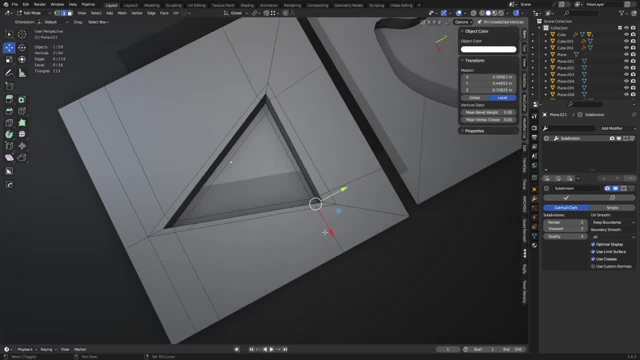 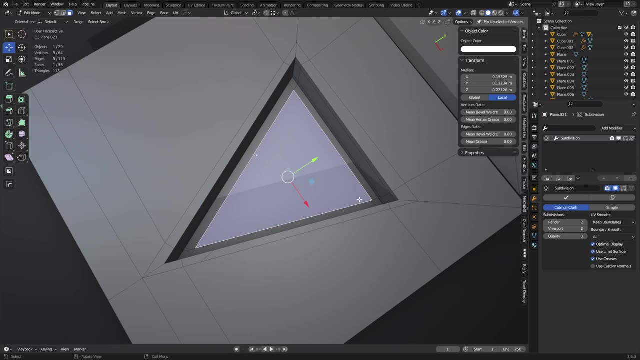 Let's say we needed more density in this middle section here, And this is what I really wanted to show you the most: How do you subdivide a triangle, right? Well, we saw how How it worked when we subdivided it with level one subdivision.